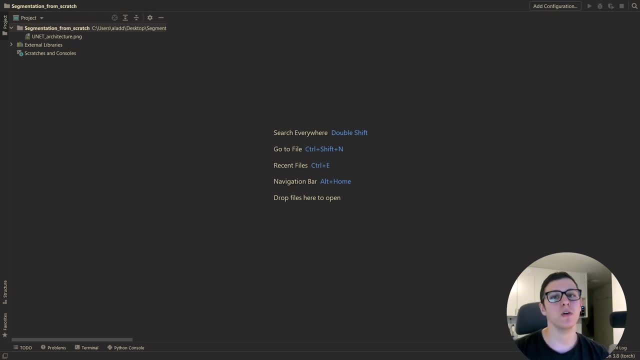 What is going on? guys? hope you're doing awesome. In this video we will go through how to do image segmentation in pytorch, And this means that we will, you know, set up everything from scratch. So we're going to build a model And that the model is going to be very similar to unit. 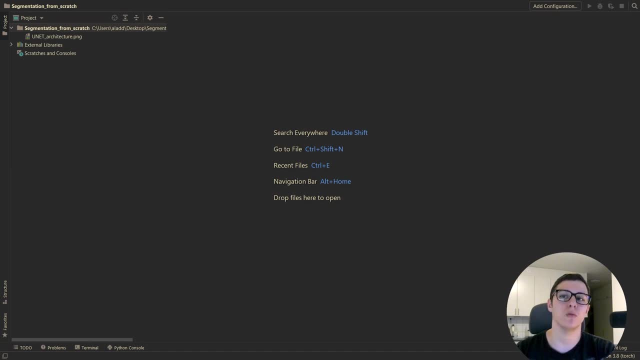 And then we're going to set up our data loading pipeline, which will include doing data augmentation for segmentation tasks, And for that we will be using the album annotations library. So if you're new to unit, if you don't know what that is, or the album annotations library, 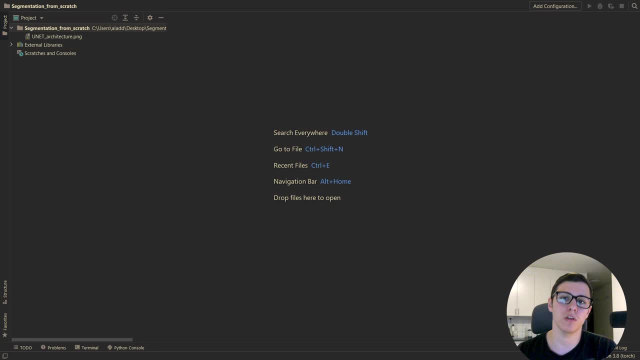 then I have separate videos for both of those which you could check out. And then, lastly, we will train this, this model on the Carvana data set, which is a Kaggle competition from a few years back. All right, let's roll that intro And then let's get started. 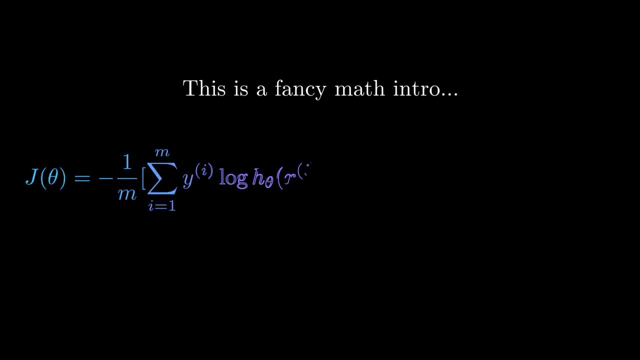 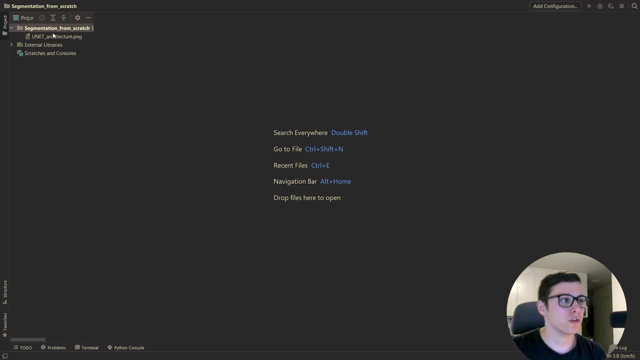 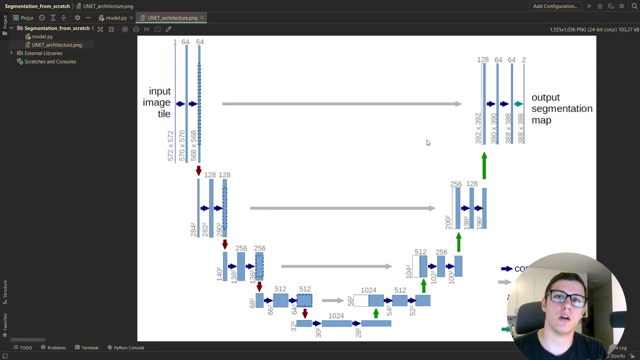 with the model. Alright, so let's just create the a model dot Python file And maybe before I start, let me just talk a little bit about the differences that are going to be in our implementation versus the paper. So here's an image that I went through on the paper review video. 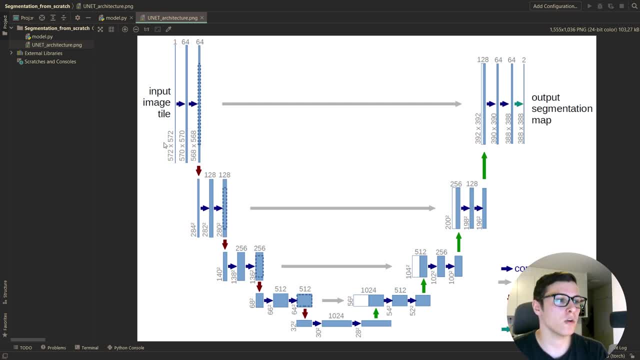 But so the difference that made major difference is going to be in the paper review video. But so the difference, the major difference, is going going to be in the paper review video. But so the difference, the major difference, is going to be that we're going to use padded convolutions because it's going to simplify a lot, Maybe not? 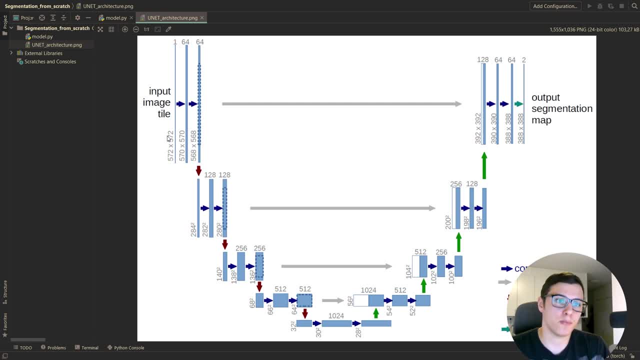 for the model, the actual model implementation. you know it's pretty trivial to just change the padding to zero and then you'll get a valid convolution. But the major difference is that when we're doing the data loading part, that's going to be much more difficult if we use this. 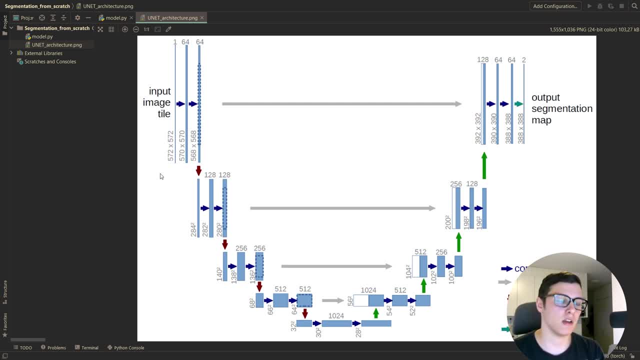 valid convolutions. So you would need to implement this, this mirroring padding, which might not be too, too challenging, But when you have larger images, you you're going to have to need, you're going to have to do sort of a multi crop of your image and then sort of stitch that up in some way. 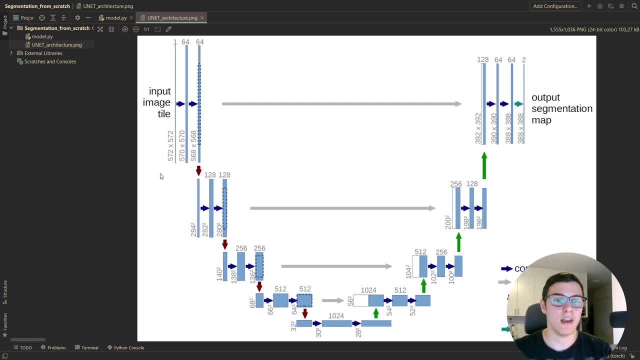 afterwards just makes things a lot more complicated. And when you think about the fact that the winners, for example, for the Carvana Kaggle competition, they use the same same convolutions in their implementation, And I think the prize was $30,000 or something like that. 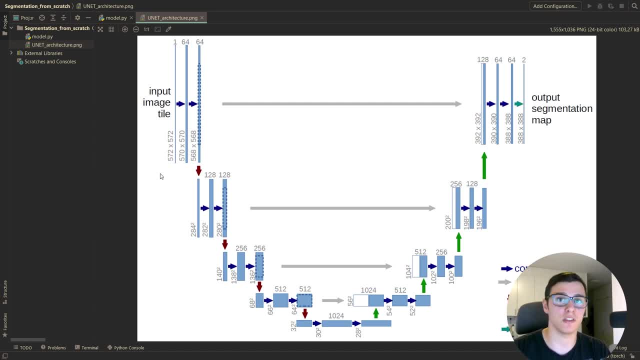 You can only imagine that if their accuracy would have improved using valid convolutions, then that's exactly what they would have done. So you know we're not losing too much performance here. Alright, that's enough rambling about the architecture, let's just get started. 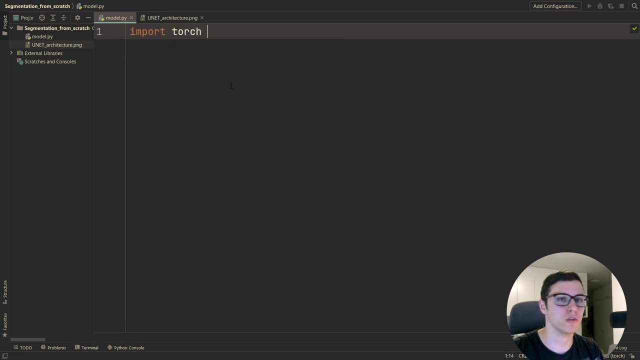 So what we're going to do is we're just going to start with import torch, import torch, that nn as an N, And we're also going to use import torch vision, dot transforms dot functional as tn. All right. so looking at the architecture right here, you can see that the first thing that they 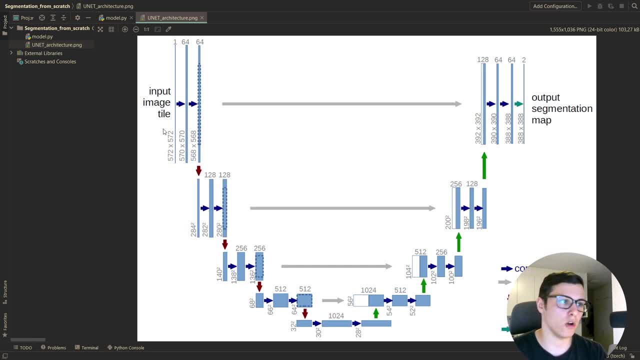 do is that they are actually what they do in sort of all of these steps is that they use two convolutions in between, So they have some input. they run it through two, three by three comms And then they do similar right here, similar right here, similar right here and similar on. 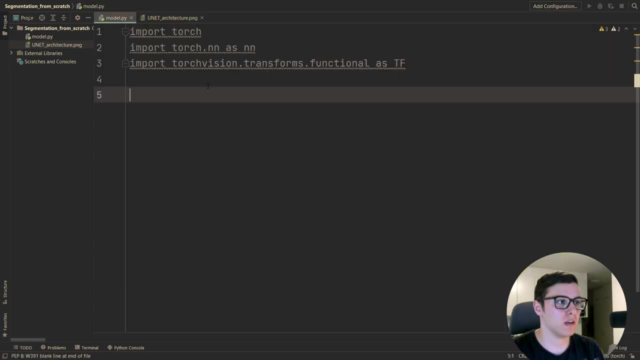 the opposite side. So one idea is that we can create a class which we'll call double convolution. We'll inherit from nn module, we'll create our init function That's going to take in some in channels and some out channels, And we'll just call super. first of all, double conv, self dot init. All right, so all we'll do. 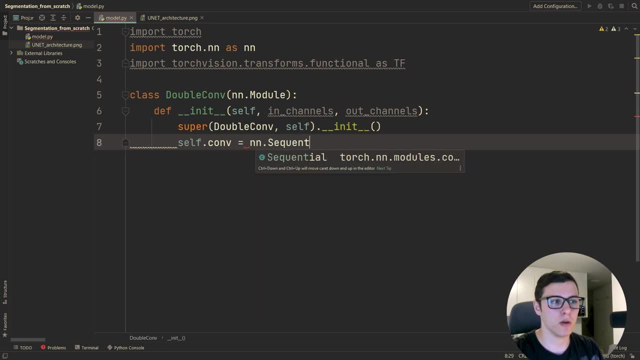 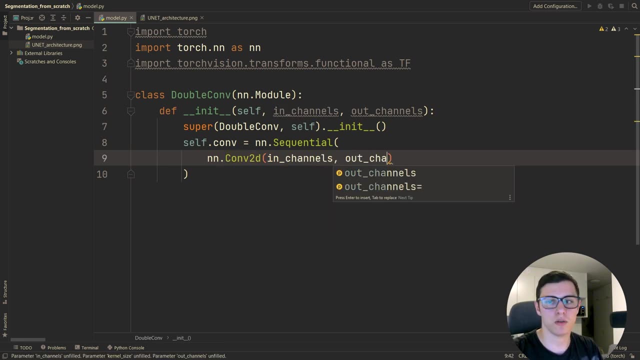 here is just selfcom- equals a sequential model which will use a comm 2d with some in channels. we'll set the kernel size to three, the stride to one and we'll set the padding to one, which will make it a same convolution. So you know- I'm assuming you know- what same convolution. 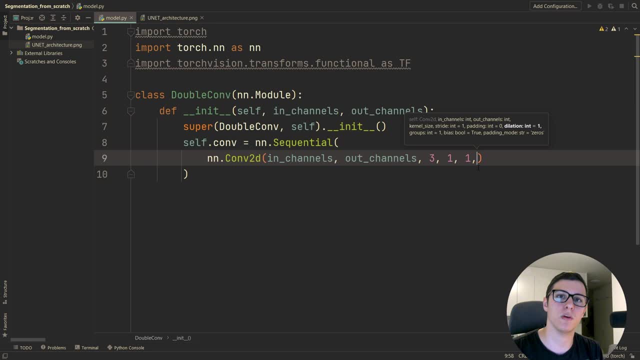 is, But that means just that the, the input height and width- is going to be the same after the convolution. I'm going to set bias equals false here also, And the reason for that is because I'm going to going to use batch norm, And so in the original paper I'm going to say that the value of the 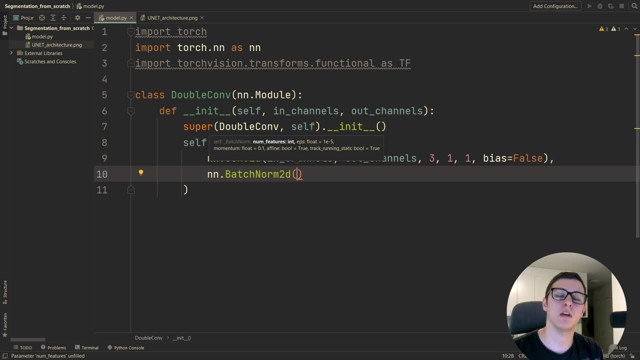 think the paper was from 2015.. And I think batch norm, the batch norm paper- came in 2016.. So of course they didn't use batch norm, But I figured that there's. I mean, it would only be beneficial, So let's use it. And so we're using by bias equals false. 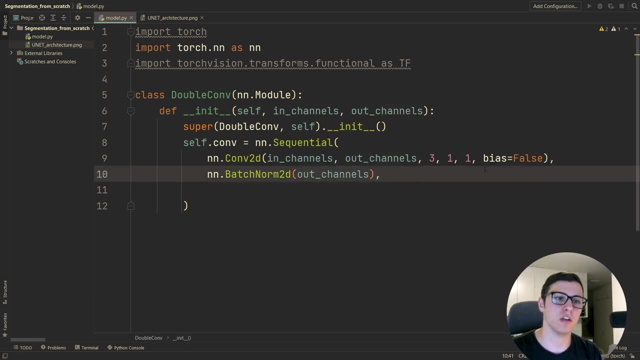 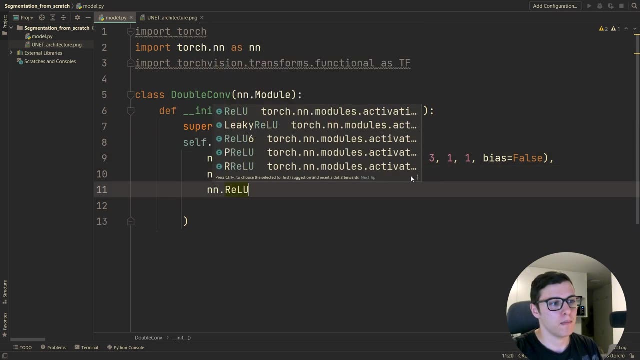 just because we're using a batch norm. So it's just an unnecessary parameter to have a bias because it's going to be cancelled by the batch norm. That's just the detail. But yeah, then we'll use a relu, we'll set in place to true And we'll just copy paste this. 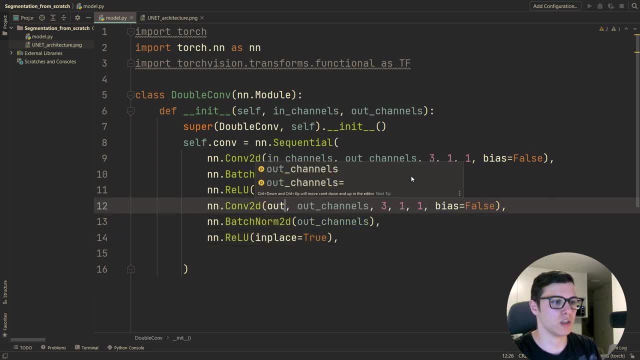 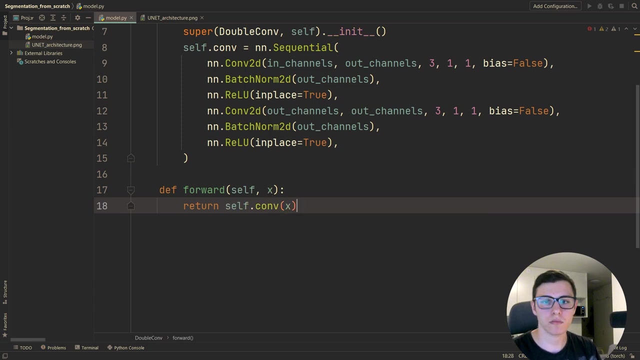 right here And do our channels to our channels for the second column, And that is it. So we'll just do forward. Forward is going to take some input x, And we'll just return selfcom of x. Alright, so what did we do? Well, we created this step. they're going to be sort of intermediate. 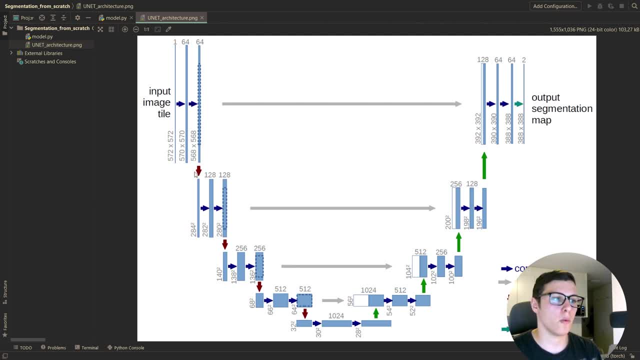 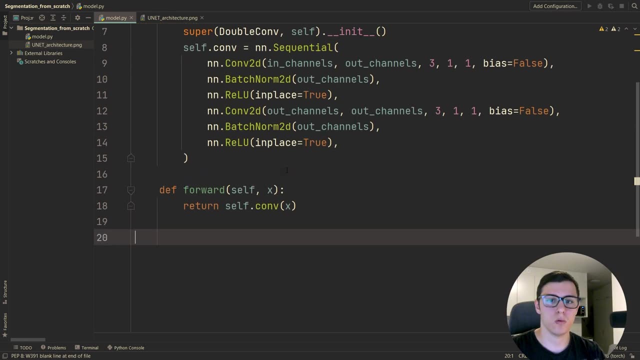 intermediate between these, And so what we want to do here is just a self pool, right, we just want the max pool stride to kernel size two And then again use these, these double comms in between. So we'll just create our class class unit. 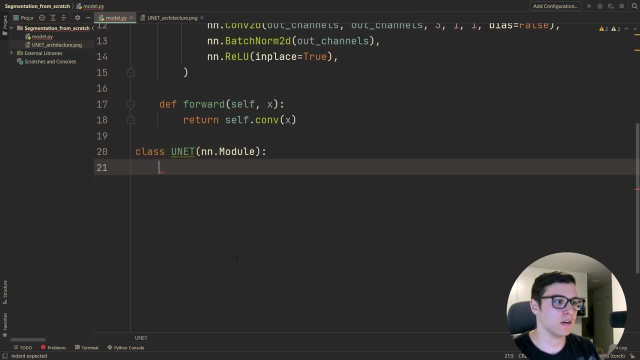 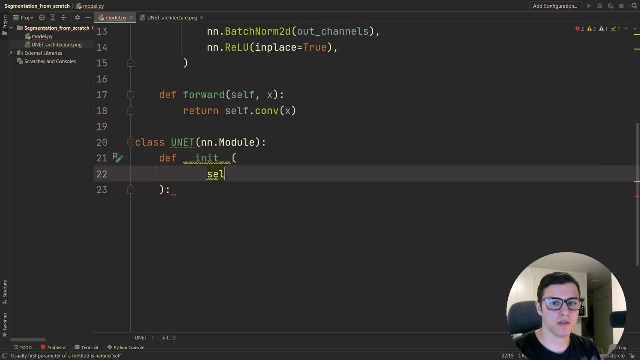 we'll inherit from nn module. Again, create our init function And see. so we're going to have self. we're going to specify some in channels. In our case, our in channels is going to be three, So let's just set default three. the out channels is going to be 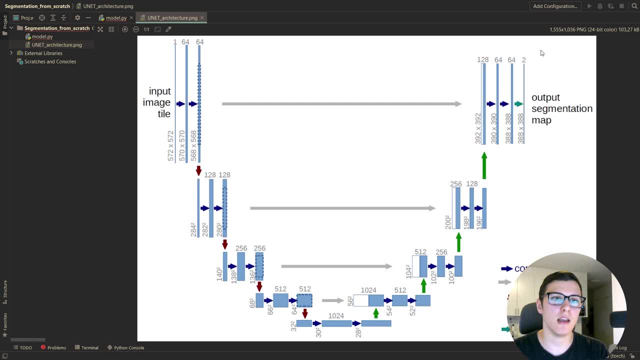 one. So in the paper they had our channels to two, And well, I guess I mean, this is a parameter you can choose, But we're going to do sort of binary image segmentation. Of course we're going to, you're going to be able to extend this to several, But the difference here is that if we're 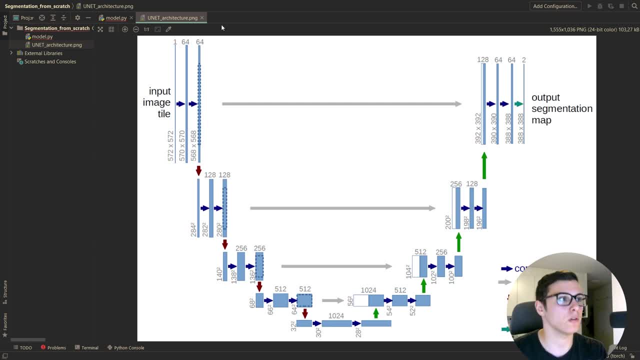 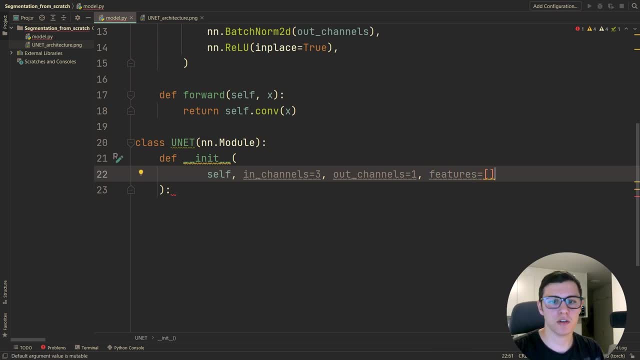 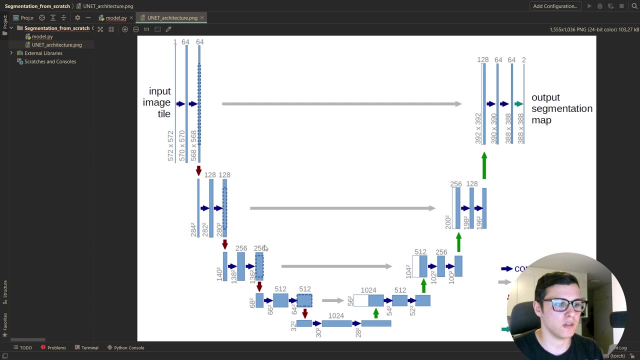 doing binary, we can just output a single channel. So let's just set output channels to one as default And we're going to specify some features, And these features right here is going to be sort of the features right here, So 64, 128, 256, 512.. And then they're going to be exactly the same. 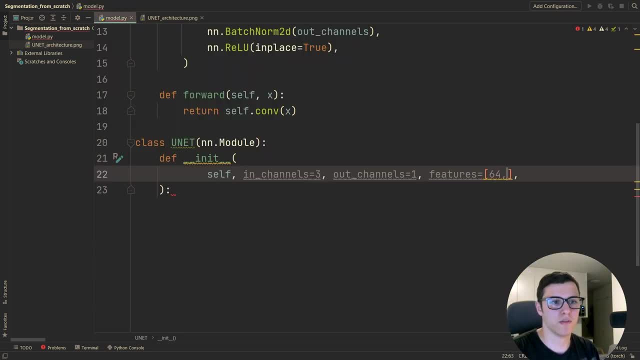 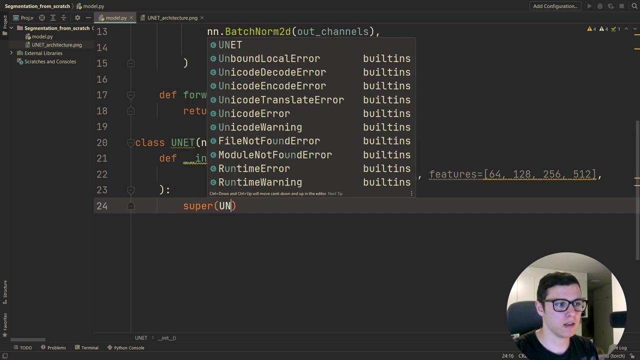 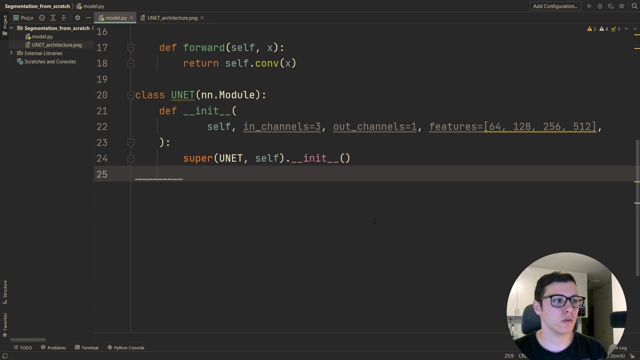 on the upward. So we'll just set 64, 128, 256 and 512.. Like that, Alright. so then what we'll do next is call super- Can't forget that part, So super in it, Alright. and then what we're going to create is: we'll create two lists, So we'll call them. 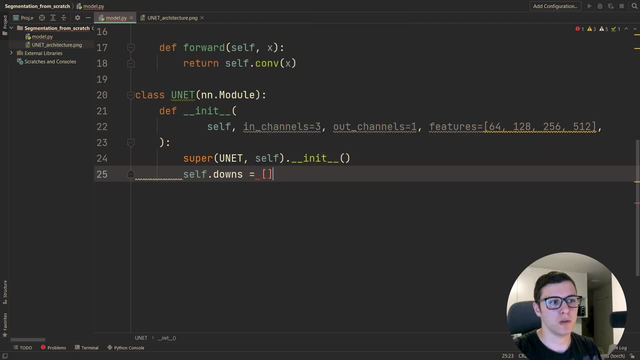 self dot downs And we'll create a list. But you can't just use a list like this, because we're going to be storing the sort of the convolutional layers and all that stuff, And then what we got to do is use a module list. And I guess why this is important is because 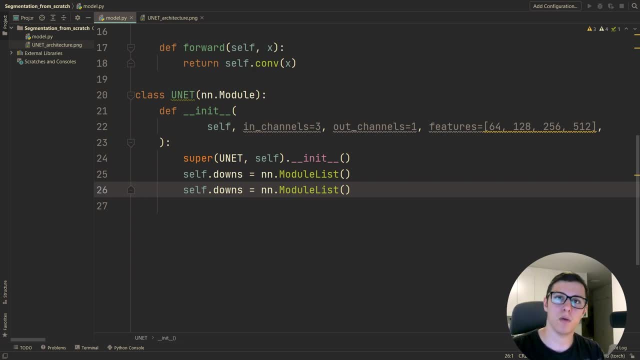 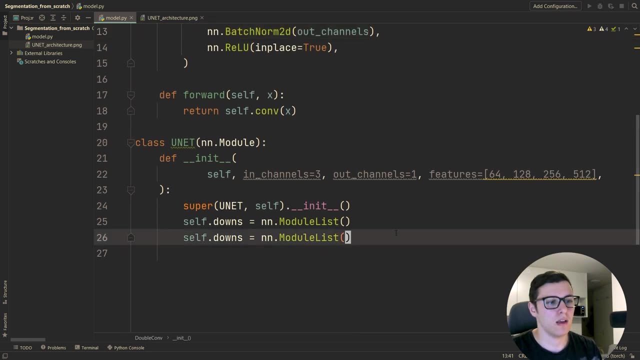 we want to be able to do. what is it called like model, that eval and stuff like that, And then we serve for the bash from layers and so on, And that's why it's important to have this module list. So we'll just have one for ups and we'll have one for downs And then we'll have a 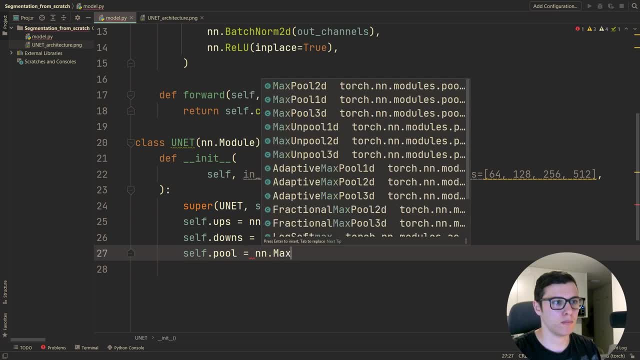 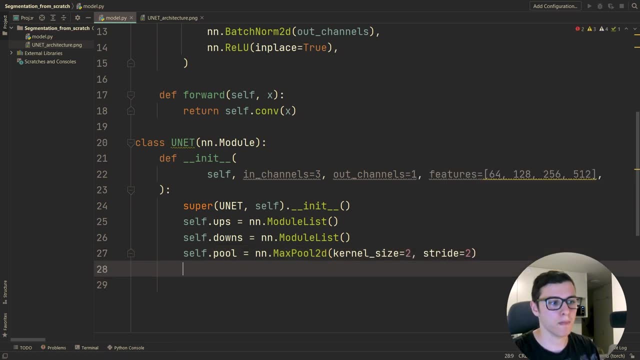 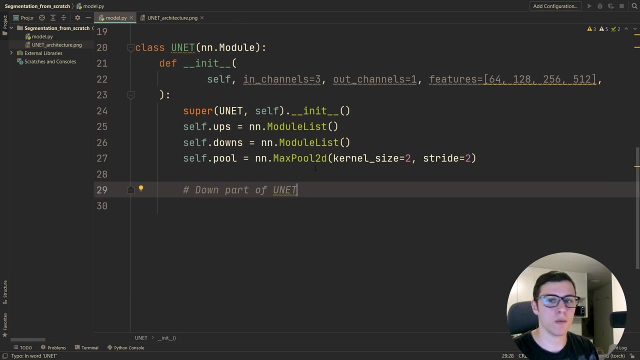 pooling layer. So let's just do max pooling to the. the kernel size will be to, stride will be, stride will be two, And so let's just do the down part of unit first. So for the down part, what we'll do is we'll go through the features, So for feature in features, And we'll do first stuff that. 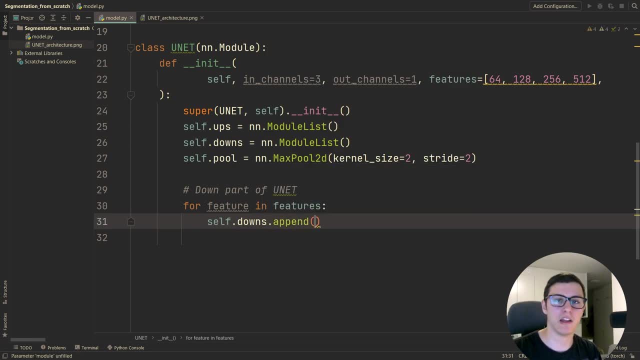 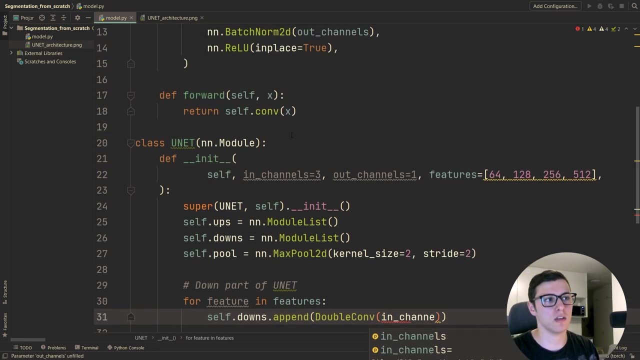 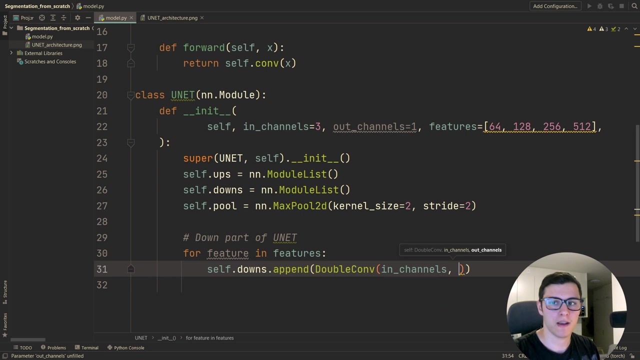 downs dot append. So we'll add a layer to this module list. it's going to be a double com And it's going to be in channels. right, because this double comma that we just created take some in channels and some out channels, So we'll just send in in channels as initial. 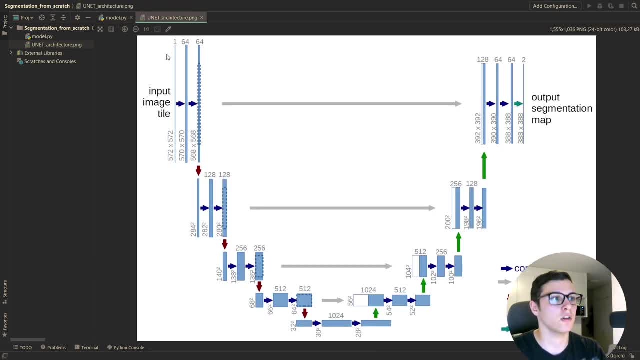 and then feature right because it's going to be. if we look at the architecture, it's just going to map some some input right, in this case one that they had to 64. And that's exactly what we have right. So in the beginning, or in the beginning, we have three here, but it's 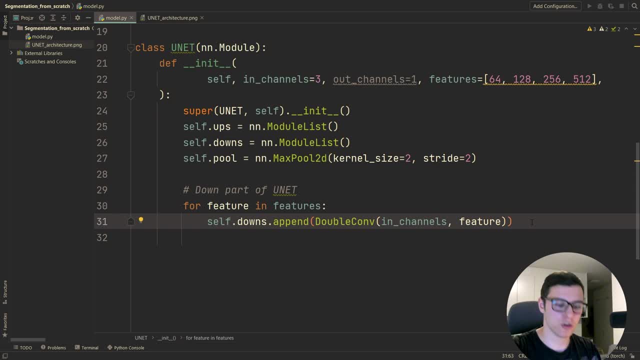 going to map three to 64.. For the next feature, we need to make sure that we set in channels to feature Right. so this is going to go through the loop depending on all that we have in those features, And it's gonna do. 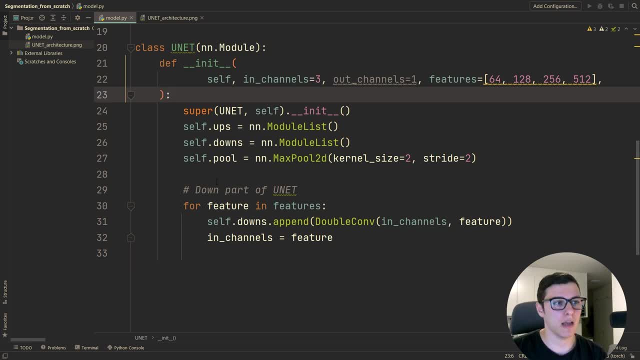 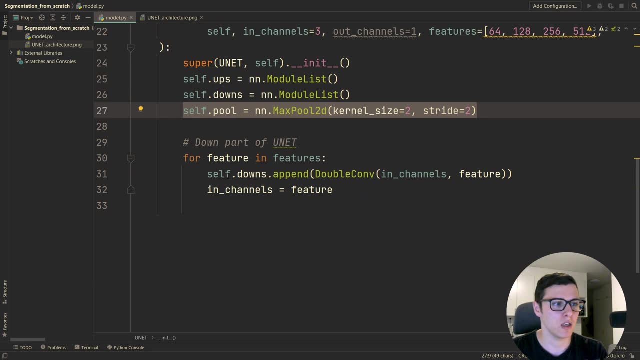 all those calm layers, All right, and we're going to use this pooling layer in between in our forward method, but you'll see that pretty soon. So what's next? so we got to create the the up part, And what we'll do here is we'll just go through the. 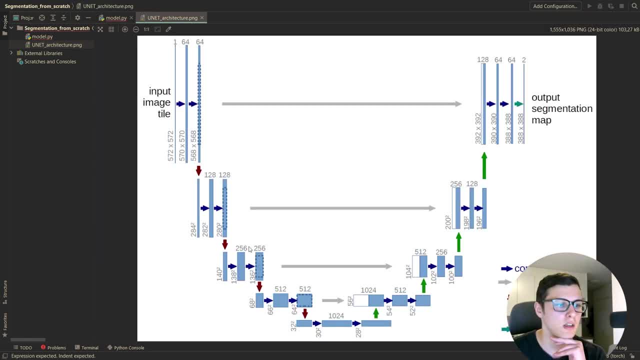 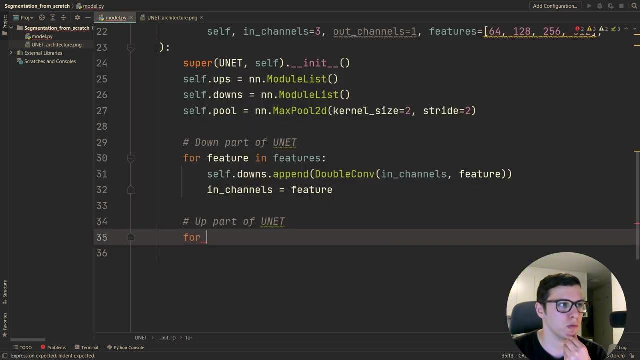 so if we look right here, what we just did is create all of these steps right here And this at the bottom. we're going to go through all of these steps right here And this at the bottom. here we'll create sort of outside of the for loop. So we'll do. we'll do that pretty soon. So 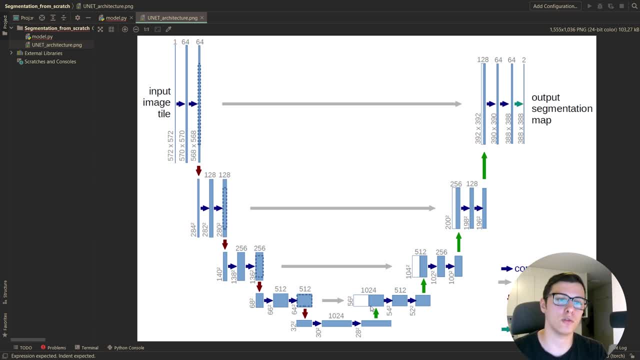 for the upsampling part, we're going to be using transpose convolutions. what you could also do here is just use a sort of a bilinear and then a calm layer on afterwards And you know, that's sort of what they, what they've started to, or they've done it for a long time. But if you look at, 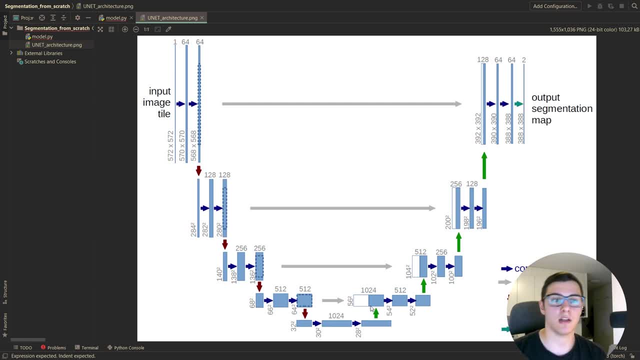 Gantt's, for example, in program they realize that transpose convolutions create these artifacts and they started to use that. So I would imagine that would be a better option and a cheaper option probably. But you know we're not going to do that. we're going to use similar approach. 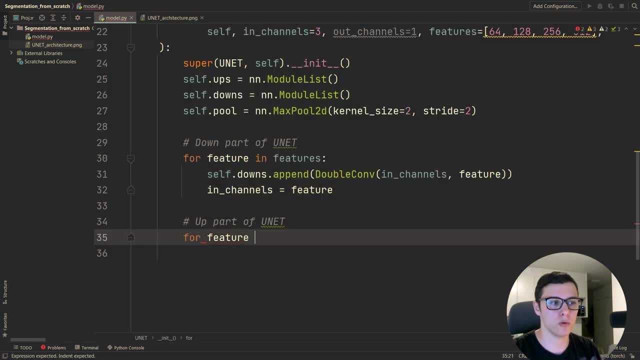 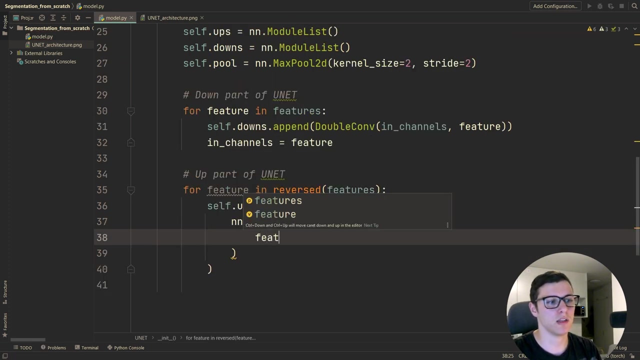 to the paper. But so what we'll do is we'll go through the features And what's important here is that obviously we're going to go from the bottom and up. So we'll do for feature in reversed of features. in our com transpose 2d we'll set the in channels to be featured, times two And the. 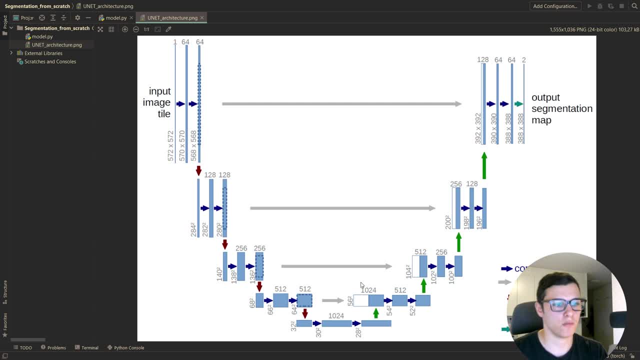 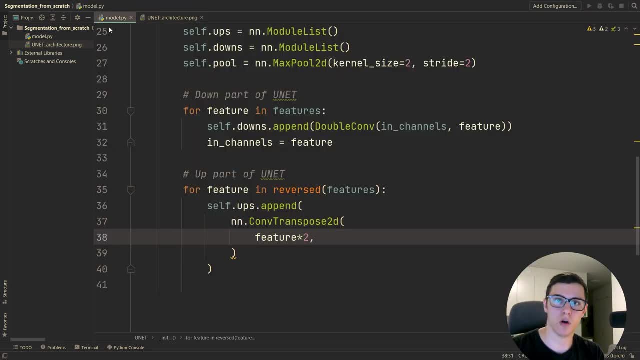 reason for this is because we're going to be adding the skip connection, So it's going to be, you know, 512 times two, And that's going to be the case for, for all of the transpose we're going to concatenate along the channel dimension, sort of this. 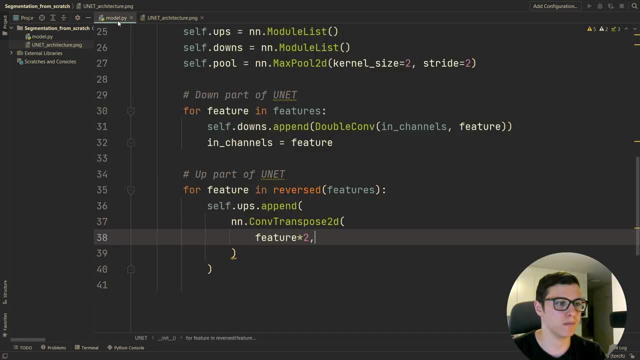 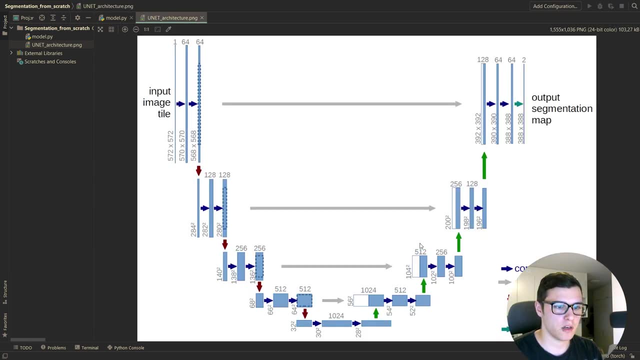 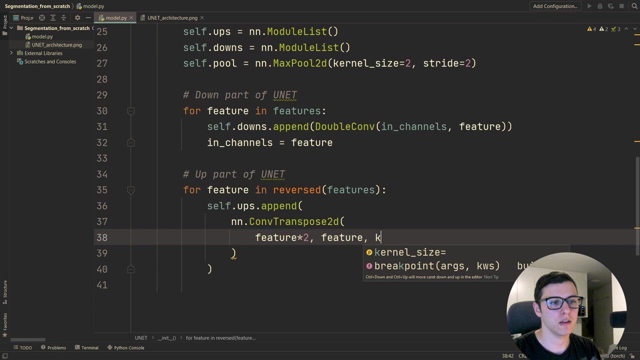 this gray skip connection right here for all of those sort of up layers, Then the output is just going to be feature. So, as you can see, it's right: here is 512. And then here it's 256. And then it's 128. So we'll just do it to feature. the kernel size is going to be: 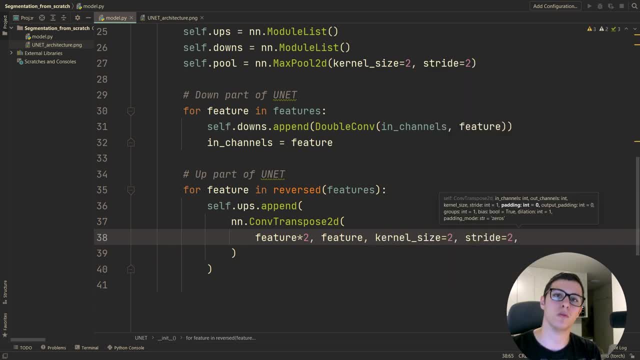 two stride is going to be two, So this will sort of double the height and the width of the image. All right, what we'll do next is we'll just append also a double comp, So we'll do feature times two to feature. 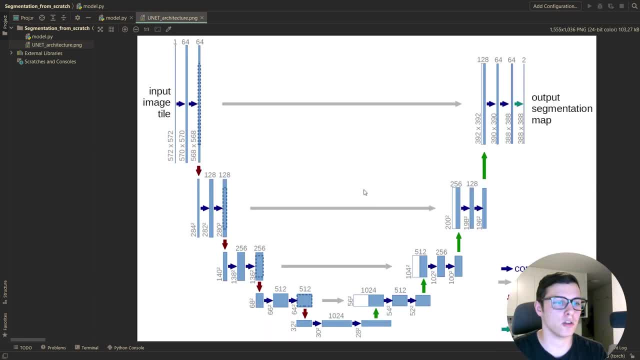 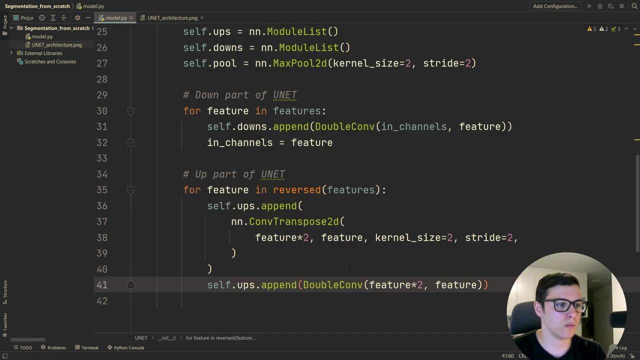 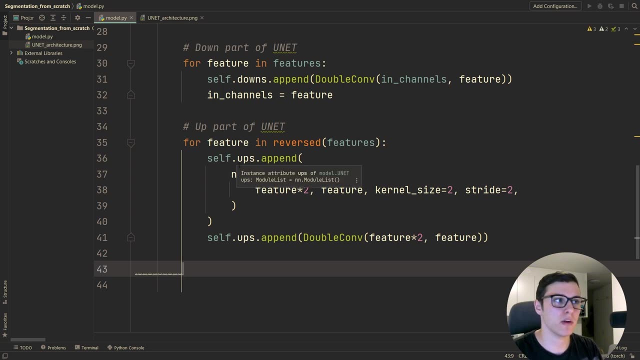 And so why we're doing that is because we're going to do up, and then we're going to do two columns up, two columns up, two columns. So that's what we're doing, appending this right here And let's see. So what's missing right now? sort of this at the bottom right here. 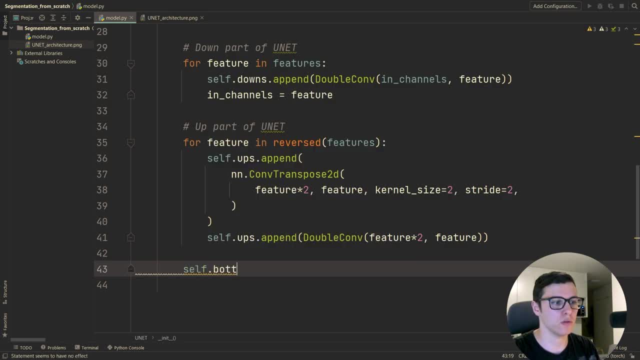 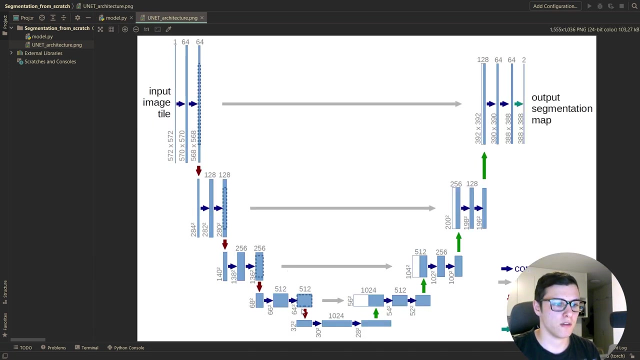 which I'll call a bottleneck layer, So we'll just do self dot. bottleneck is equal to double comp Of features minus one, And so what we're doing- features minus one- is because we want this 512.. Right, that's the last in our features list And we're going to map that to features. 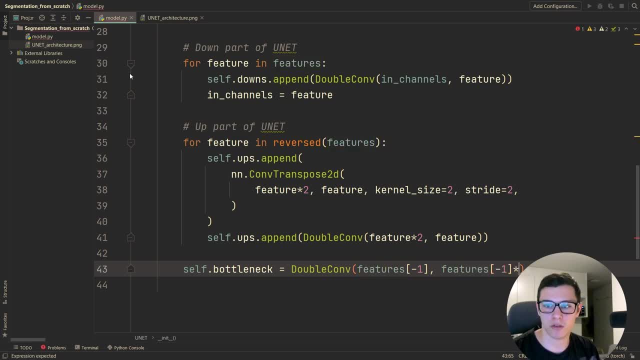 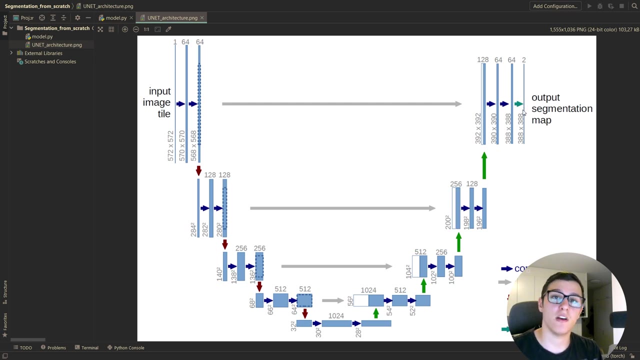 times five features minus one times two: right, it's going to be 1024.. And then, for the last thing we're going to do, right here at the top, we're going to this sort of the absolute. last thing we're going to do is a final calm, which is going to be a one by one. 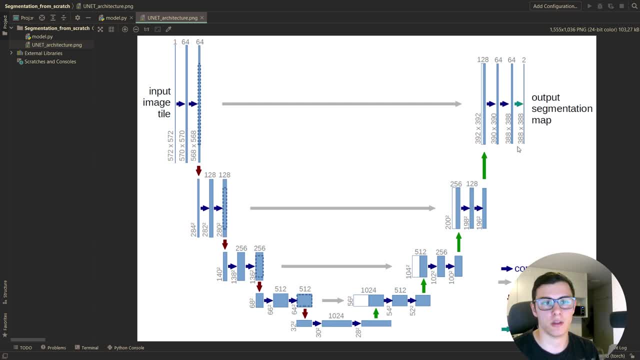 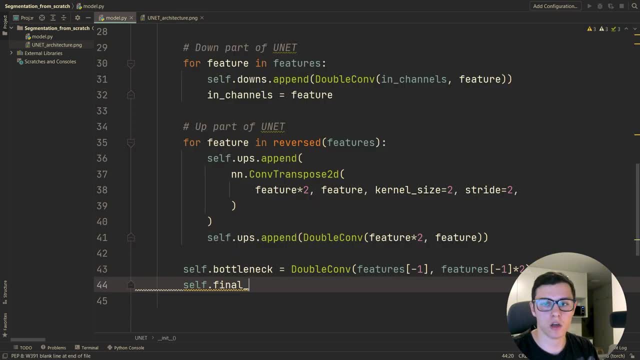 calm And it doesn't change the height and the width of the image And really what? what it does is just change the number of channels. So we'll do final calm. That's just going to be a common to the layer of features of zero, to our channels, And the kernel size of that is going to be one. 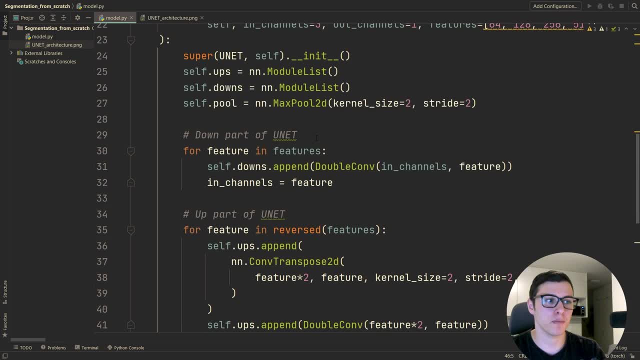 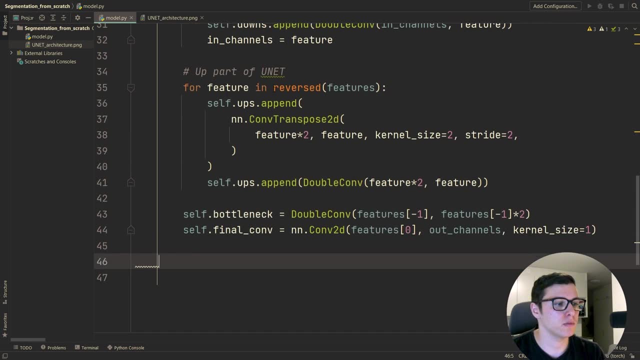 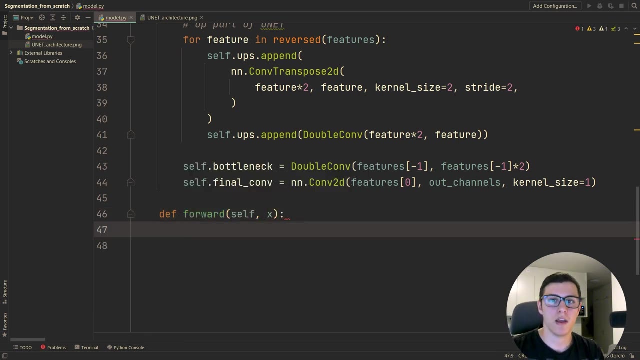 All right, hopefully I didn't go through this too fast, So that's just the inner part. Now we've created all of the modules that we're going to need for the forward step, And so let's do it: Define forward self comma x, And what I'm going to do is I'm going 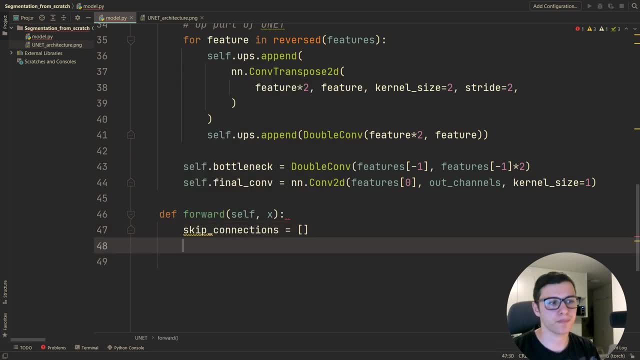 to create a list. I'll just call that skip connections, And you guessed it. we're going to store all of the skip connections in that one. So let's see what we're going to do is we're going to do for down in self dot downs. So you know, that's the the downward part. 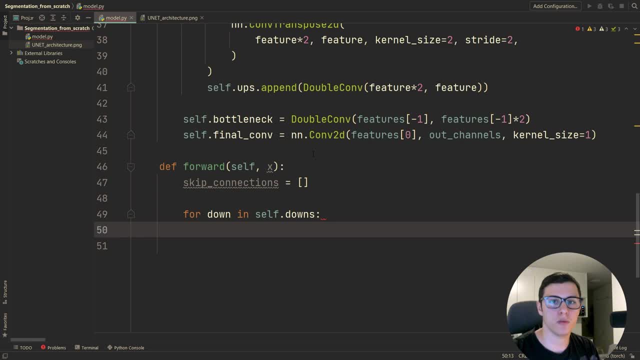 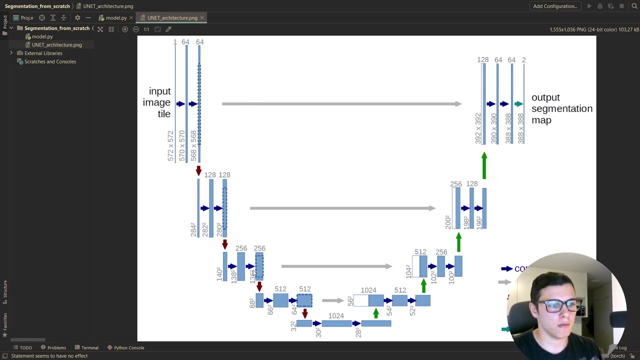 right, That's what we do first, And for the downward part we just do: x equals down of x, then we add the skip connection right before the down sampling. So we do these two columns, add the skip connection to that which we're going to use later on, And we do that for every, every. 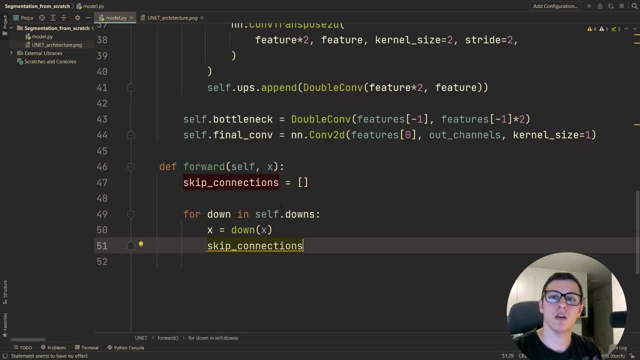 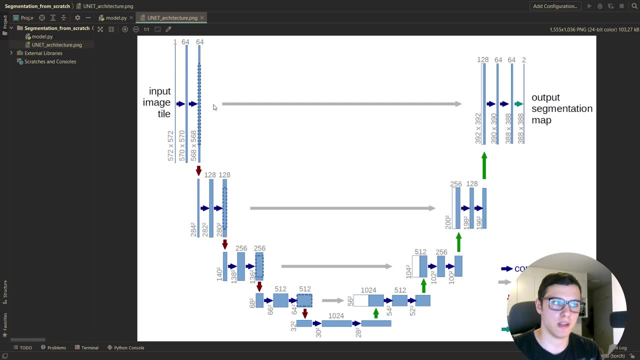 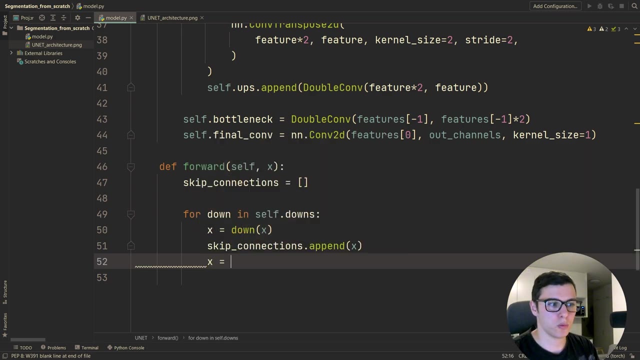 part. So skip connections. dot append x. And I guess the ordering is important to know here: the first is going to be the one with the highest resolution And then the last will be with the smallest resolution, And what we'll do next? self pool of x. And that's it for the downward part. 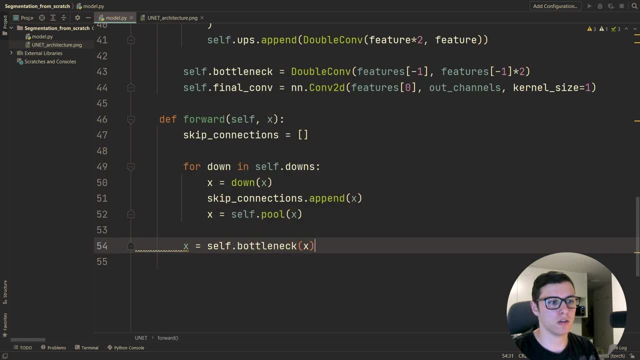 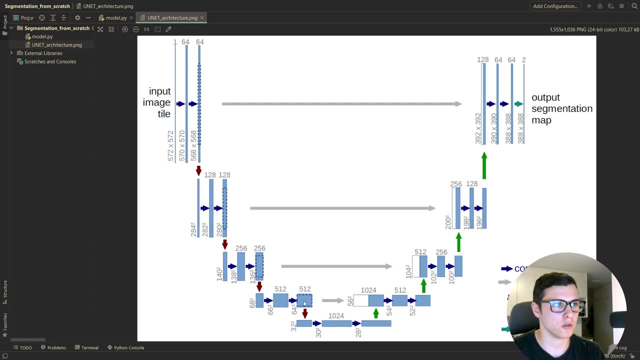 Then we'll go through the bottleneck layer right. So what we've done in these, in this for loop, is we've done all of these steps until we'll we're right here. So we've done the pooling and we just want to do this double. 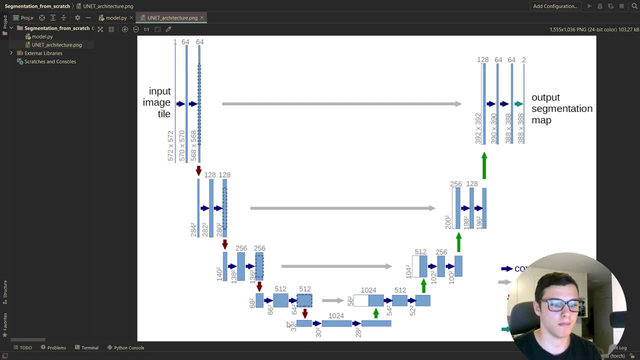 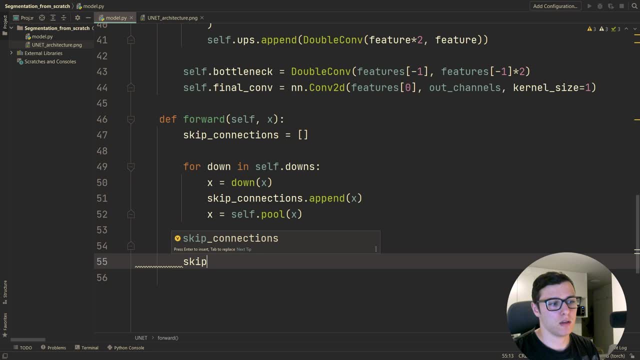 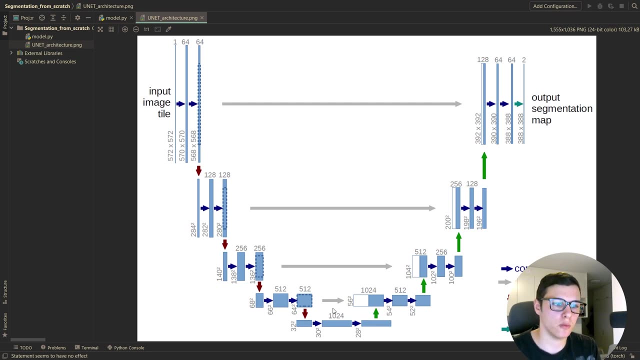 comm right here And this double comm will be a self dot bottleneck. All right And all right. so one thing we're going to do just to make the skip connections a little bit easier is because obviously we want to sort of go backwards in that order when we are doing the. 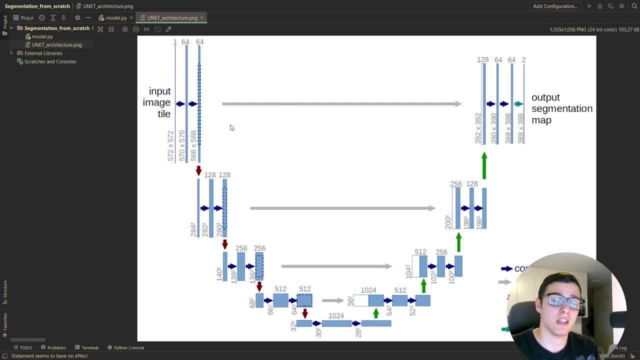 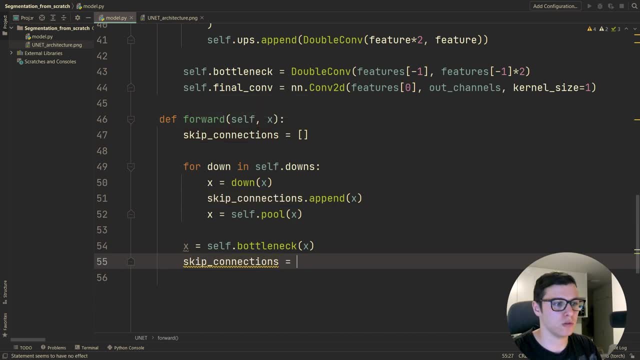 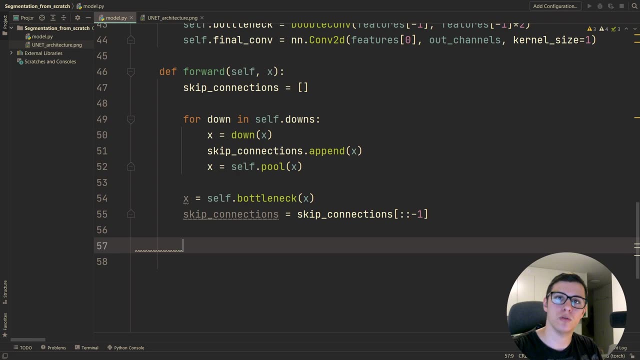 concatenation, As I said, the first element is going to be the one with the highest resolution. So we'll just reverse that list. So skip connections. we're going to do skip connections and then just reverse that list, And then what we'll do is we'll go through the self dot ups. 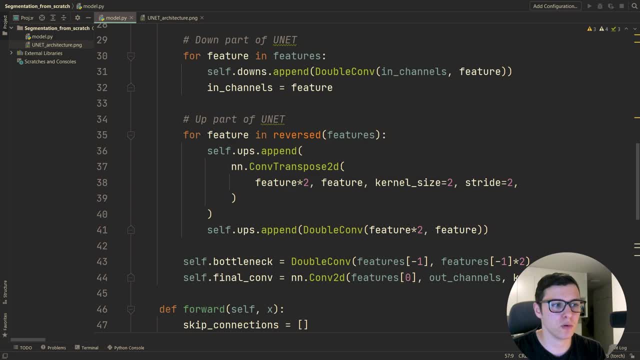 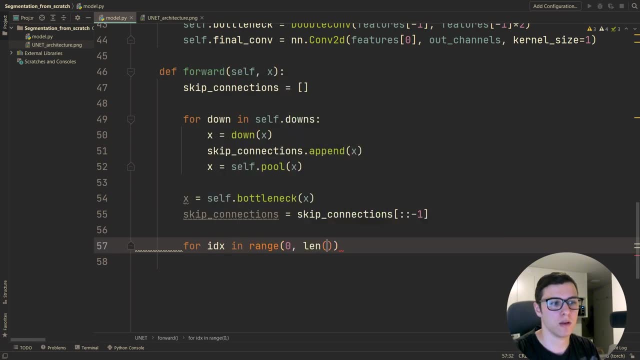 So the self dot ups that we created, we added a com transpose to D and we also added the double comp. So what I'll do here is I'll do for index in range of zero length of self dot ups And then we'll do a step of two. All right, 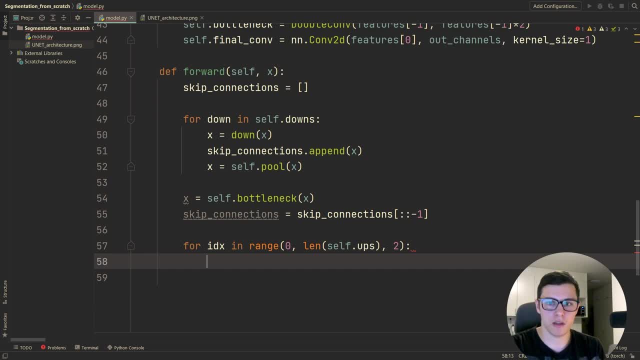 The reason for that is because I want to do the the up and then double comp. So up and double com, And that's going to be sort of a single step. That's why we're using a step of two here. Again, there are probably better ways of doing this. Let me know if you think of a better way. 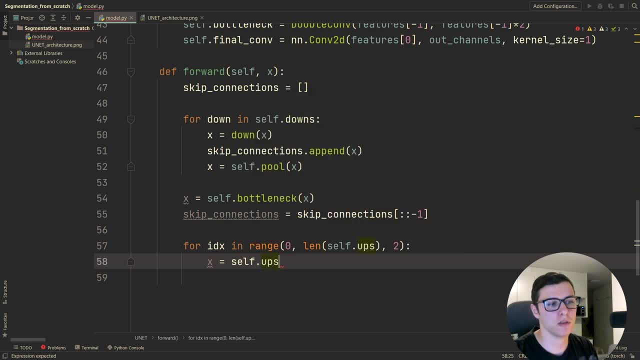 to do it. But so what we'll do is we'll do self dot ups of that particular index, so zero in the beginning, right, We'll do of x, of that, What. so what we're doing here is is we're doing the com transpose to D, right, What we'll do then? 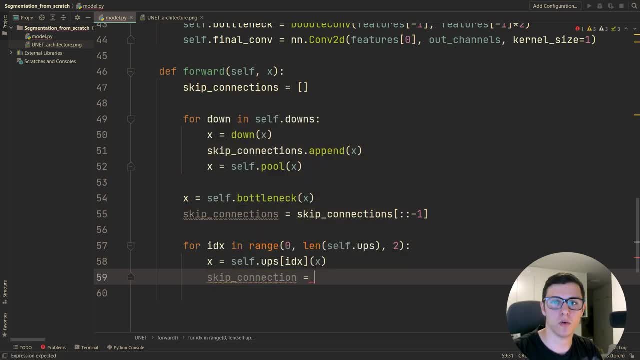 is we'll add the skip connection, So we'll do skip connection equals skip connections of index integer division by two. And why we're doing that is just because we're doing this step by two right there. So obviously we want to still take a skip connections in, you know, a linear sort of a step of 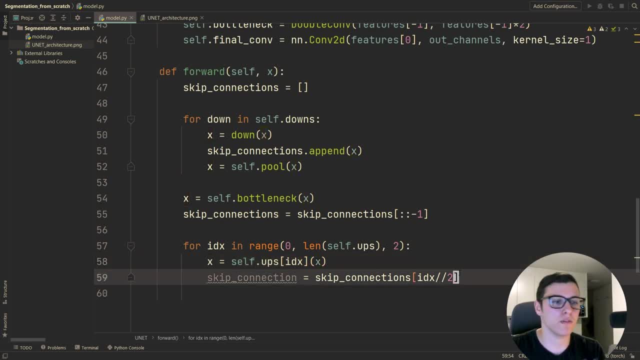 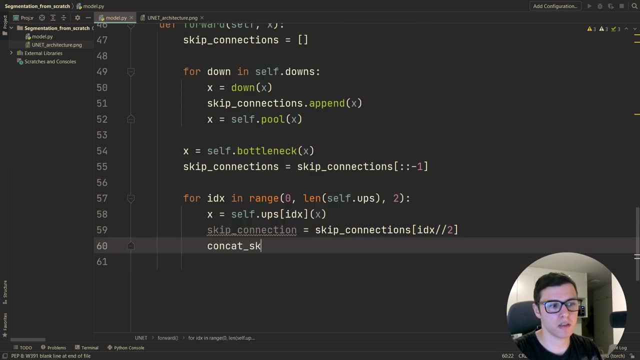 ordering. So that might be a little confusing, but nothing too too difficult there. Then we'll concatenate them. So we'll do concatenate skip, sort of concatenate the skip connection. we'll do torch dot concatenate skip connection and the x and we'll add them along the channel dimension right. So we have. 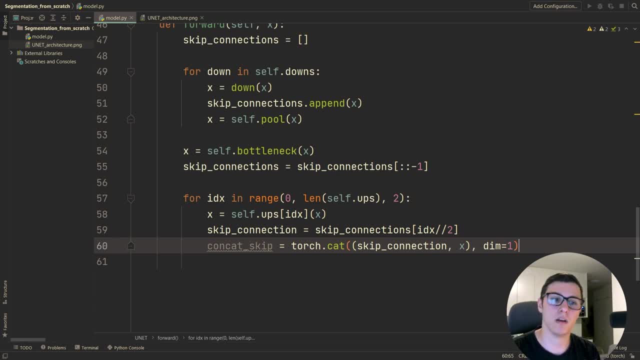 batch channel: height, width, So we'll add them along dimension one. Lastly, we'll just do self ups of index plus one of concatenate skip. Right, that's it. So what we're doing here is: we're doing the upsampling. Alright, so it's following this: we're doing the upsampling. 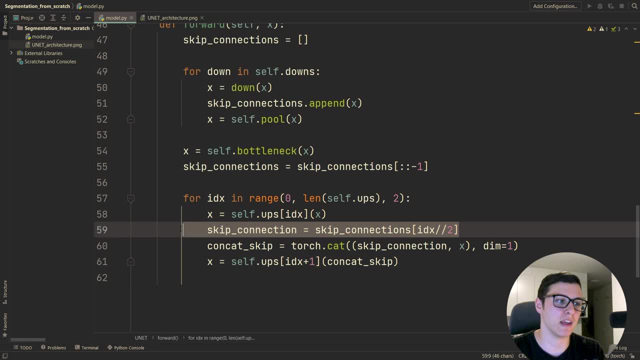 we're concatenating, No, sorry, Okay, so we're getting the skip connection And then we're concatenating, Then we're just running it through this double comp And then the last thing we're going to do is just return self dot. 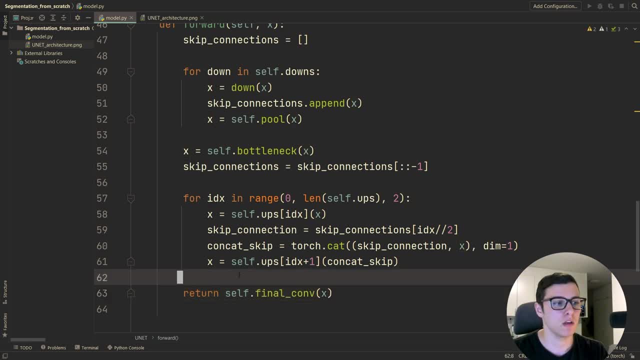 Final calm of x. Right, So I think sort of we're done, But I guess I guess one improvement we could make here is, let's say, you're not in inputting something that is perfectly divisible by two at every step. Right, that's, that's what is going to happen for this. 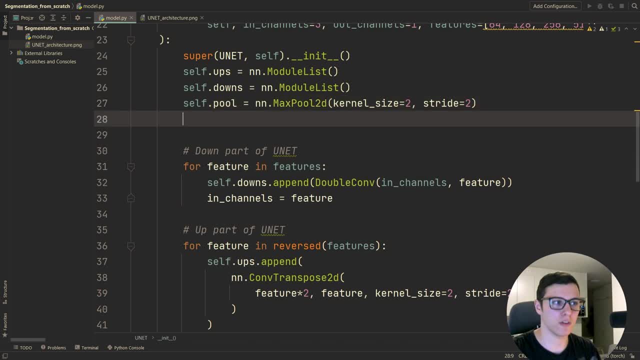 self dot pooling layer. So for just to give a concrete example, let's say we input 161 by 1260.. What's going to happen here is that the max pool is going to take this into an 80 by 80. So it's going to floor the division by two. But so we have 80 by 80. And obviously, when we then 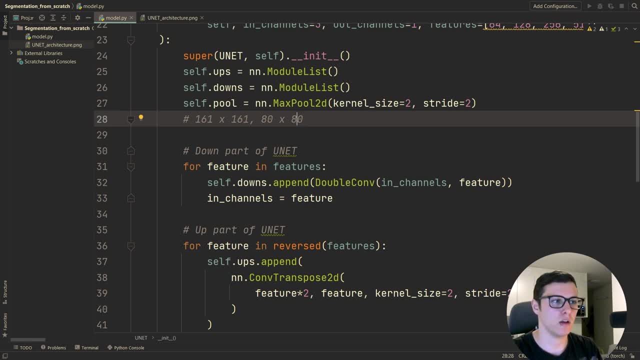 up sample that's going to create an output. So the output will be 160 by 160.. Meaning we won't be able to actually sort of concatenate the two right, because they need to have the same height, width, And that's a problem. So you could solve that by always choosing an input. that is perfectly. 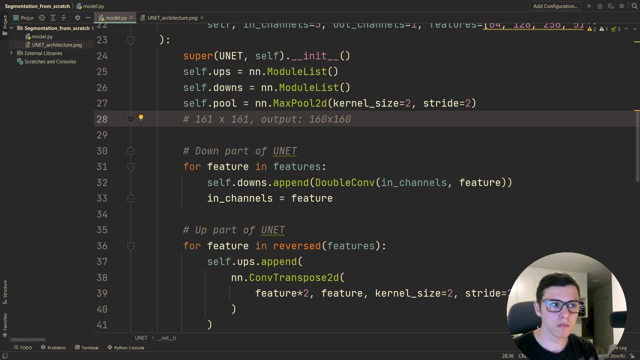 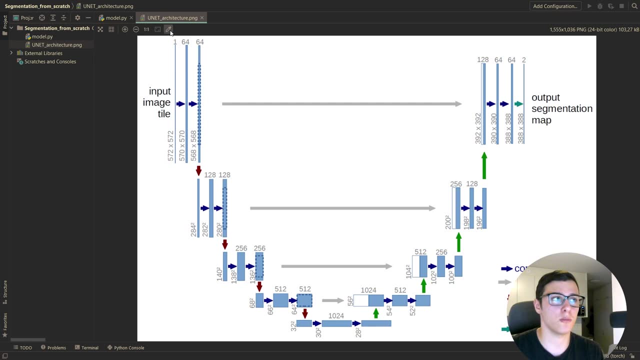 divisible or, I guess, divisible by 16.. Because it's going to be four steps, right? So one, two, three, four, all of those are going to be divided by two. So that's one solution, But of course, 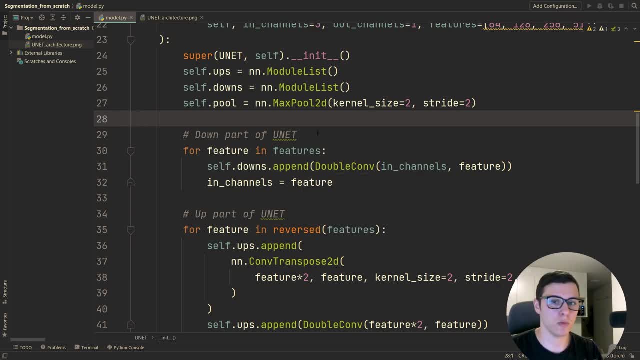 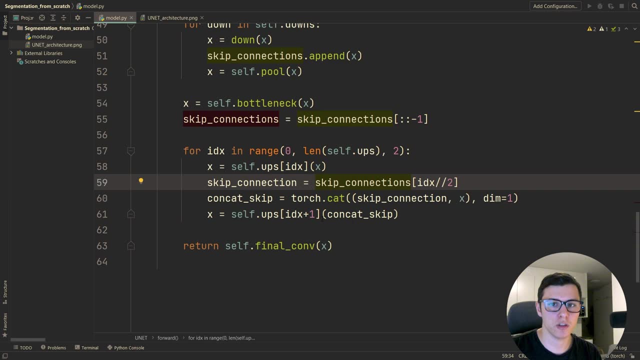 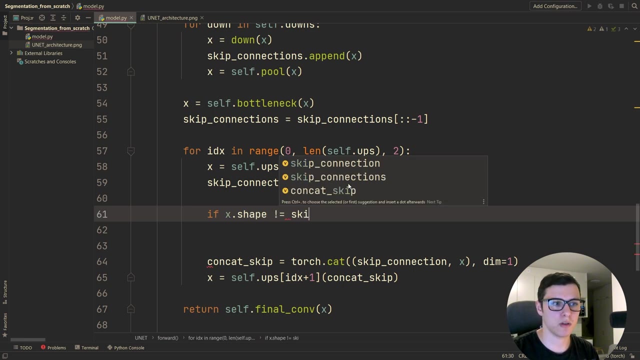 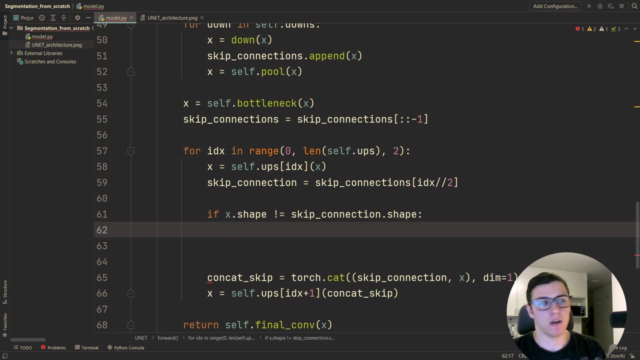 we want to make our implementation general in that way. So what we can do is, when we're concatenating them, we can just check right here if they don't match. So if x dot shape is not equal to skip connection dot shape, then you can solve this by different methods In the paper which is 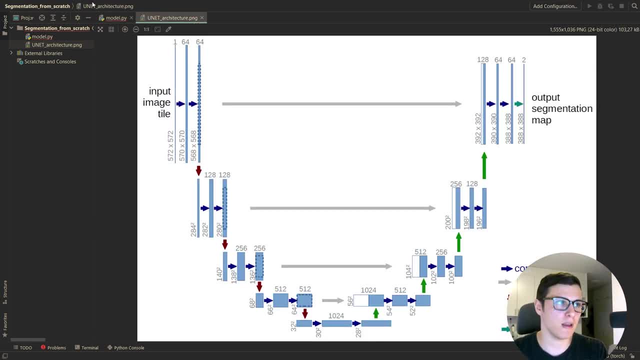 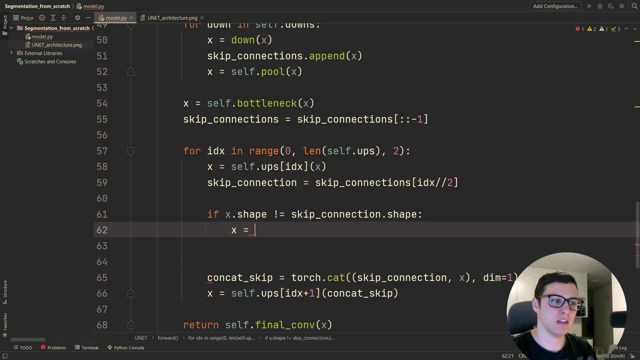 a little bit different, but they used cropping right here. What you could also do is you could add padding And what I what I did is I'll just do a resizing, So I'll use this TF, the torch vision functional, and we'll do TF dot resize. 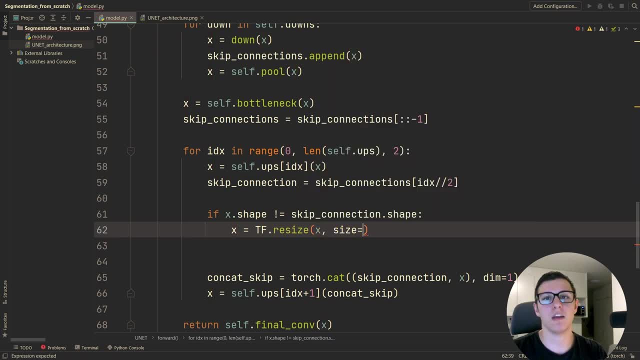 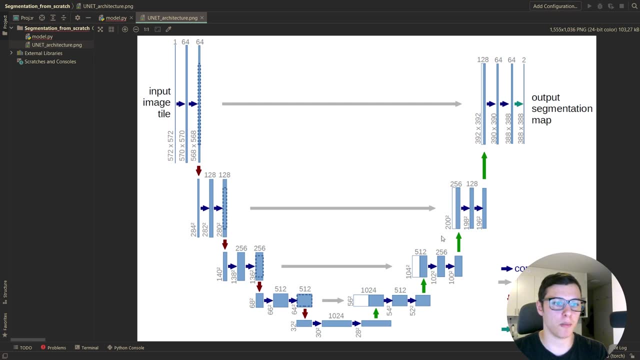 of x and then we'll just set the size. So, if you think about it, the, the x which is coming from the sort of the upward part here, it's always going to be smaller than what was, you know, down sampled, just because of that reason that that max pool always floors the. 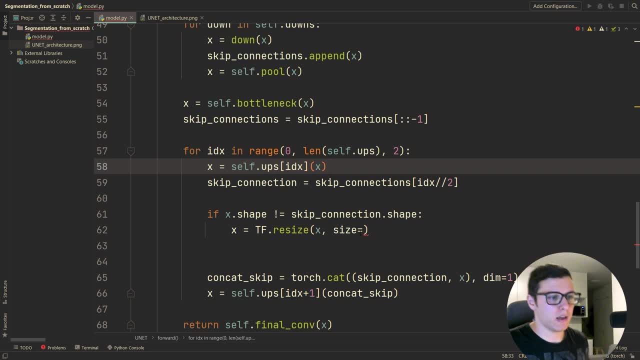 the shapes. So. so I guess it's just important to resize the x, And I don't think this is going to sort of impact the accuracy too much, I hope, because you know it's just going to be sort of. 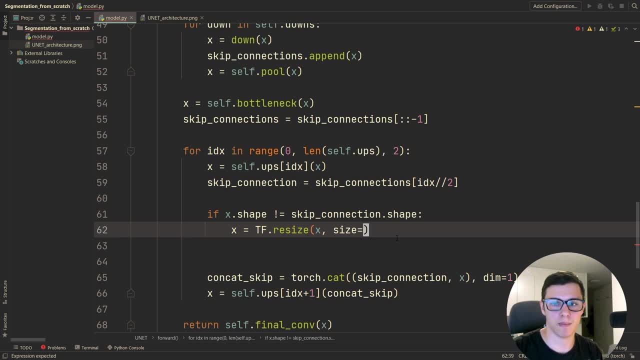 a one pixel difference, And so I don't think it matters too much. I haven't tried this extensively, though, But so skip. connection dot shape. So what we'll do here is we'll just take out the height and the width, So we're skipping the batch size and the number of channels. 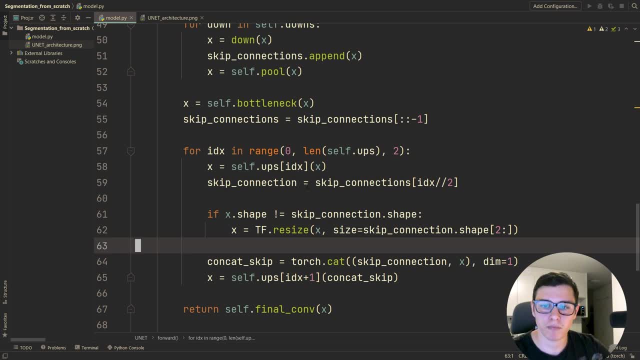 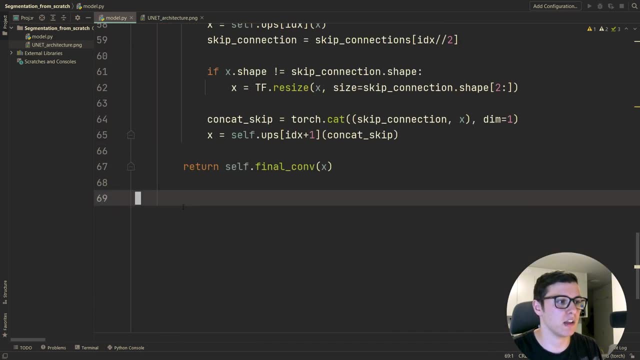 But that's all we have to need for the resizing. All right, So that was, you know, unit in, I guess, 67, lines of code. not too bad, And hopefully it's understandable and readable still. So we'll just create a test right here. the test torch dot random, let's say we have 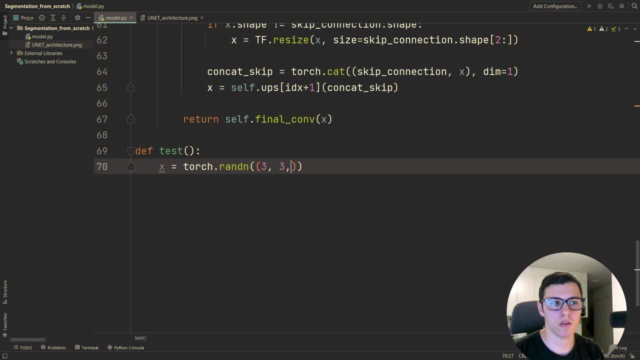 a batch size of three input. let's see one channel And then we'll do- I don't know 160, 160,, which is perfectly divisible- And then we'll do model unit in channels will set to one out channels will set to one. 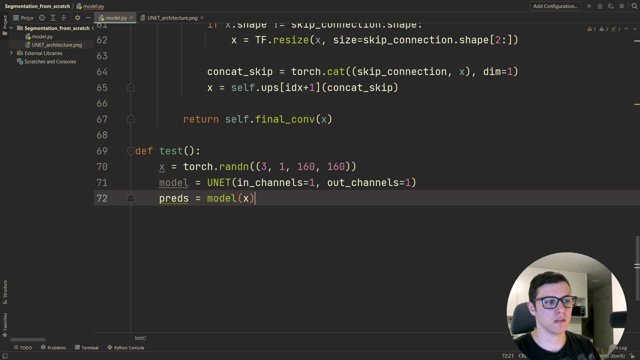 will do predictions is model of x And what we want to do, or make sure, is that the input is the exact same shape as the output. So we'll just do print print dot shape. print x dot shape And maybe also assert preds dot shape equals x dot shape, And we'll do. if name equals main, then we'll run. 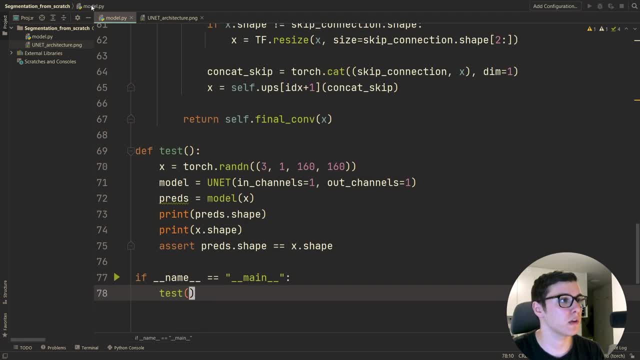 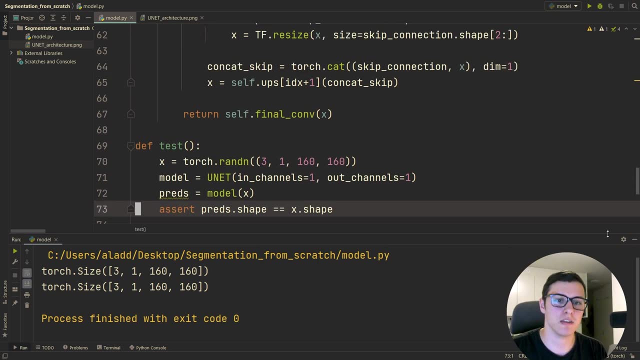 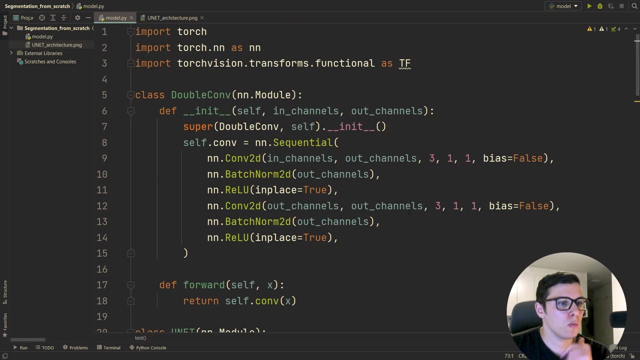 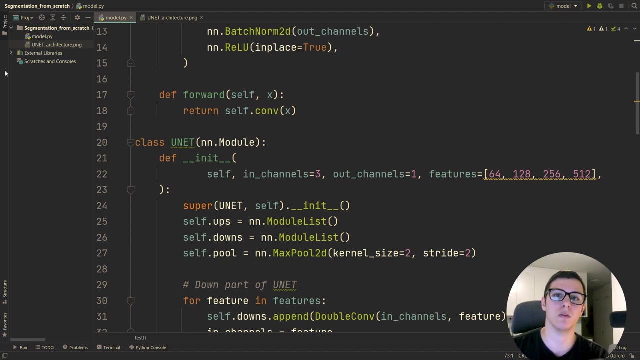 that test right there. All right, pretty good, Let's see if we can run this now And we get the result. That was, that's amazing. I always make mistakes. All right, pretty nice. So what we're going to do next, I think, is we'll look at the data and we'll set up the data loading part, And then 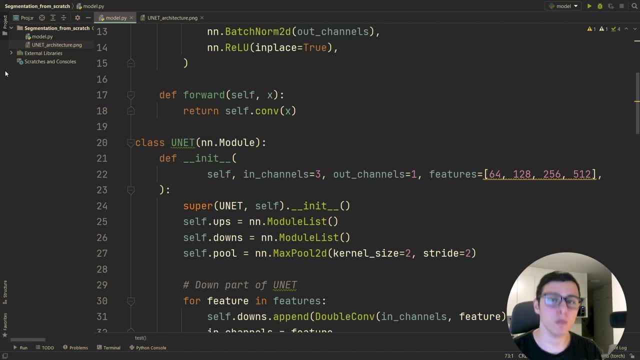 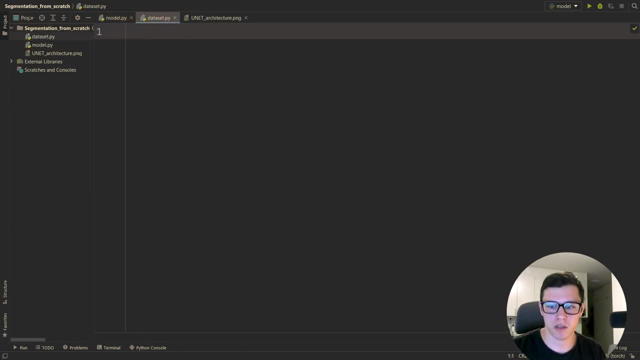 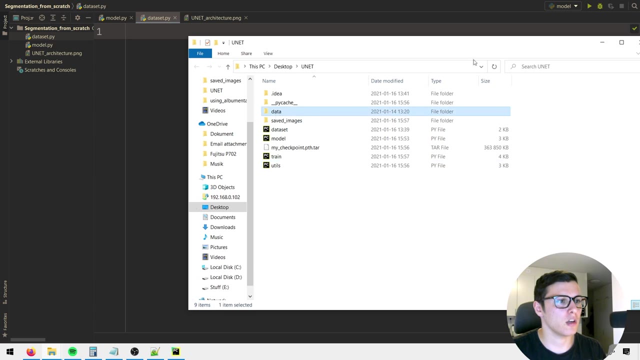 we'll actually do our now. we'll do the training, set up the training. So let's just create one called data set, And what I got to do first here is actually copy in. So this is the code that I've created, And what I'm going to do is I'm going to copy in that data into our folder right here. 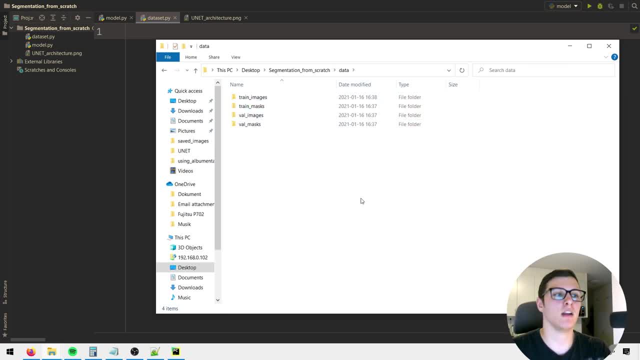 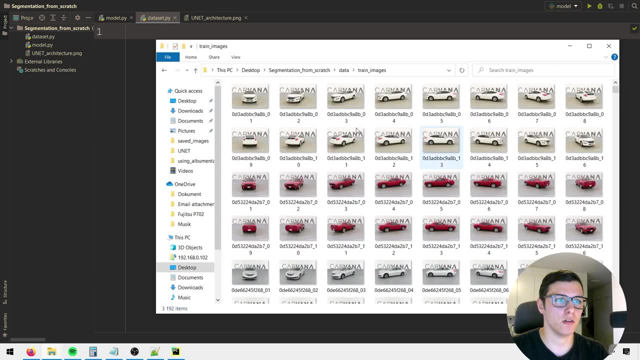 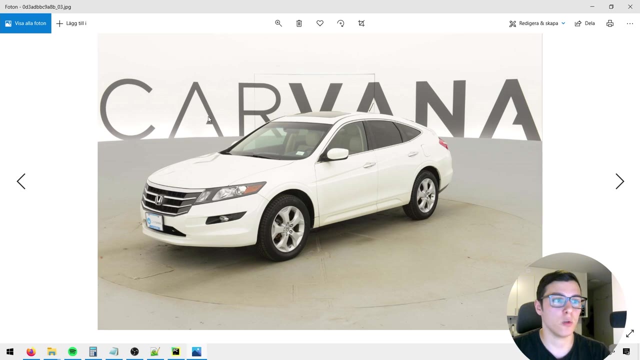 Alright. so what I've done is just put in the data right here And this. you can download this from Kaggle. All I've done here is I'm just taking the training images, which are, which look like this, And let's see if I can pull this up. So that's how they look like, And what they want is the. 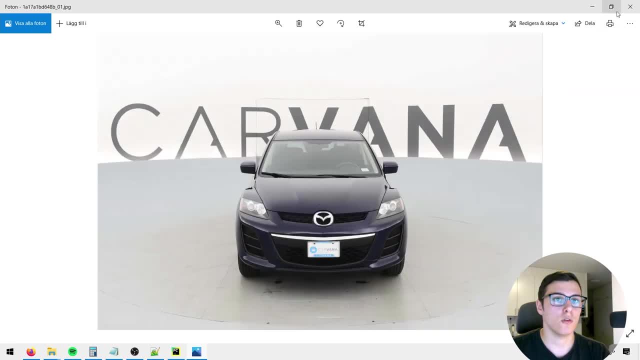 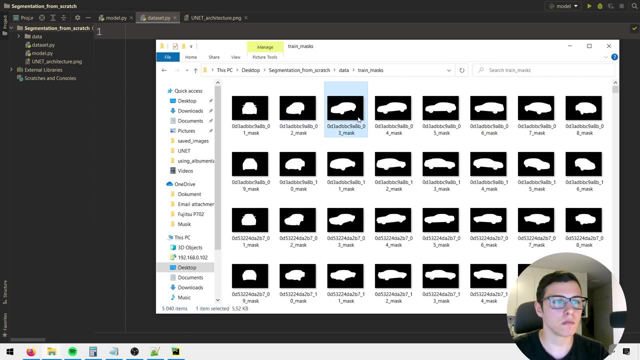 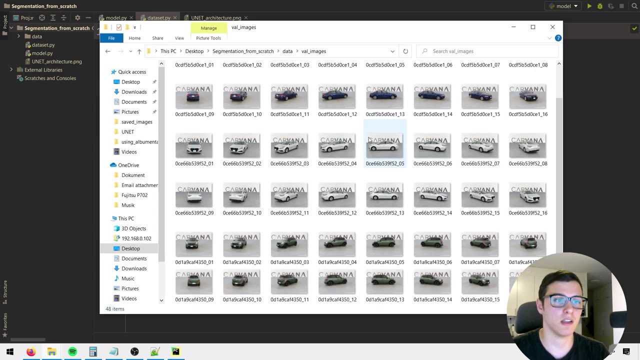 segmentation for the, for the car, And so you know the, the, the training masks, looks like this, And then and then, what I did is I just took sort of a couple of examples- 48 examples to be specific- to a very small validation set, And so that's how the data set looks like. you can download it from Kaggle. 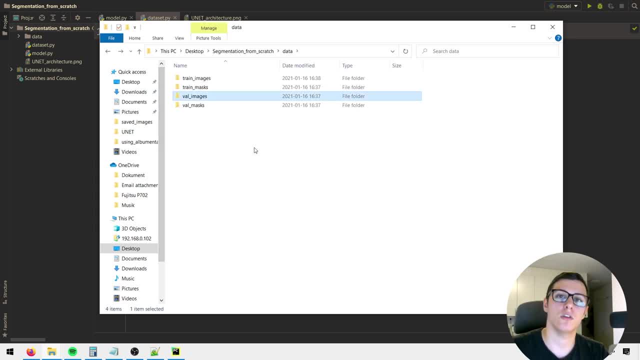 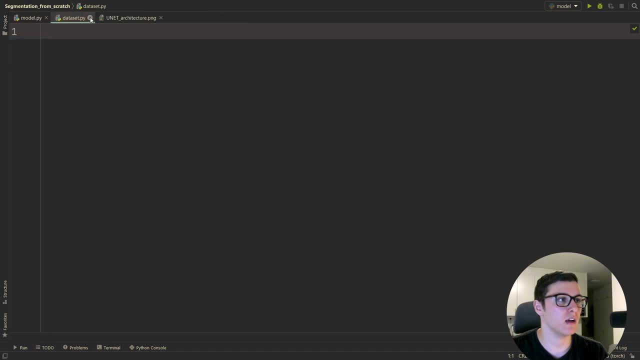 there's going to be a link in the description. So what we want to do now is set up the data loading part. Alright, so for this we're going to go ahead, and we're going to go ahead and we're going to import the data. So for that we're going to use OS. we're going to import pill, I guess from pill. 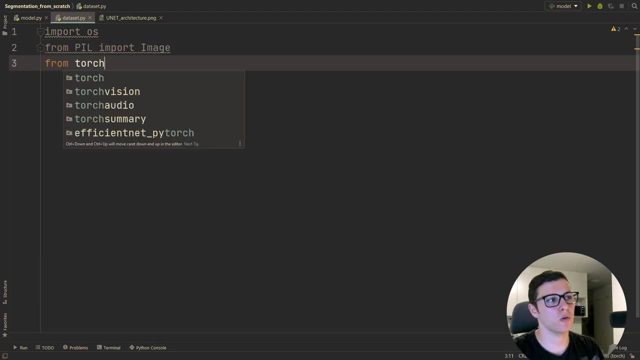 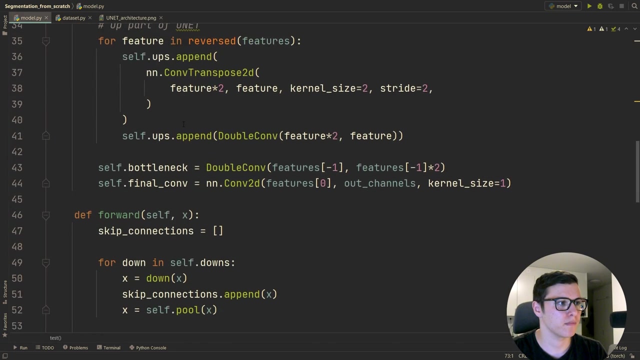 import image. then we're going to do from torch utils dot data import data, set important numpy as NP, And I just thought of one thing we could do actually on the model. So in the model right here I chose this 160, which is perfectly divisible. 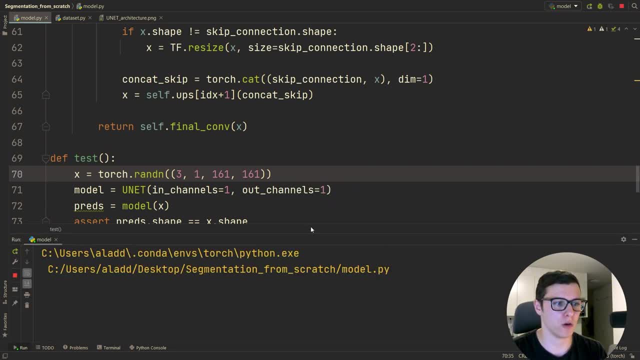 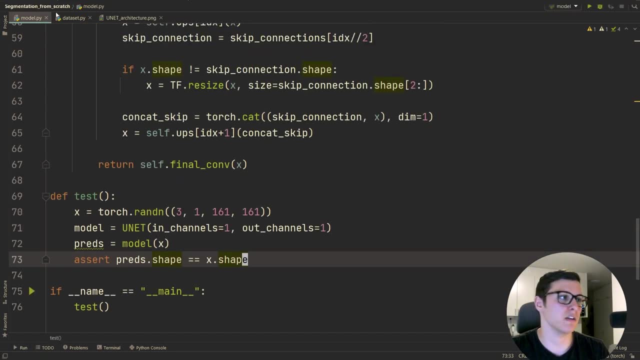 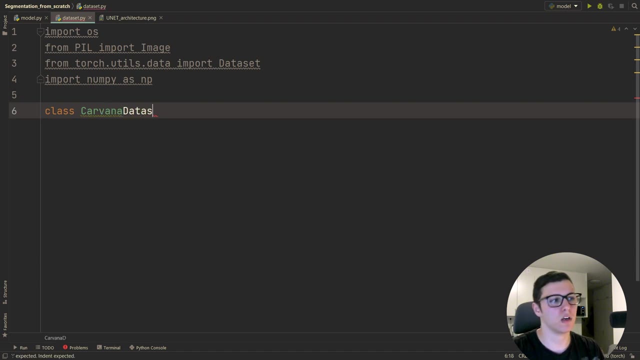 one and make sure that it still works for the model. Yeah, and there's no error, right? So the assertion was was okay, And that means that our resizing also worked. Anyways, moving on, So we're going to create a class, we're going to call it Carvana. data set inherit from data set, Let's. 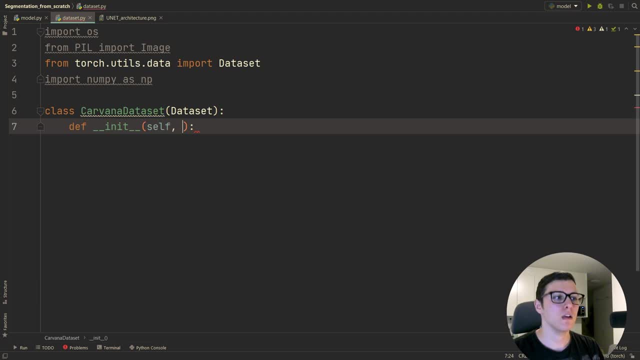 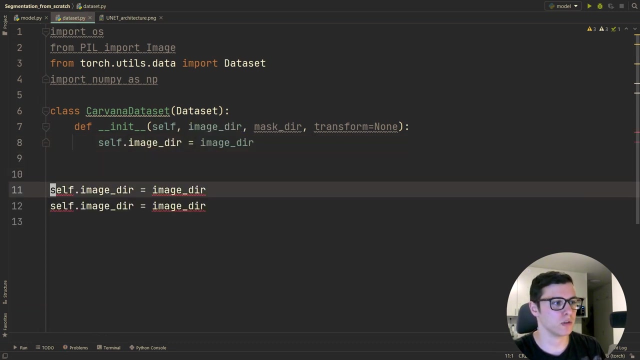 create the init method. So what we'll take in here is the image directory And we'll just create a mask directory And we'll also set transform to none by default And we'll just do self dot image directory its image directory And we'll just copy paste that two times. 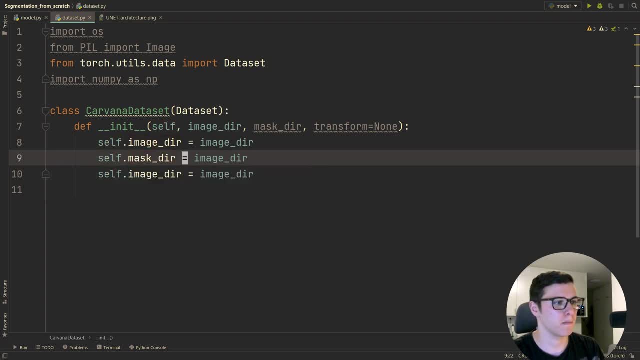 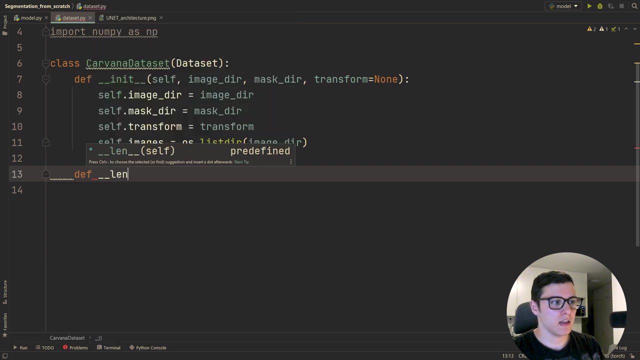 We're going to do the same thing for the mass directory. Alright, so now we have the transform, all that. What we will also do is we'll do self dot images is OS list directory of image directory, So that'll list all the files that are in that folder. So for the length of that data set is going to be pretty. 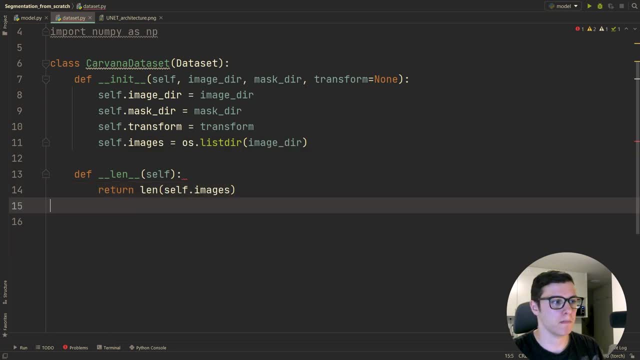 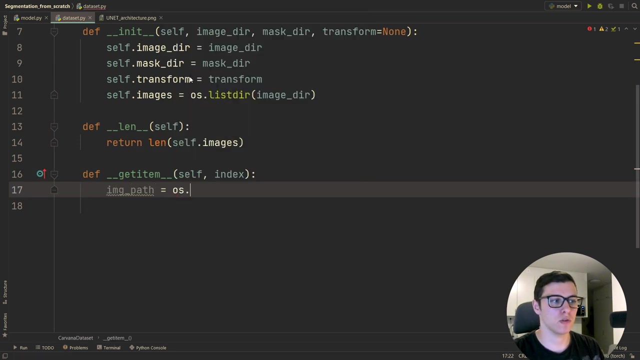 simple. we'll just return the length of self dot images For our get item, get item like that. we're going to take as input some index And what we'll do is we'll first get the image path, which is going to be always path join of the. 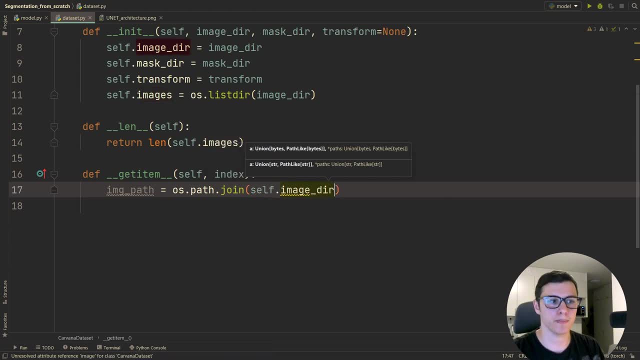 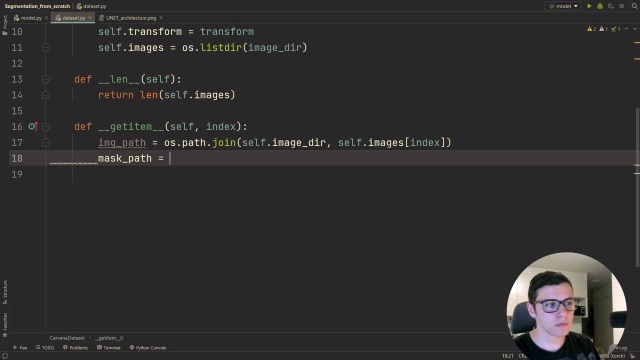 image directory. So right, so we're restored the images and then also the file of that particular image, So that'll be self dot images of index. All right, Hopefully you're following. following so far for the mask path, Pretty much the same thing, So OS. 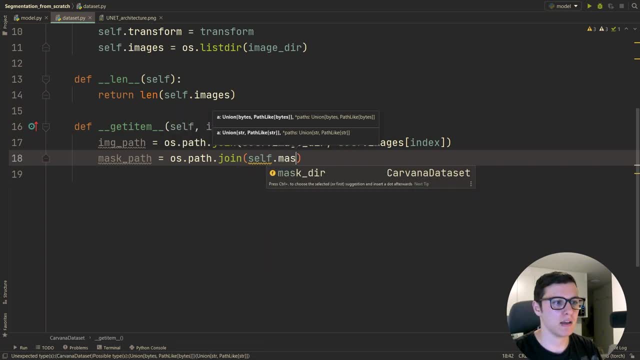 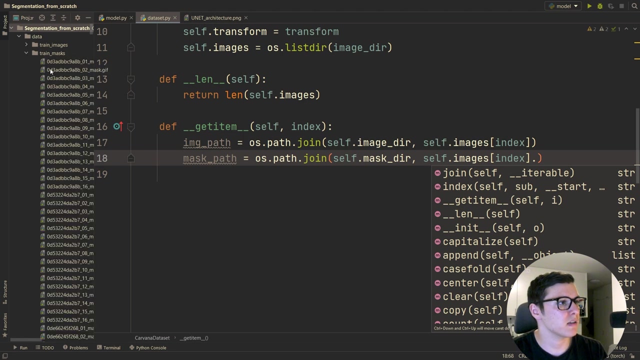 path join. but now we'll do selfmask directory and we'll also do selfimages of index. but the only difference here between- so i didn't take a look at- show you exactly. but for the train masks it has the same name but at the end it just has an underscore mask and instead of being a, i think 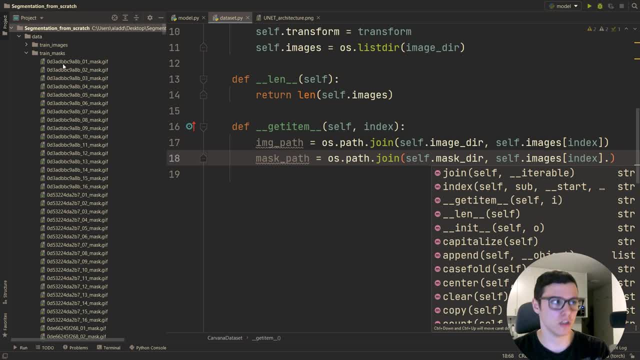 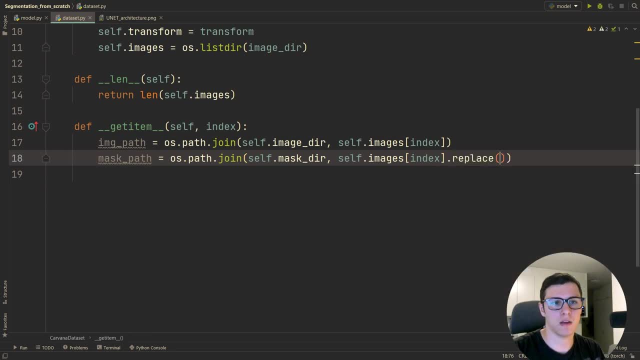 jpeg or png. it is actually a dot gif, so we gotta adapt to that. we'll just do selfimages dot replace and all we'll do here is dot, dot jpeg and we'll change that to underscore mask dot gif. all right. so now that we have the mask path and the image path, we'll just load those two, so image. 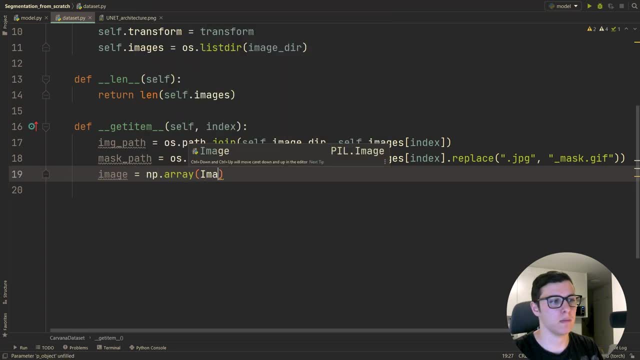 equals numpy array of you image dot open of image path. and yeah, we'll also do dot convert to rgb here. i think it's by default rgb, so we might not have to do this, but just make sure. and also why we're doing numpy over here is because we're going to be using the album mutations library, which, if you're using pill, 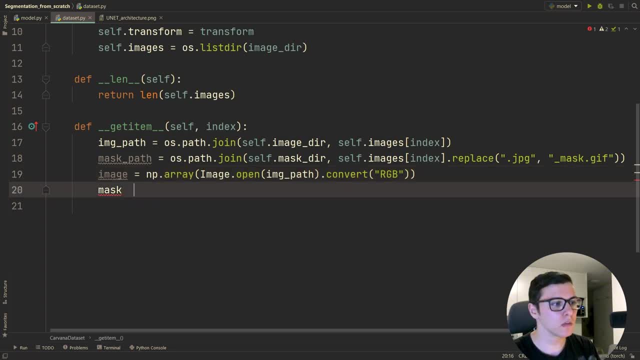 needs to be converted to a numpy array. so we'll just do mask equals a numpy array of image. dot open mask mask path. and then we're going to do dot convert l. and the reason why we're doing l here is because the mask path is is going to be a grayscale. so that's how you do that. 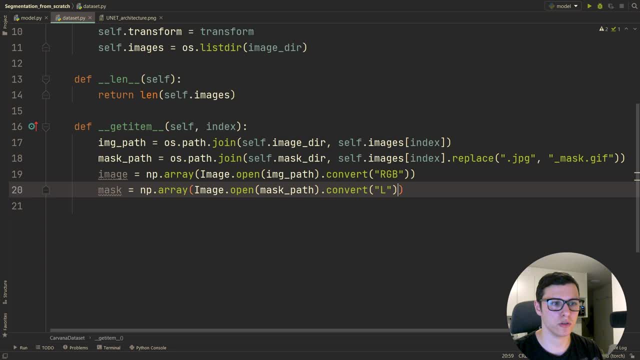 for pill. and one more thing also is we'll specify the d type to be np float 32, right? so this is going to be loaded as images between. so the i guess we have compress smo alta as d type visible, right? so we have a maintain label in here. 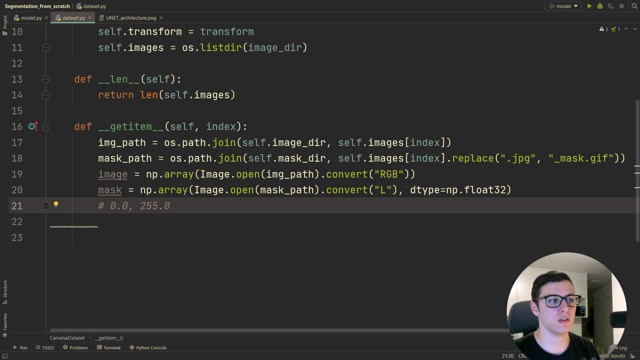 five fancy and, for now, Bot, Awesome. reason for that is because we're going to use a sigmoid on our as our last activation and so indicating the probability that it's a sort of a white pixel, and then to make sure that it's actually the correct for the labels. 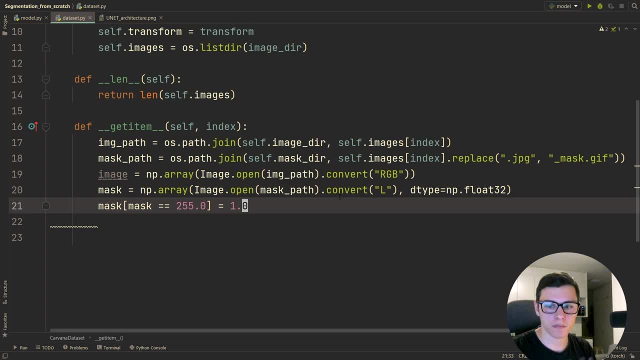 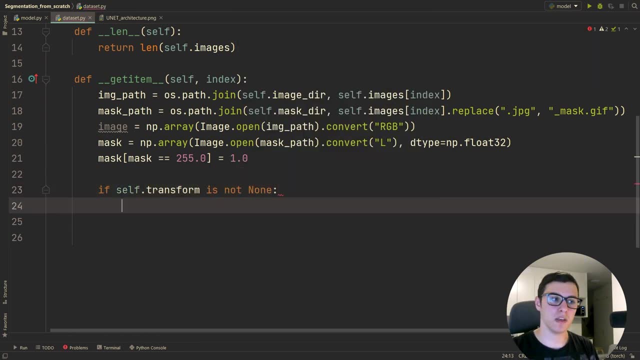 we'll just convert those two to one. all right, we'll just do. if self that transform is not none, then we'll perform the data augmentation. this is using the album intations library, so we'll just do augmentations is self transform of image equals image, and then mask equals mask, and so this you should be pretty. 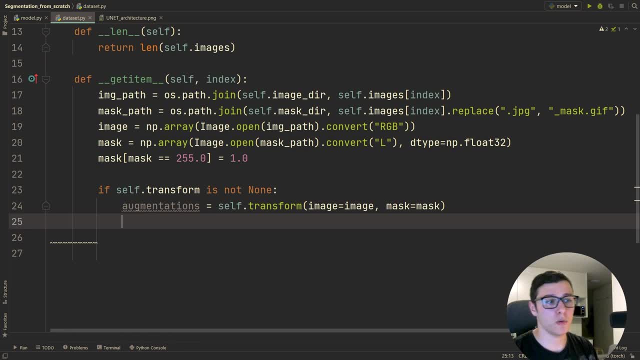 familiar with this if you watch that video. otherwise you know we're just sending in the image and the mask and then to obtain the image, we'll get the augment and we'll get the augment to the image from the dictionary with the key image and similarly with the. 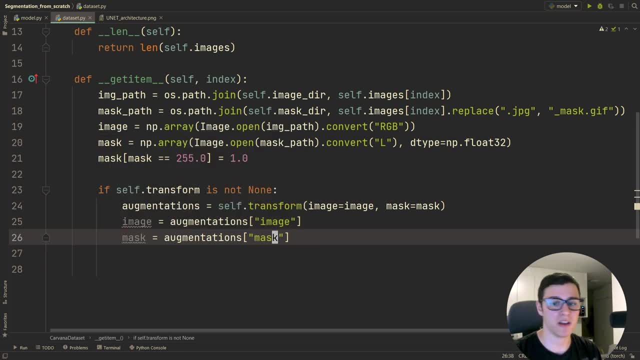 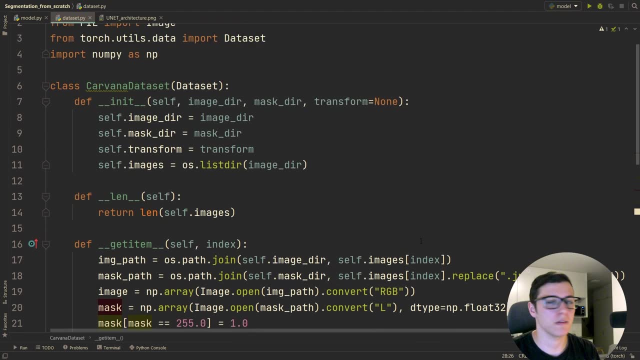 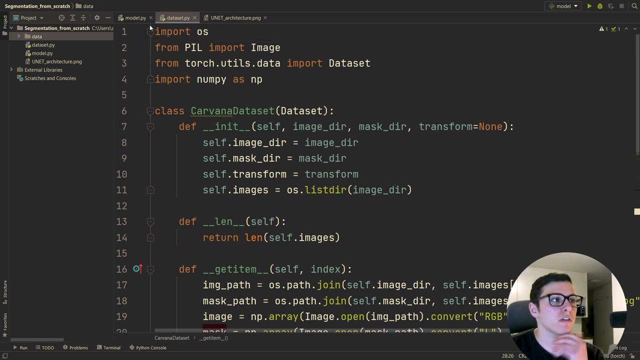 mask. all we'll do here is just change that to mask- pretty simple, to be honest, and then return image and mask. all right, pretty cool. that's for the data set, and so what? what we've done so far is create the model and the data set. I guess what? 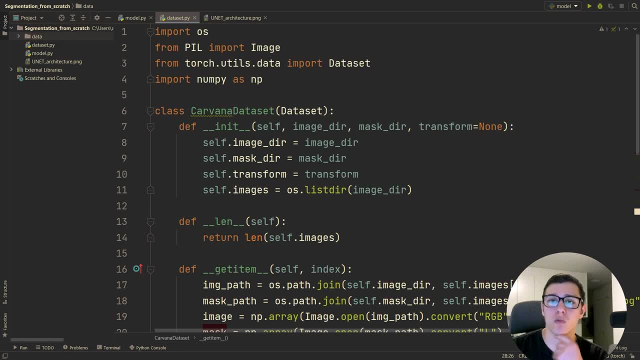 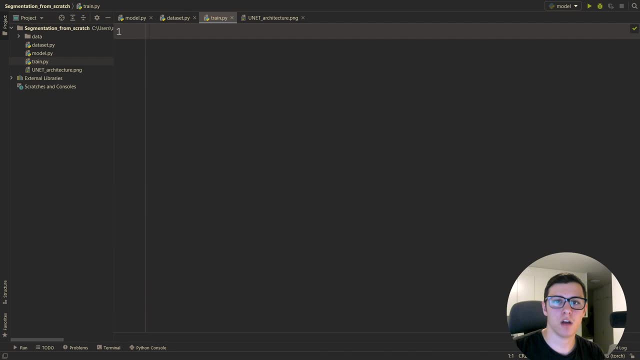 we'll move on to now is create the training part. all right, so let's just create a new file called train and I'm gonna copy paste in. let's see, I'm gonna copy paste in the imports here. so we're gonna use torch album intations as a. we're gonna need to tensor v2 tqdm for the loading. 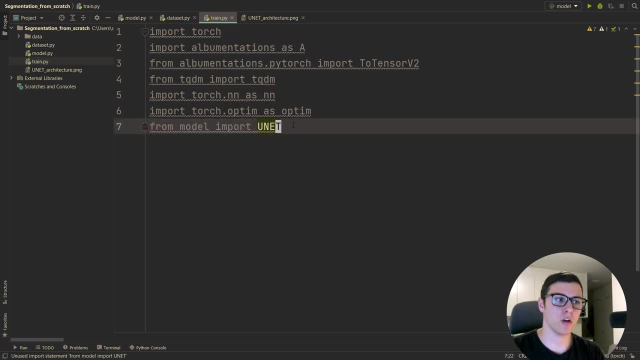 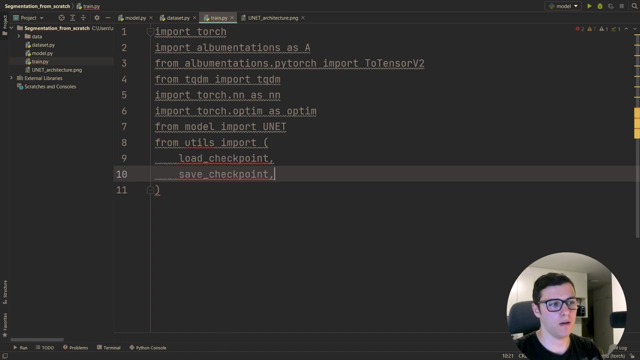 for a progress bar and then we're gonna import our model as well. and yeah, we're also going to create a utils file where we're going to import, I guess, load checkpoint, save checkpoint. let me copy paste in that as well, and we're gonna create those guests later on. but so we're gonna be using 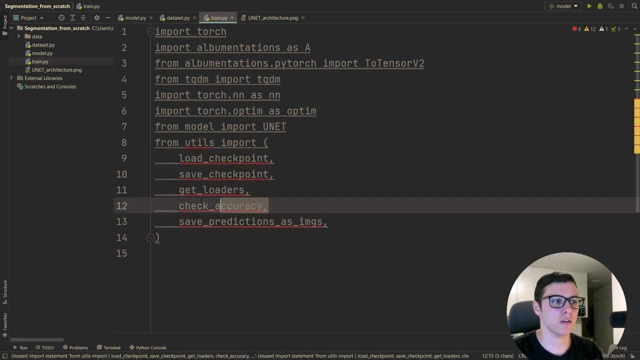 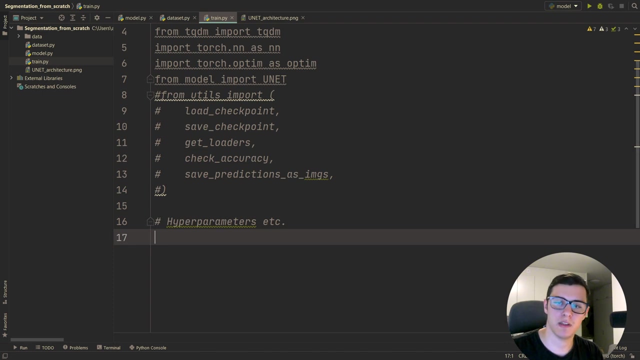 load checkpoint, save checkpoint, get loaders, check accuracy and then save predictions as images. so we'll create those later on. just I'll comment that for now. and for hyper parameters, I'm gonna copy paste in those as well. so I'm just setting the learn rate 1 e. 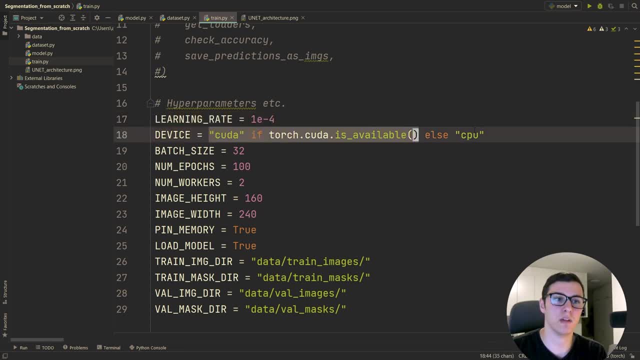 minus 4 device CUDA, if it's available. otherwise we'll set it to the CPU. batch size 32 might have to decrease that now when I'm recording number of epochs, maybe let's set it to 3 num workers, 2 image height. I'm just going to set a. 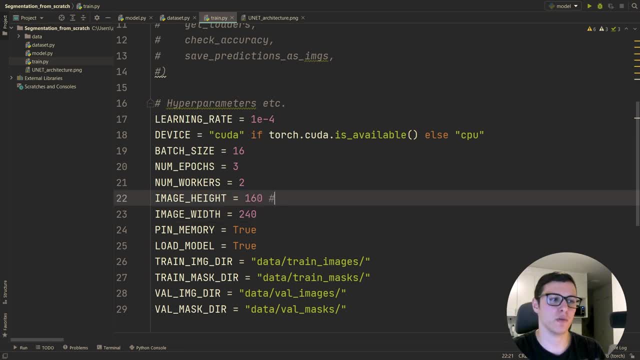 very small image height. they are originally. image height is originally 12- 12. image height is originally 12. image height is originally 12. image height is originally 12, 80 and the image width is 1918 originally. so we're just going to be. 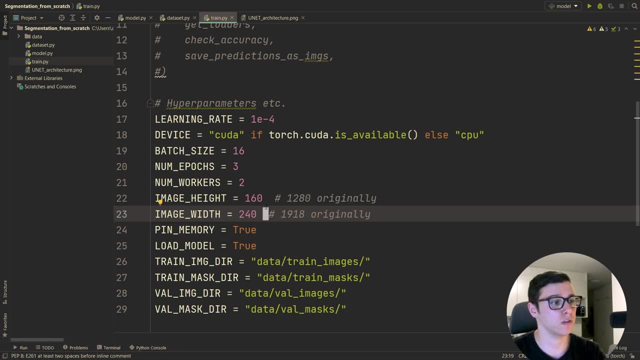 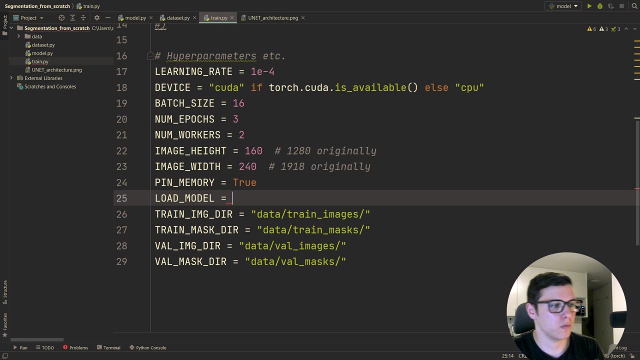 using you know, a very, very smart small part, but you would just change this, if that's. you know, if you were doing the competition and you wanted to obtain better score, and yeah. so pin memory: is true, we're gonna set load model, set it to false originally and then just specifying the paths. 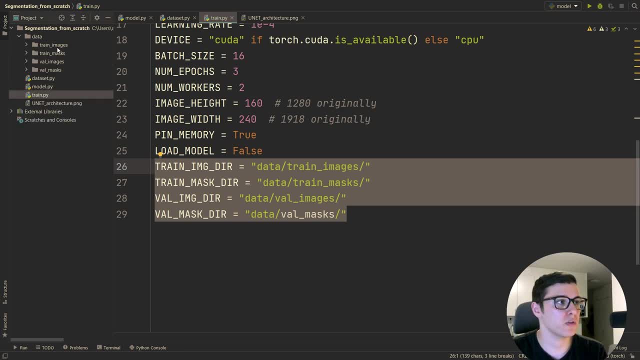 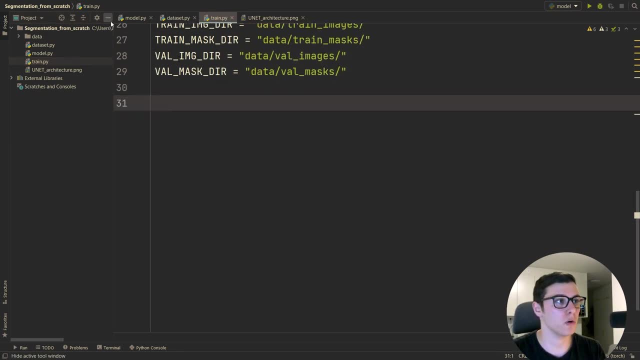 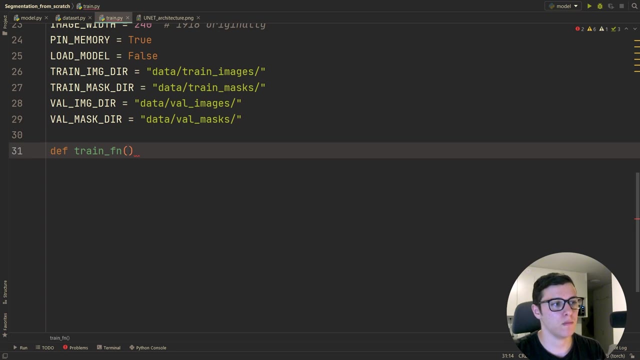 where we have the data set, that's, the training images and then validation images. all right, so I'll just show you the general structure that we're going to be creating. so the general structure will just have a training function where we will send in some loader, some model, some optimizer, loss function and also. 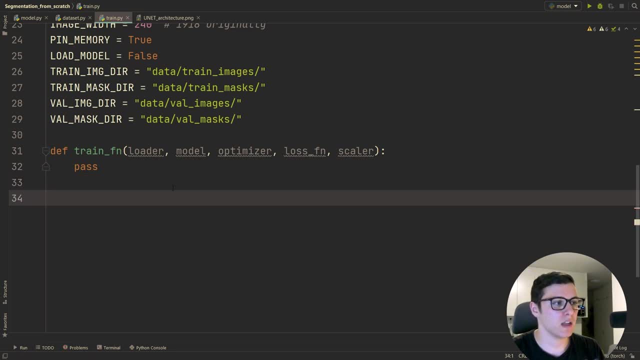 scalar. I will go through that, but so that's the train function. we'll have a main function and then we'll go through that, and then we'll go through that, and then we'll go through that and then we'll do check if name equals main and why. 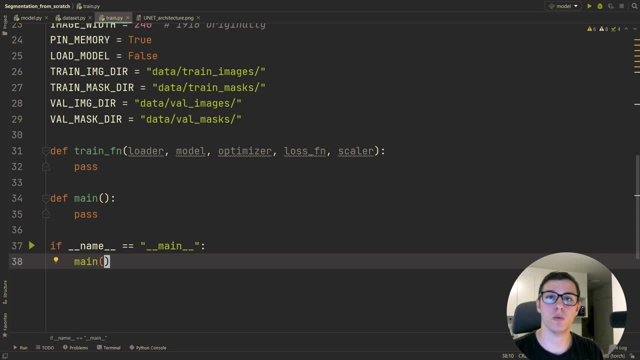 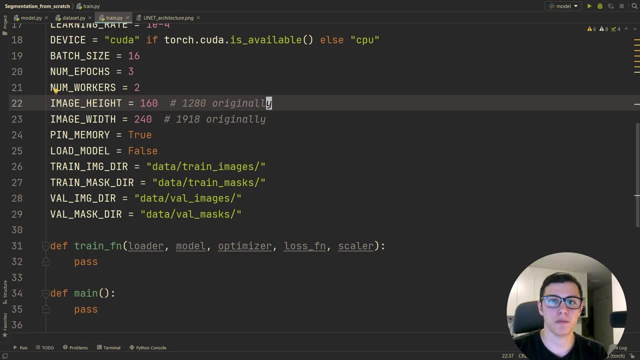 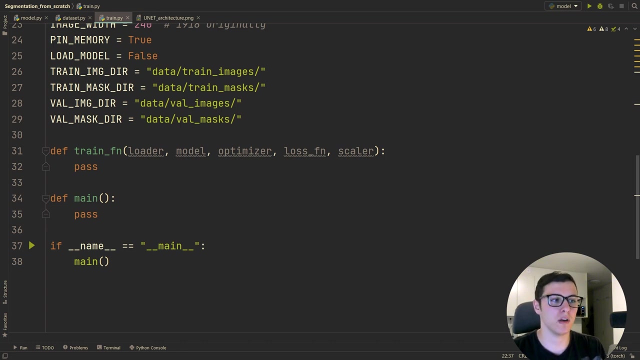 this is important right here is it's on Windows. you need to do this. we don't get any issues when you're running num workers, all right. so I mean we could perhaps start with the train function. so the trained function is going to do one epoch of training, and we'll use TQDM here for a progress. 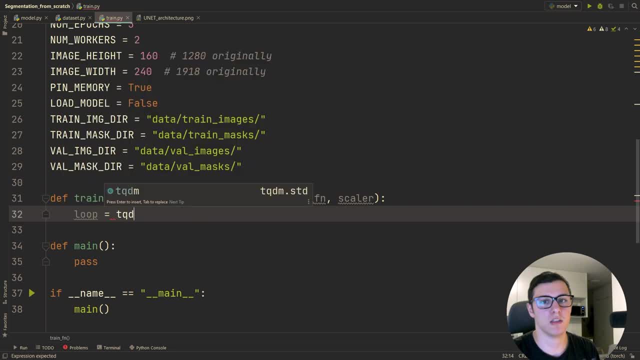 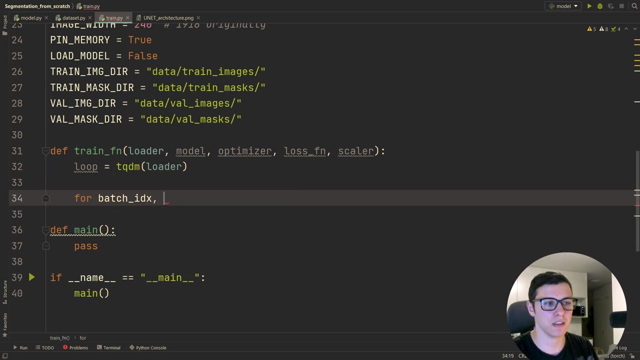 bar, so we'll just do a loop is TQDM of loader, and if you're not familiar with this, you don't. you don't have to do this, but I have a separate video on TQDM for a progress bar as well, so we'll just go through for batch index and then data. 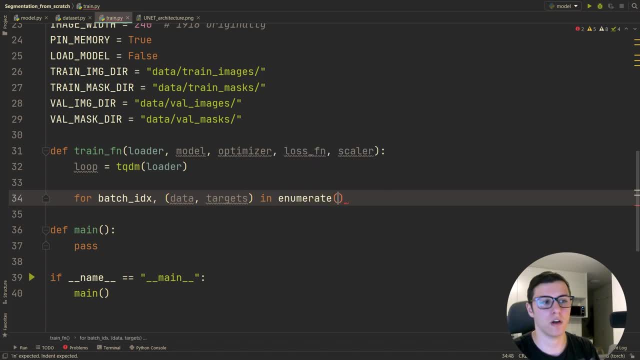 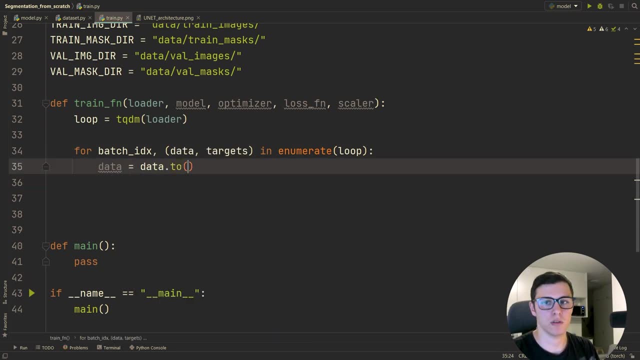 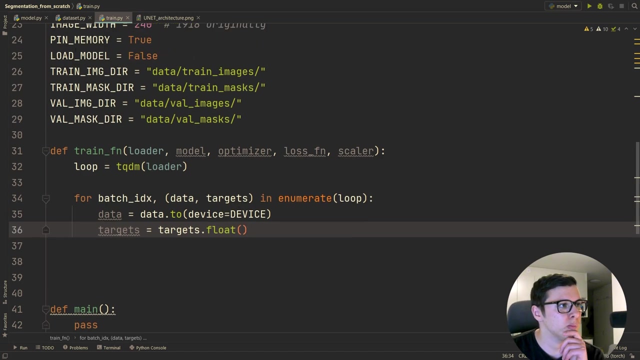 and targets in enumerate of that loop, and what we'll do is we'll just get it to CUDA. so data to a device equals device. same for the targets. also, one thing we need to do for the targets is converted to float. it should be float, right, mmm? yeah, it should. 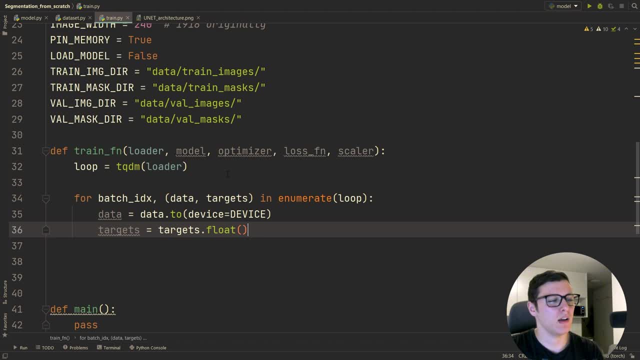 be float for some reason. it might not, I don't remember, but I think it's important for the. I think it's important for the binary cross entropy loss that we're going to be using. yeah, so I'm just converting into flow. think I got an error for that, or? 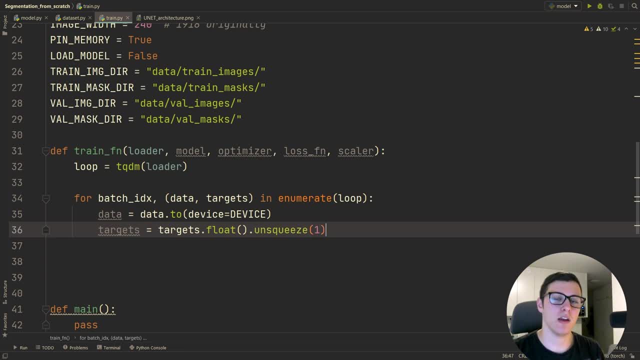 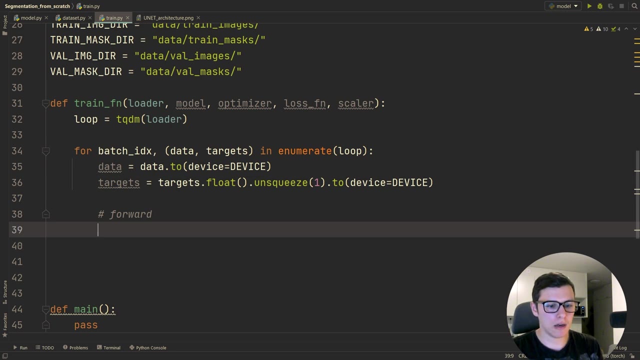 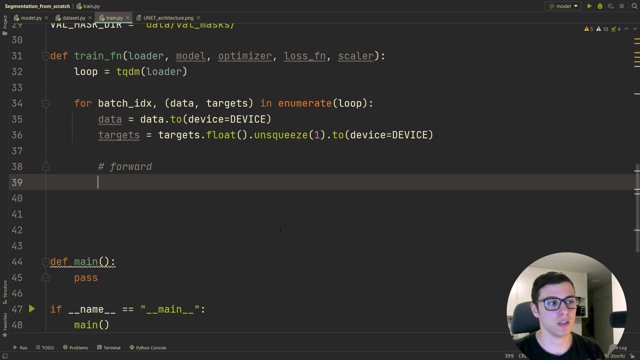 something. all right. we'll just do unsqueeze one and sort of adding a channel dimension, and then we'll do two-device equals device, all right. so for the forward, we'll use float 16, training, which I have a separate video on how to do, but so float 16. 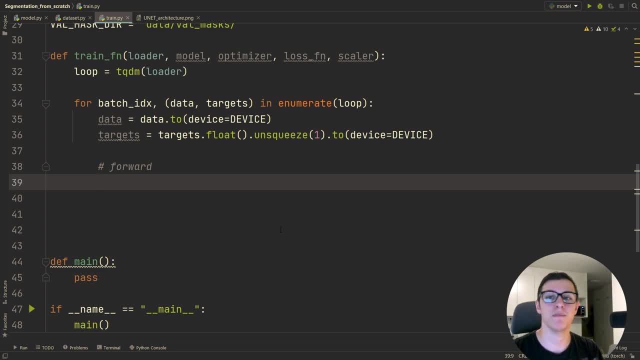 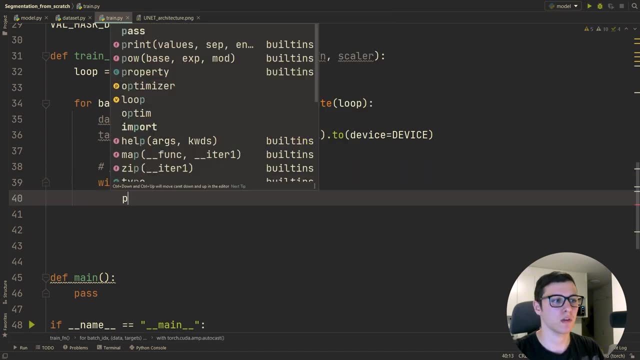 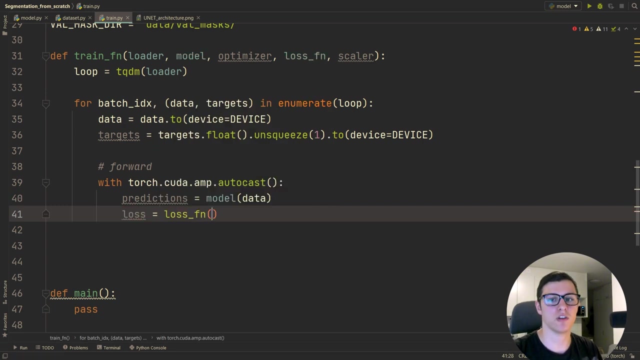 just sort of reducing our VRAM and speeding up training. so it's not too difficult to do either. we'll just do with towards CUDA amp autocast. we'll get the predictions by doing model of data. the loss will send in loss function and the predictions comma targets. 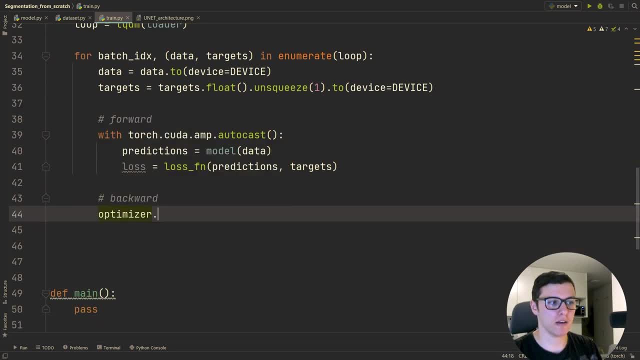 for the backward, I will first do zero, grad zero, all the gradients from previous. we'll do scalar dot scale of loss dot backward, and then scalar dot step of optimizer and then scalar dot update- all right. and then we'll do sort of we can update the TQDM loop showing the loss function so far. 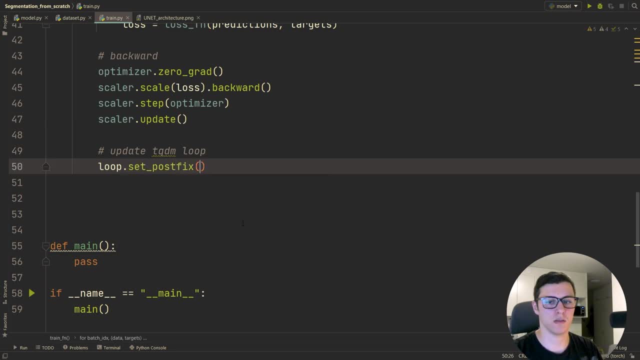 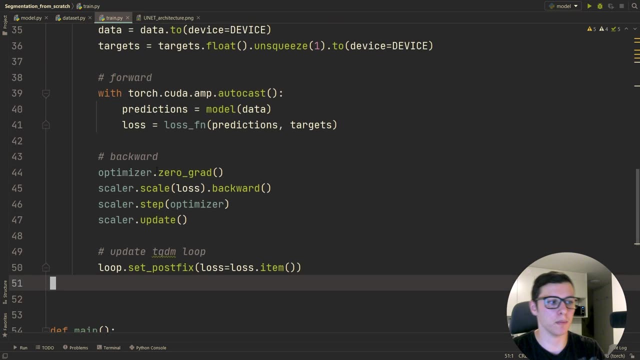 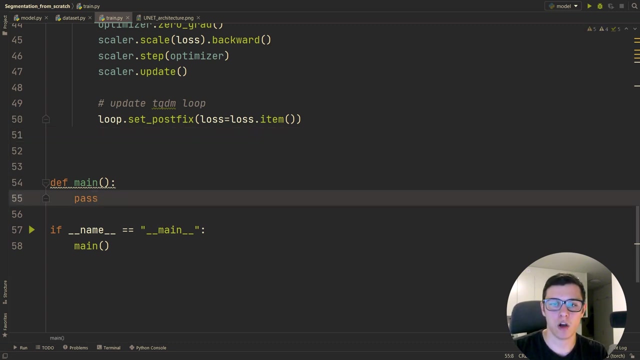 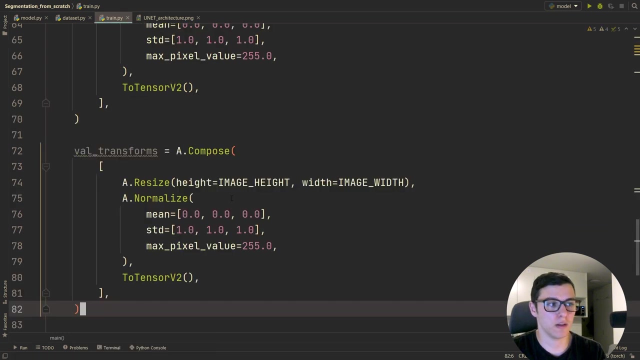 so we'll do loop dot set post fix loss equals loss dot item. all right, so that's for training, one epoch in our main function. I'm going to- let's see, I'll copy in those two, just because I've covered it in the albumitations library when I did that video. but so all I'm doing here is we're doing a resize. 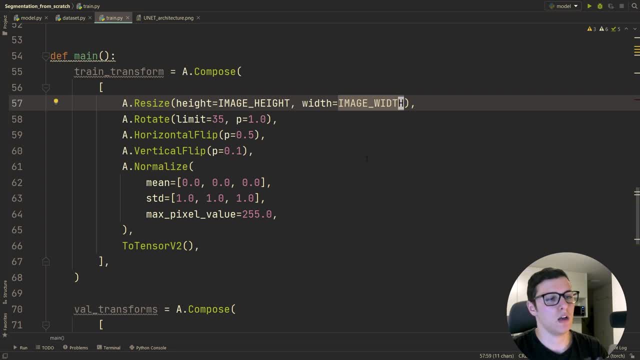 to the height of image height, image width, which we wrote at the top, and then we'll do a rotation: horizontal flip, vertical flip, normalize. here we're actually just dividing by 255, so we're getting a value between 0 and 1, and then to tensor and similar for the validation, although we'll just resize and normalize. 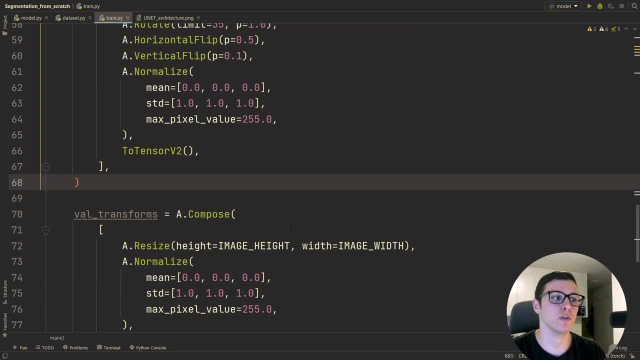 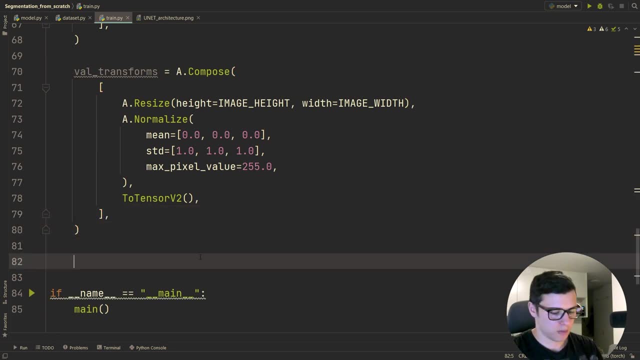 right. so that's all we're doing here. very similar to pytorch, nothing really difficult here. alright, so next we'll just create our model, which is going to come from unit and which we created so in channels. it's going to to be three, our channel is going to be one, And we'll get that to device The loss function. 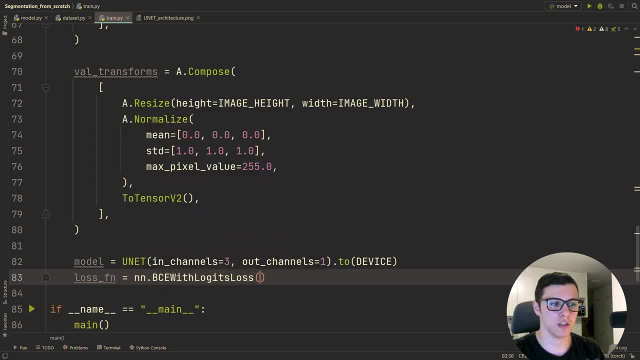 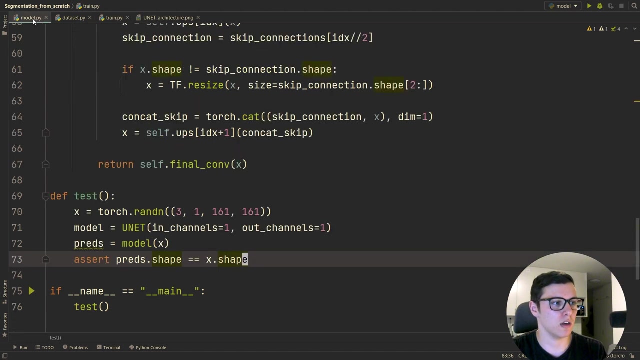 is going to be a BC with logit loss And so so binary cross entropy. And why are we using with logits is because we're not so on our output we're not doing sigmoid. You could remove this with logit loss If you did right here, if you did torch dot sigmoid on the model or the output. 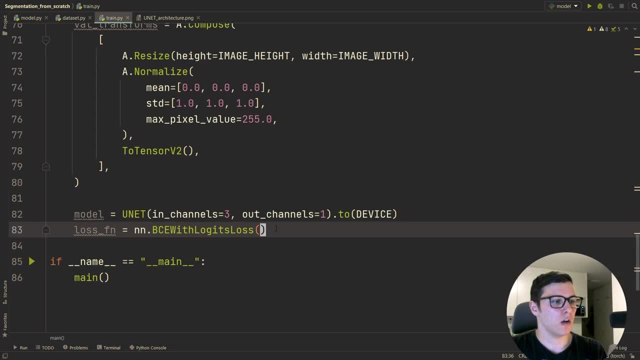 of the model. All right, and then? so what would you do if you were extending this, if you wanted multi class segmentation? all you would do you would change the out channels. let's say you had three different colors, three different classes. you would change this to three. 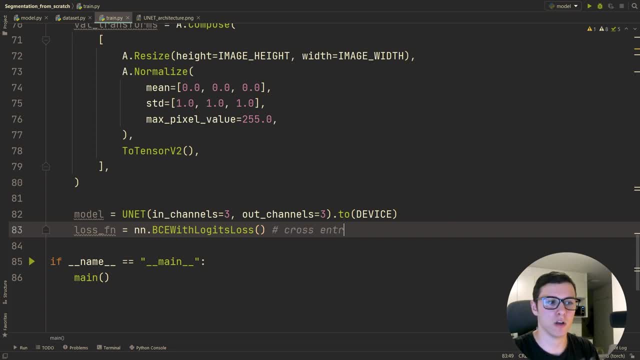 you would change the loss function to a cross entropy loss And that's all Right. So you know, this is very easily extendable to multiple classes. Let's just do that for now, And then we'll do our optimizer. So our optimizer. 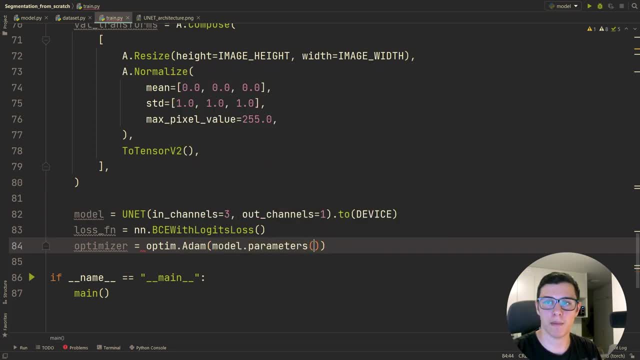 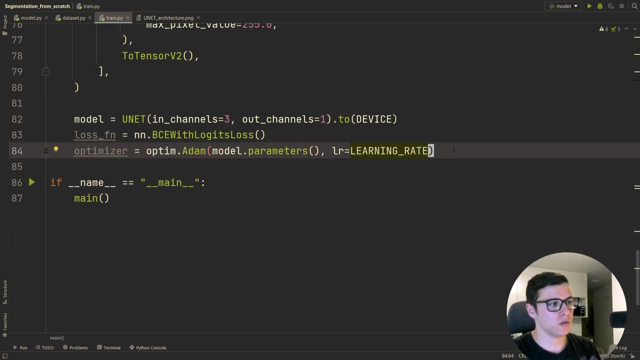 I'm just going to use Adam with mandat parameters. learning rate equals learning rate. All right, so to get our loaders. obviously we could do. you know, Carvana, data Set and then data loader. of that I think it looked a little bit ugly, took a little bit too. 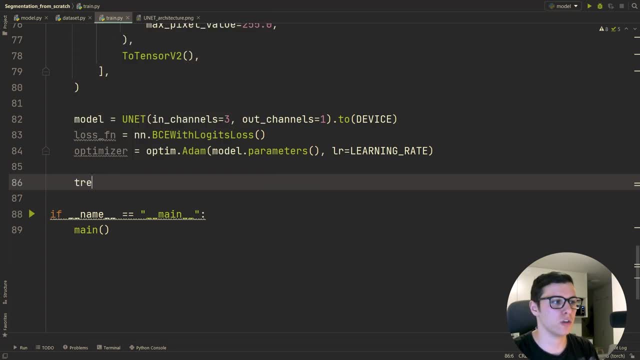 much space on this main function. So we're just going to do train loader, comma val loader And we'll run get loaders And I guess here we're going to send in the train image directory, train mass directory, validation And the batch size, the transforms that we're going to perform. 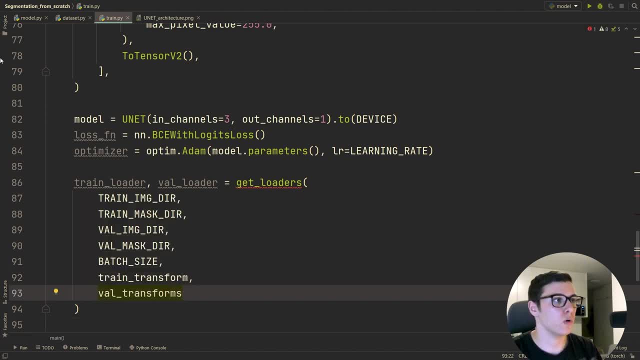 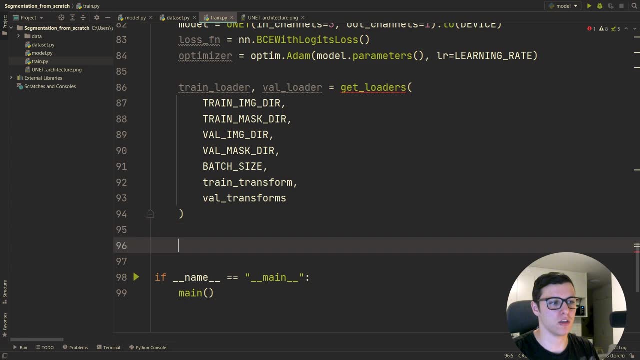 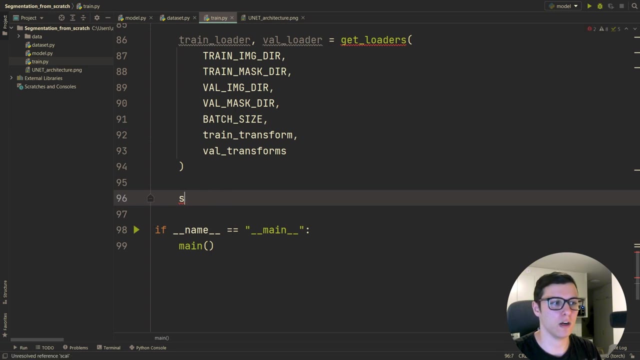 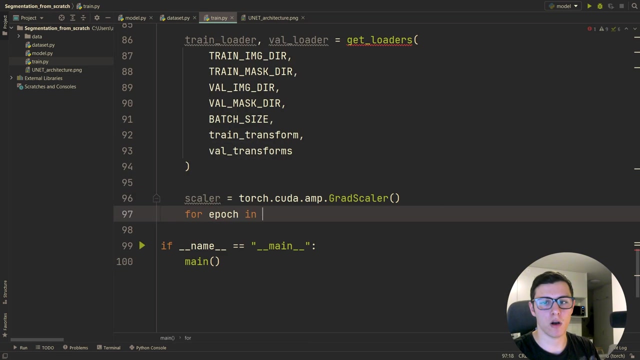 and then the val transforms. So we'll go to that, create that utils file and do that. But I guess we could finish this as well, So we're going to create that pretty soon. First we want to do scaler is torch dot, CUDA, dot, amp, dot. grad scaler. We'll go through for epoch in range of num epochs. 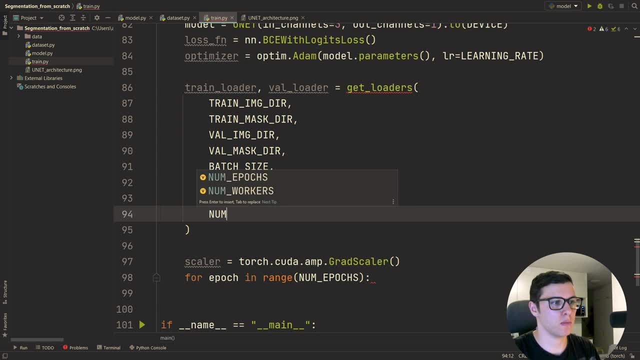 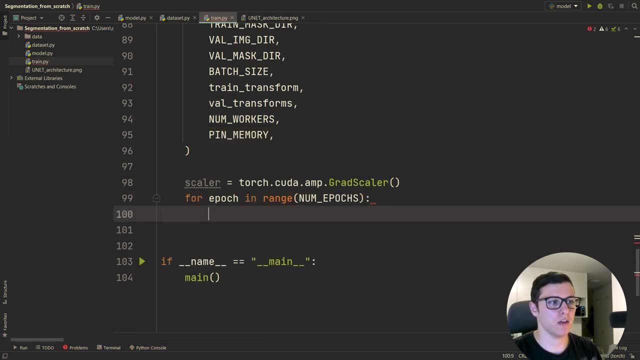 I guess also we need to send in here, we're going to send in num workers and also pin memory. Alright, so for epoch in range of num epochs, we're going to call our train function, which will just send in the train loader, the model, the optimizer, the loss function and the scaler right, Nothing. 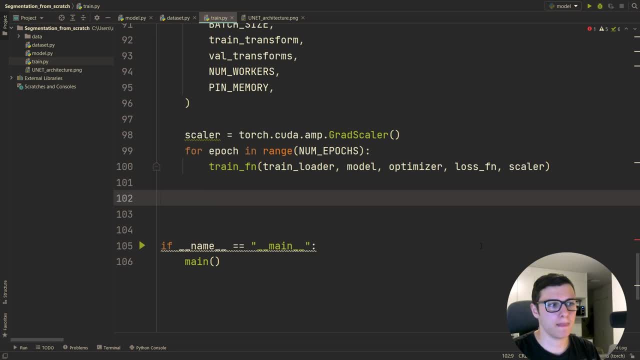 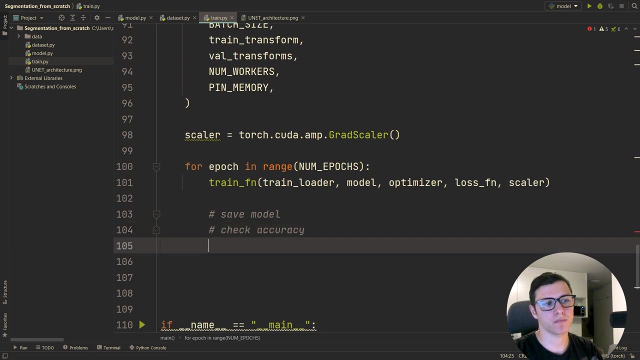 too difficult here And let's see what we need to do. So I guess one thing, What we'll do later on is we'll do save model, we'll do check accuracy And then we'll do print some examples to two folder and then we'll just see that it. 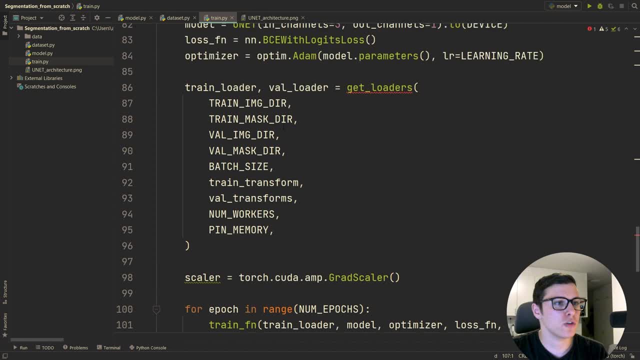 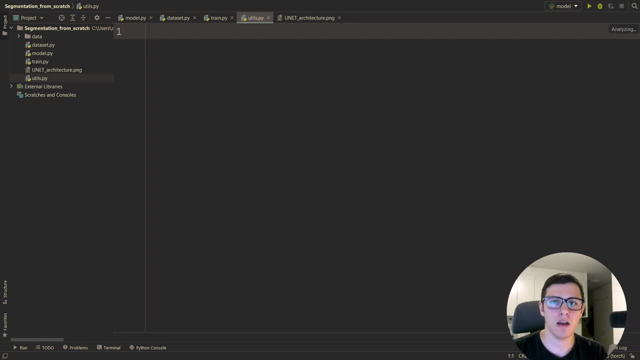 actually looks good. But So first let's create this utils files now, so utils, And I'll just copy paste in the import. so the import: torch vision, torch Carvana, data set right, and then the data loader. I'll paste in two files right here, which. 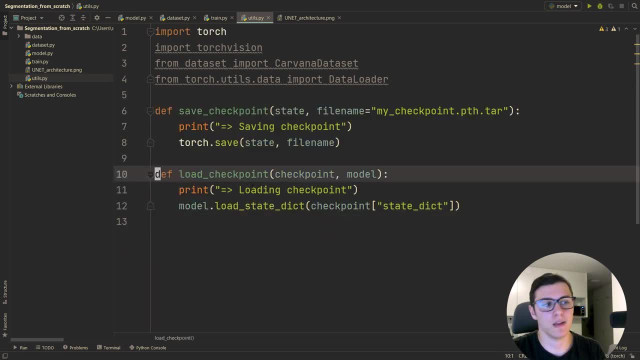 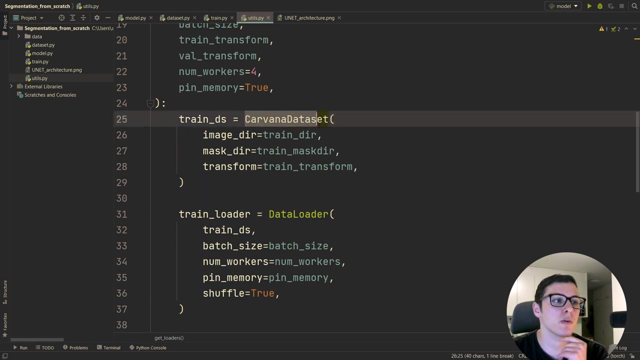 is two functions rather, which is save checkpoint and load checkpoint again, I also have separate videos on that, if you want to check that out, and I'll also copy paste in the get loaders and I'll go through it. so the reason for this is: I think this is honestly pretty simple. all we're doing here is we're creating. 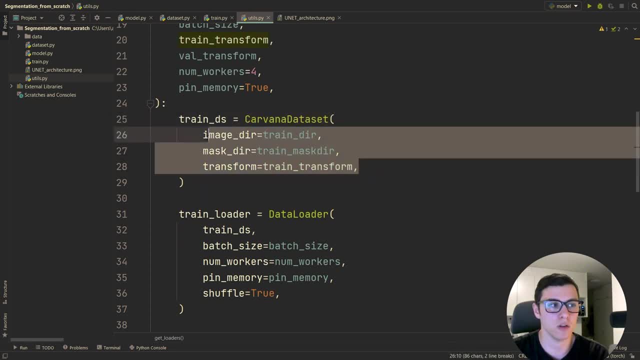 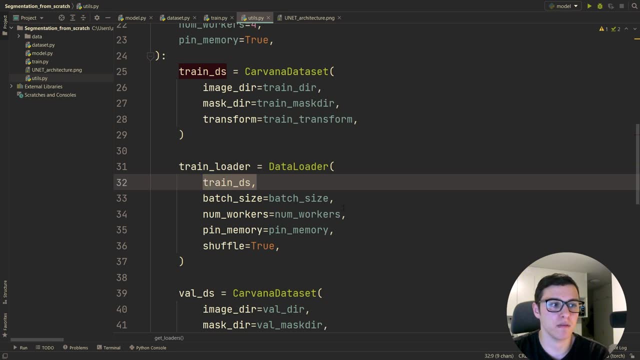 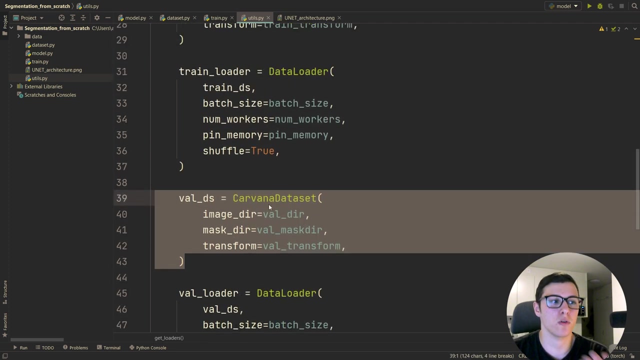 the coronavirus. we're specifying the transforms and all of that, the image directory, mass directory. for the train loader, I were specifying the training data, set, batch size, nom, workers, pin, memory and then shuffle similar thing for the validation. so the difficult part here was actually called cream loader and then making it really hard to actually compute a full. 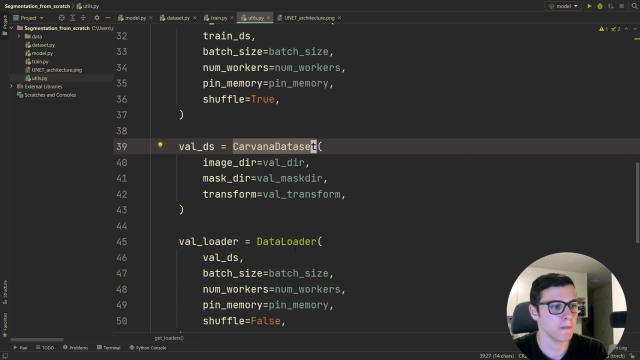 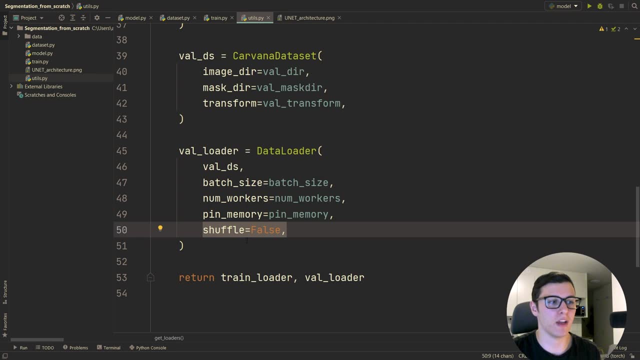 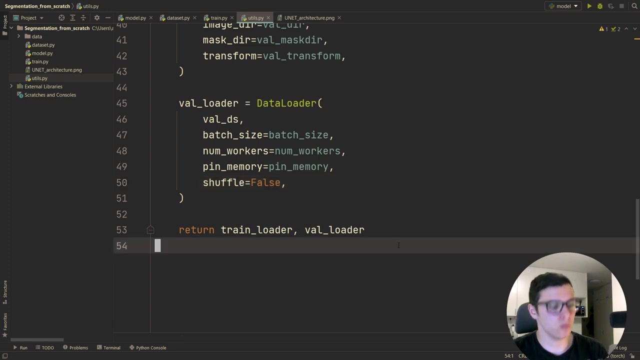 creating that Carvana data set, which we did before, And all we got to do is just create similar for the validation loader And we won't shuffle that one And then just return train and loader. I guess we could do the check accuracy. 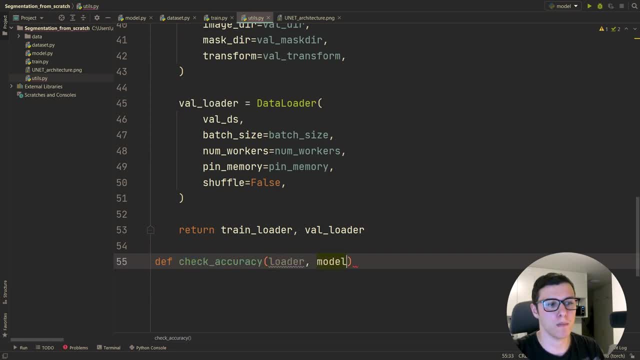 That might be a little bit more difficult. So we'll send in some loader, some model, some device, default CUDA And we'll check first. so the number of correct is going to be 0, number of pixels we'll set to 0.. 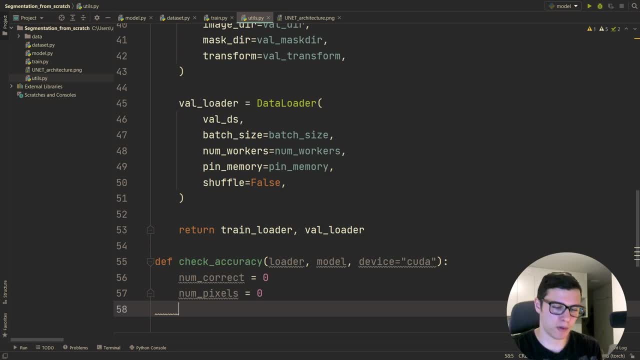 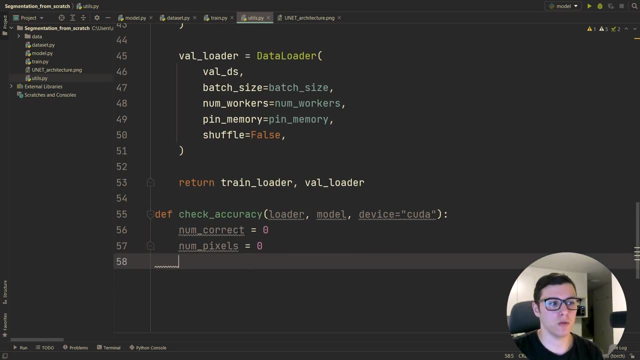 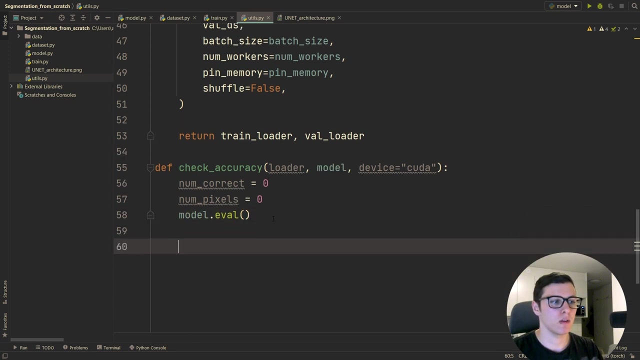 So remember, for segmentation, we're outputting a prediction for each individual pixel, the class for each individual pixel. So what we'll do is we'll just, or we'll get to that, And then we'll also do modeleval. We'll wrap everything with a torch, no grad. 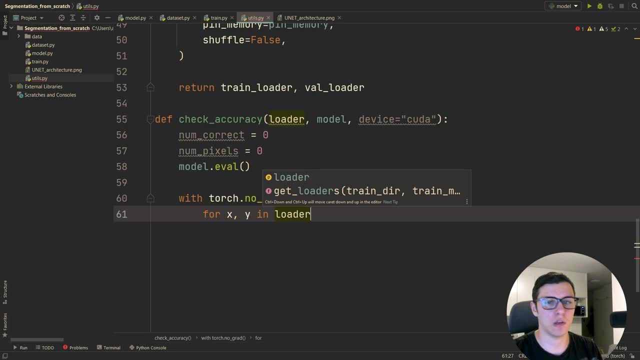 And then we'll go through that loader. So for x and y in loader we'll do xtoDevice, YtoDevice, We'll run through the models so we'll get some predictions. which is torch sigmoid of model of x. 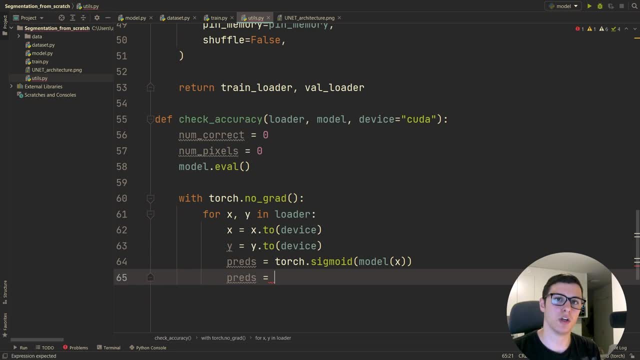 Then what we'll do is we'll convert all those that are higher than 0.5 to 1.. All those less than that, we'll convert to 0. 0.5. 0.5. 0.5.. 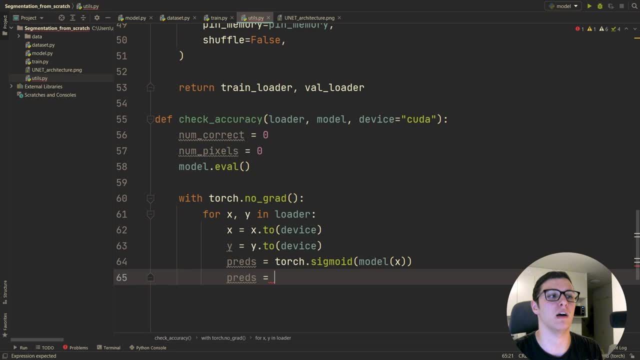 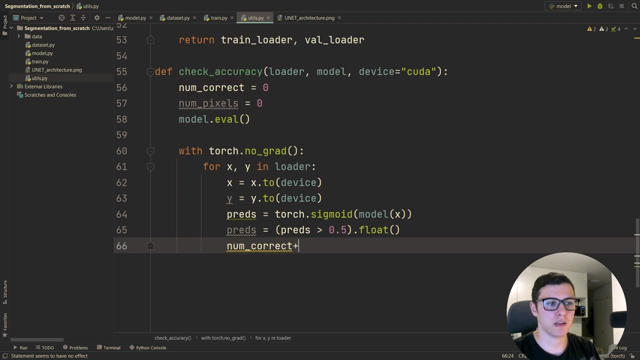 0.5.. you would need to adapt this check accuracy to to if you would have more classes, but I don't think that would be too difficult perhaps. but just know that this is for binary. so we'll do predictions. is predictions greater than 0.5 and then dot float right, we'll do number of correct is plus equals the. 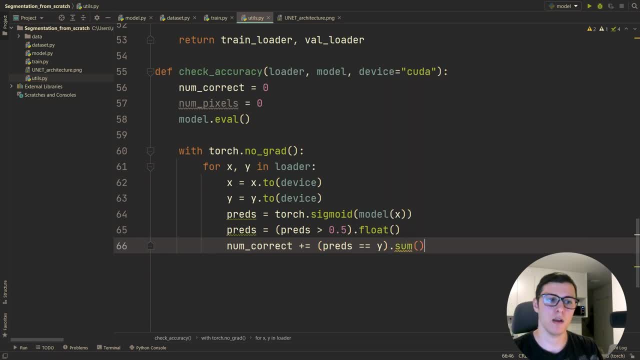 predictions that are equal to Y and then sum, so that will sum all, sum all of the pixels. then the number of pixels that was in that image is going to plus equals torch dot. number of element, numeral of predictions. and yeah, so then we'll just print: you know, an F string got number correct, divided by number of. 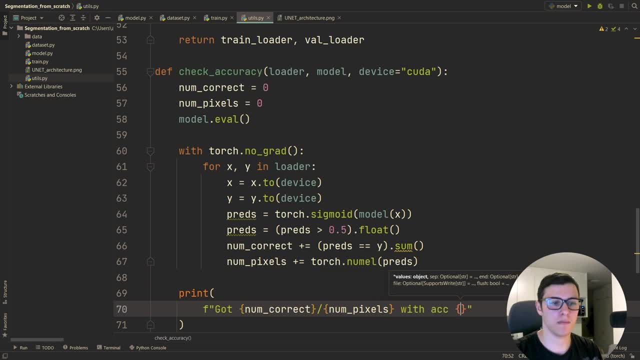 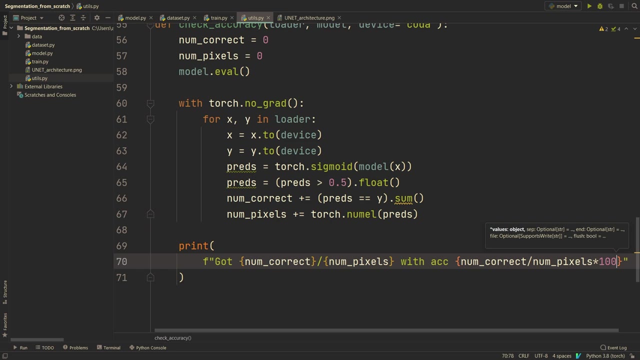 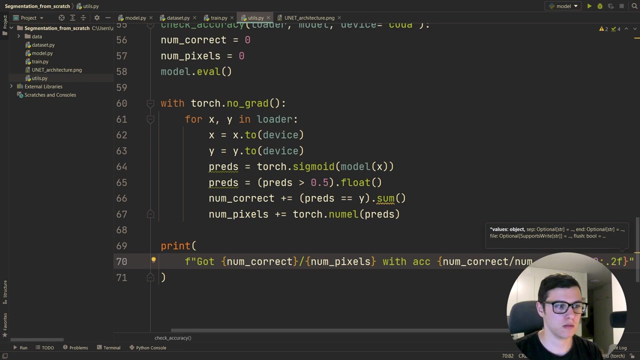 elements and then we'll just print. you know, an F string got number correct divided by number of pixels with accuracy, and then let's just do num correct divided by num pixels and we'll multiply that with 100 and then with two floating decimals. yeah, so that's it for the accuracy, one thing I actually want to. 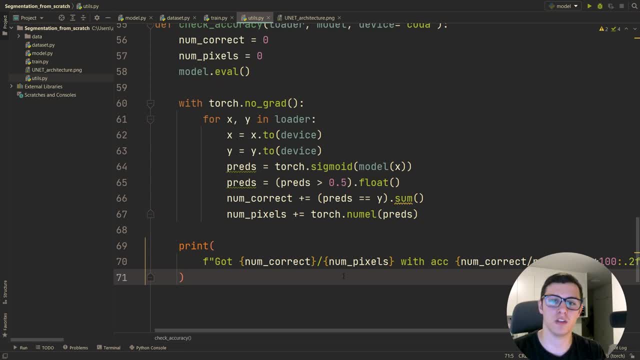 edit in a bar. so what we wanted to note is something that students can believe in, things we're going to look at, a normal interpolation that you can do on face. so what we want to do is the same thing that we want to do here as well, which, if 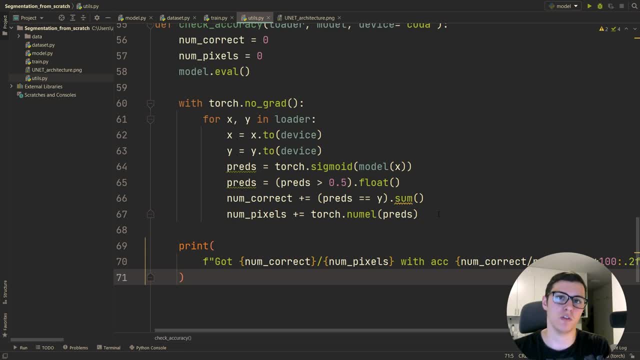 you don't follow this, it doesn't matter too much. but one thing that's kind of flawed when doing the accuracy is that if we just output sort of just black pixels- is we just output sort of just black pixels- will have an accuracy of greater than 80%. so they found that there are better metrics for measuring this, similar to object detection, using intersection over union and so on. it's a better metric. they also found thatえる experiences as well out to the object detection, we do have a number of interchange criteria and things that also need to be. did you knowfilmon học, if you want? 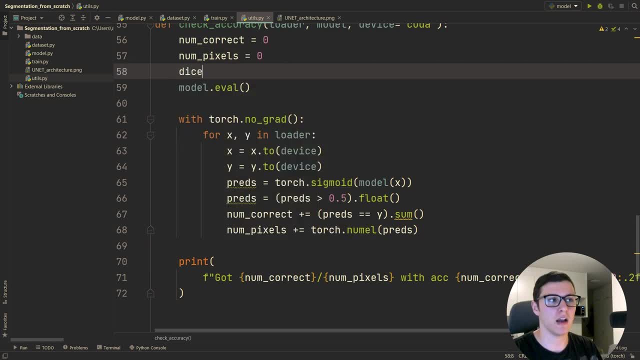 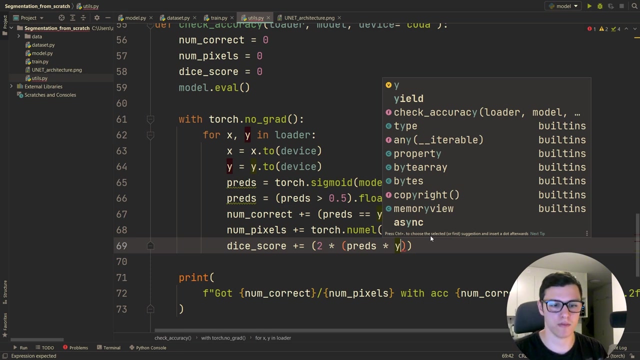 found that there's a better metric for this, which is using a dice score, And this is just one line, So I'm just going to add it. But what it is is it's going to be two times sort of the the pixels. where they were, there were the boat outputting a sort of a white pixel. 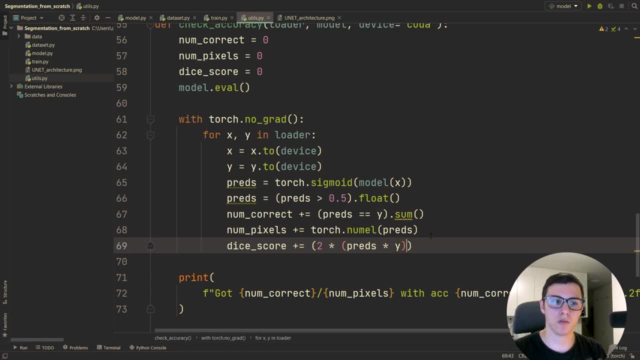 So we're going to just, element wise, multiply them. So where they are the same, they're going to be up with one. we're going to sum those two, So we're we're summing the number of pixels where they are both the same or both outputting a white pixel. then we'll divide that by prediction, by: 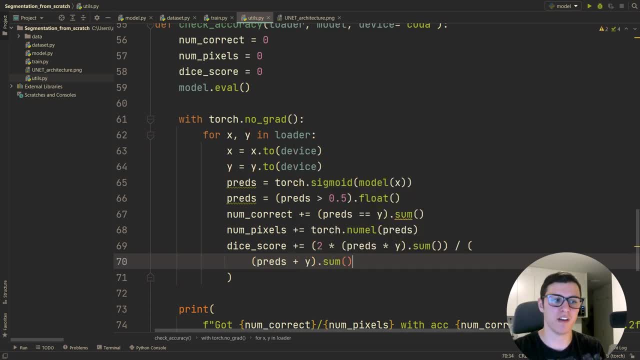 predictions plus y dot sum. So we're dividing by the number of pixels that they're outputting, one for both of them, And then we're going to divide that by the number of pixels that they're outputting for both of them, And we'll just add a epsilon of one e minus eight. Yeah, so yeah, actually I don't. 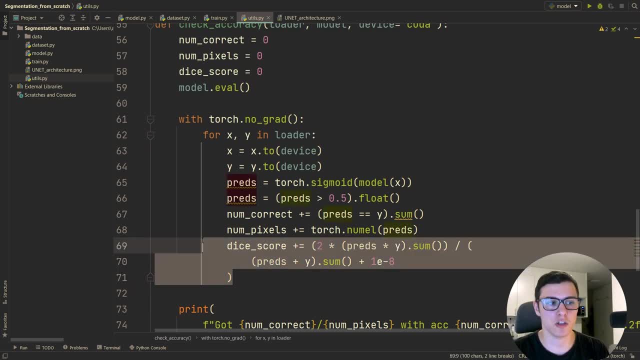 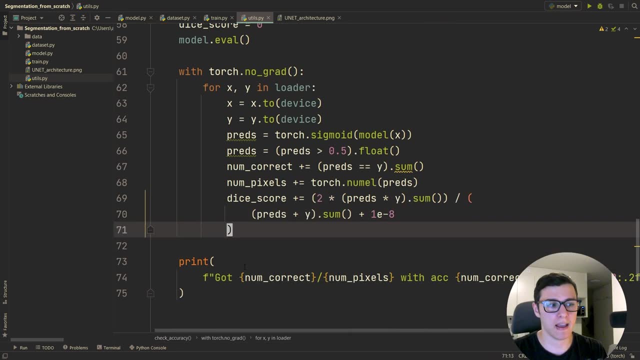 know too much about die score. This. this is just for binary, So it's pretty simple here. You can probably Google and find out how you do it for multi classes, And so we'll just use this for now, just knowing that it's a little bit of a better measurement to evaluate how good it is. But if 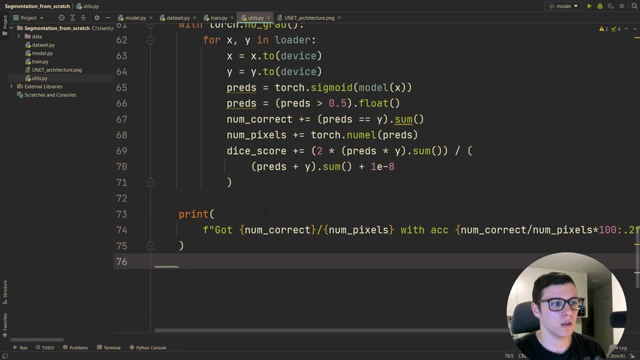 you don't follow it, you're not going to be able to do it, So we're just going to do it. And then all of this- don't don't bother too much about that, All right, and then we'll just print die score. 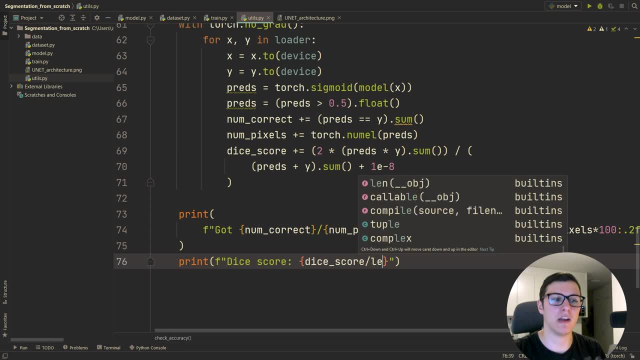 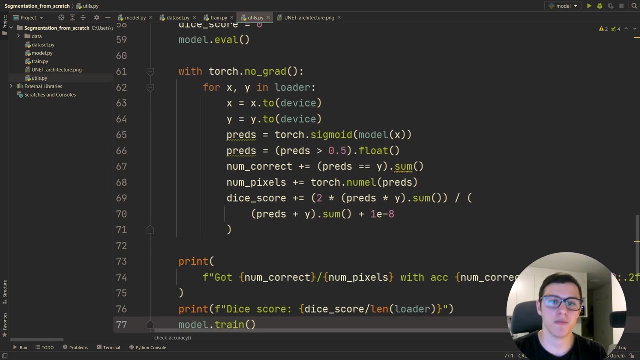 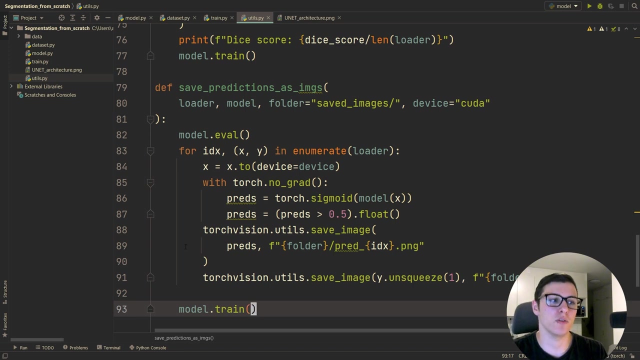 We'll do die score And then divide that by the length of the loader, All right. and then we'll set model dot train again All right. so that's the check accuracy for the same predictions as images that I also imported. I'll copy paste that in, And so what we're doing here is we're just going through and then outputting. 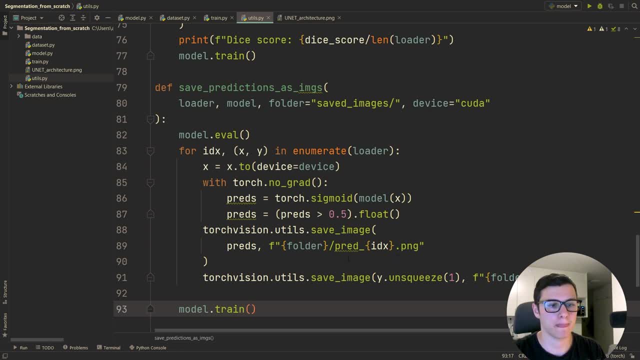 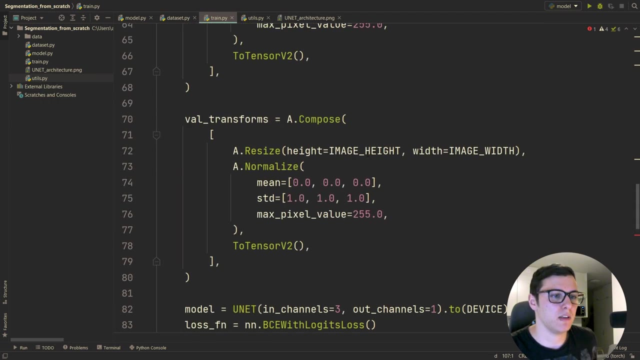 the prediction and the corresponding sort of correct one associated with that. with that one, It doesn't matter too much here. This is just so that we can get a visualization of what it's doing. All right, that was probably too fast, But yeah, what we'll do now is we'll just remove from utils. we'll 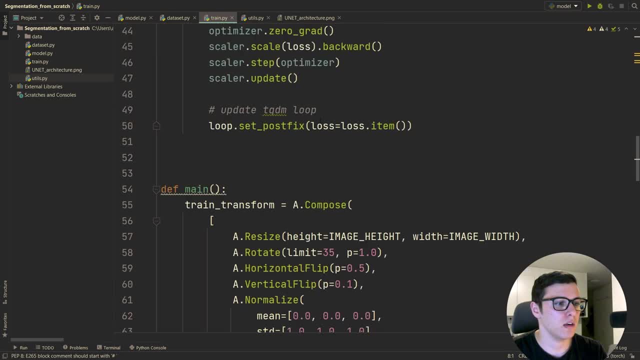 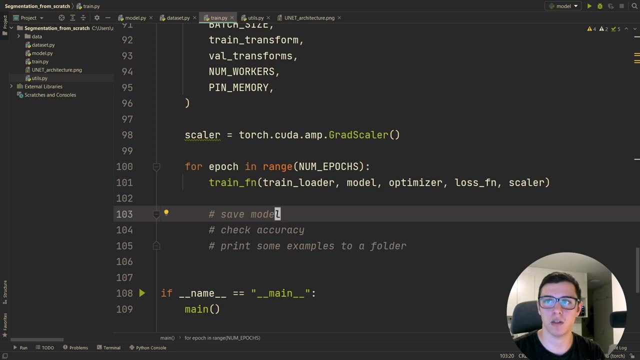 just import all of that stuff And yeah, so now we can in our right here, we can save the model And we can do all of those things that we wanted to do. So for saving the model, we'll create a checkpoint, We'll just do state. 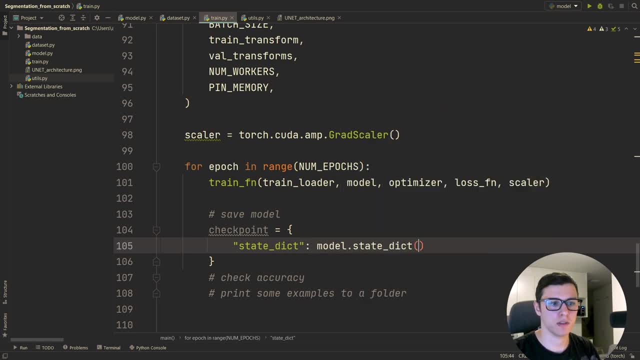 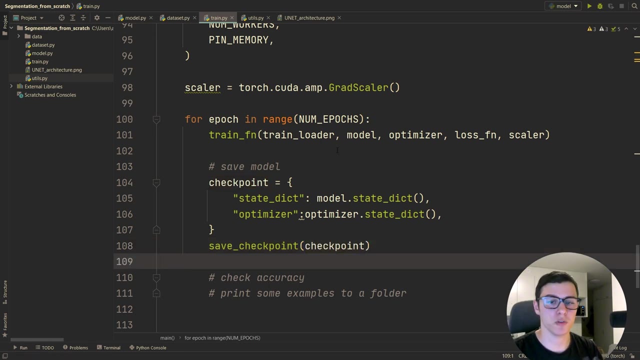 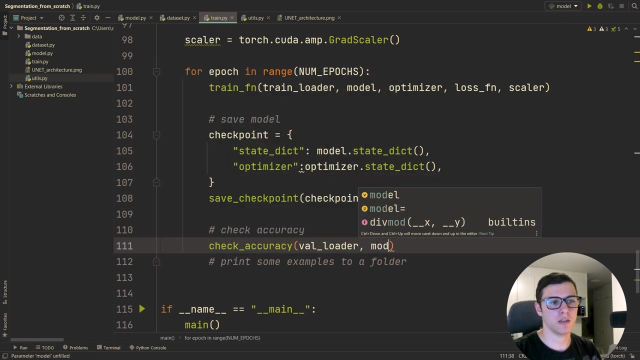 dictionary, model state dictionary. We'll also store optimizer- optimizer state dictionary. then save point of checkpoint from the utils file and then check accuracy. We'll just do check accuracy of validation loader, send in the model, send in the device And then we'll print some examples to a. 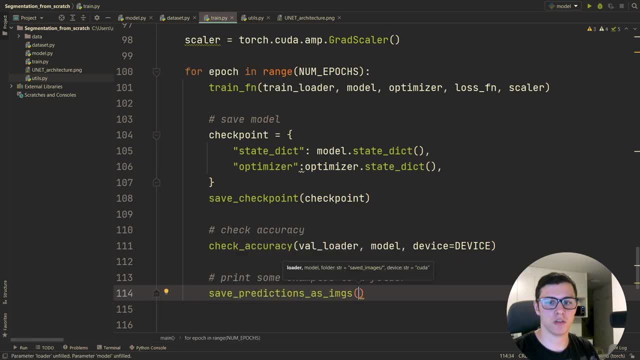 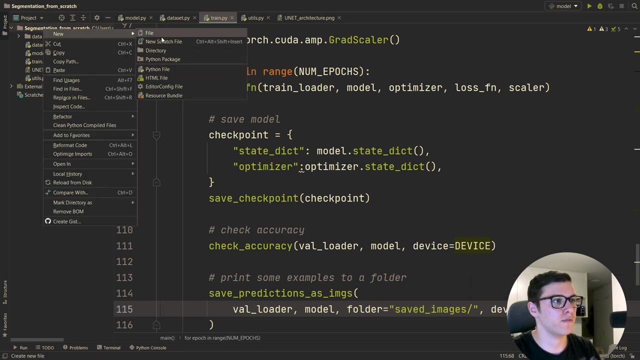 folder. So let's do save predictions as images. we'll send in the val loader model, the folder we'll do saved images, And then the device is just a device. So what we'll do here is we'll just create a folder right there, directory called. 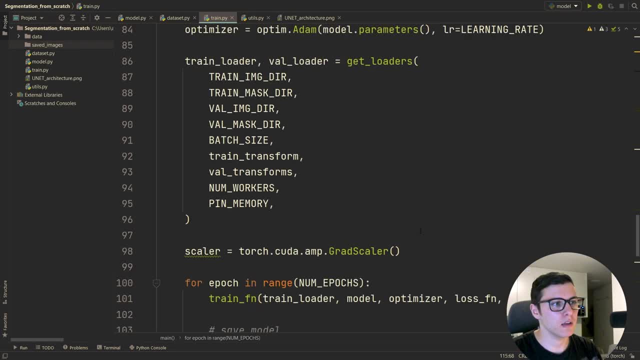 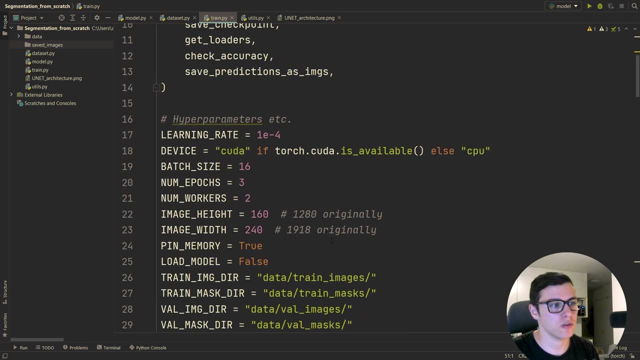 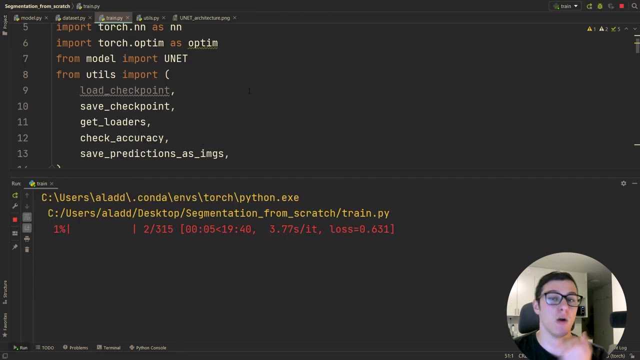 saved images And, yeah, that should be it for this one, And probably going to be some errors, But you know that's how. that's how it is, So let's try and run this now. Wow, it actually worked on the. 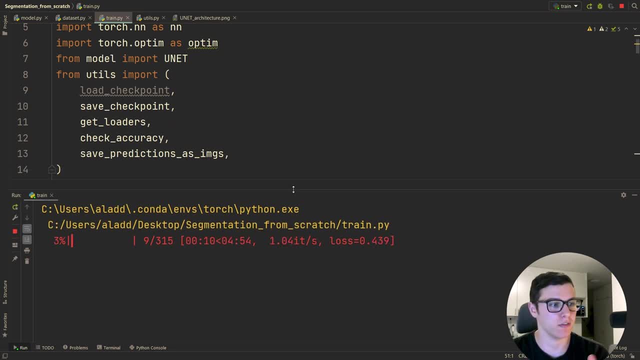 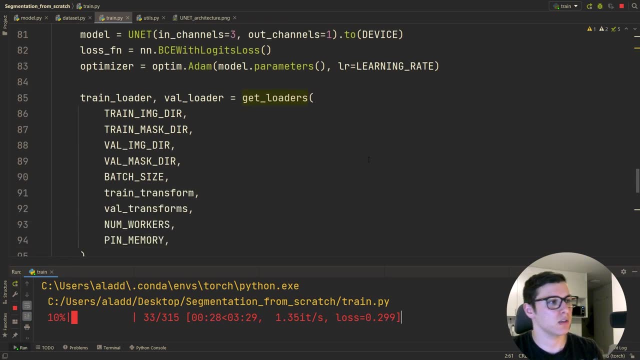 first try. I mean, I haven't made a single mistake this entire time. this entire video. that's insane. Uh, it's increasing super fast. Let's do a side check. Yeah, So we're not using the load checkpoint. Um, I guess what we can do in the meanwhile is also: let's see right here. 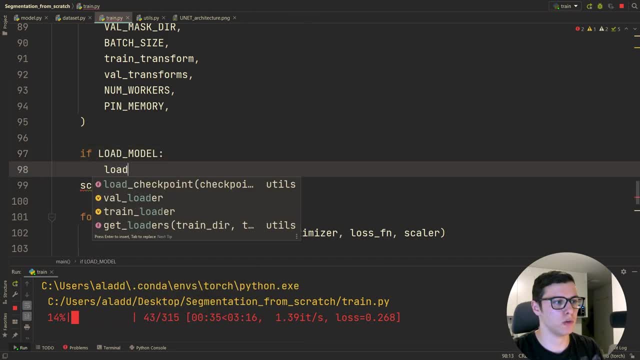 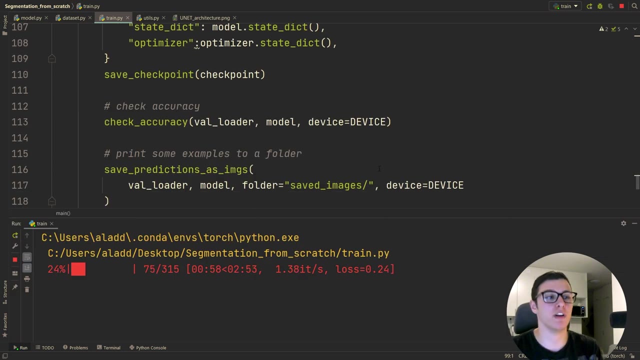 maybe we'll do, if load model will do load checkpoint of torchload, of my checkpoint. That's just what I call the file, my checkpointpthtar, And then I'll- Yeah, I'll just let it run And we'll see how good it is at the end of training. Alright, so I also 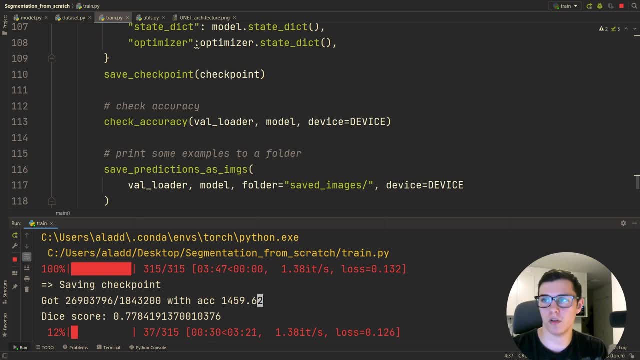 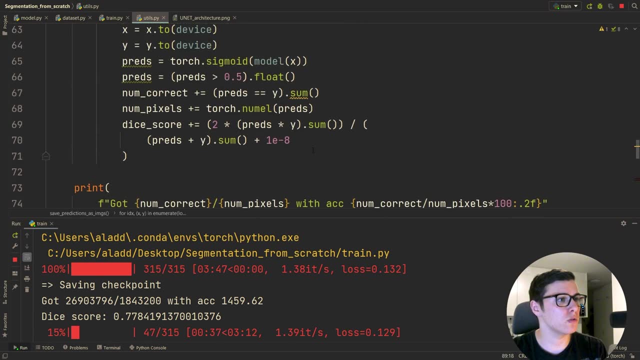 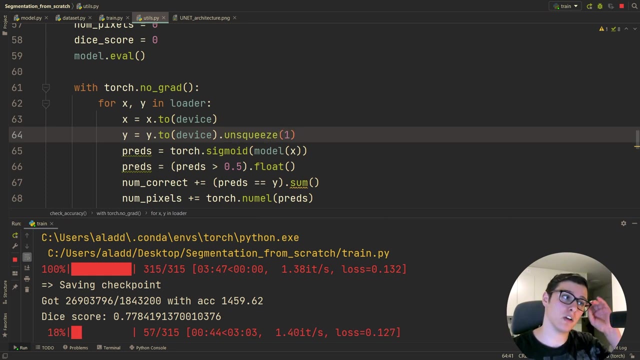 noticed now, after one epoch, the accuracy stuff is actually wrong, And I wonder what we did wrong there Exactly. I think we missed to do one thing, which is that we got that unsqueeze one right there, And the reason why we have to do that is because 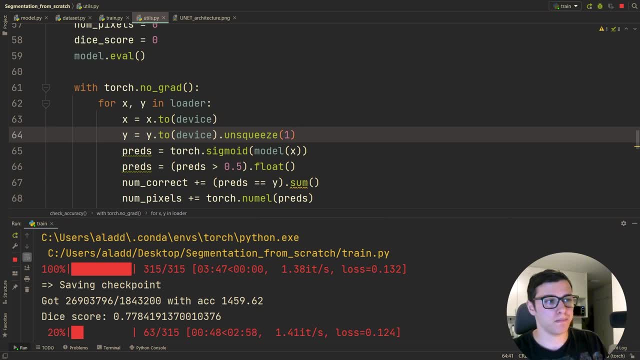 the label doesn't have a channel Because it's grayscale, So we just have to do that- unsqueeze, and then the accuracy should work. So now we're just outputting rubbish, but the die score should be okay. So what we'll do is we'll just let this. 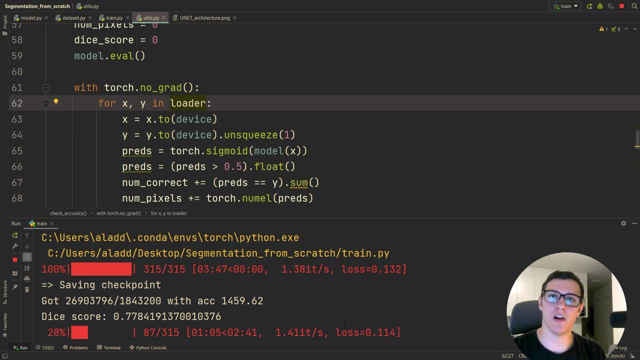 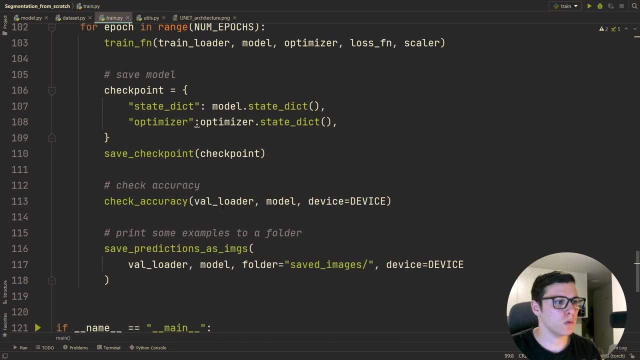 train until it's done And then we can rerun it and evaluate and see what we get for the accuracy and the die score. Alright, so now that it's trained three epochs, what we'll do is we'll just copy this: check accuracy. I will put it just after we load. 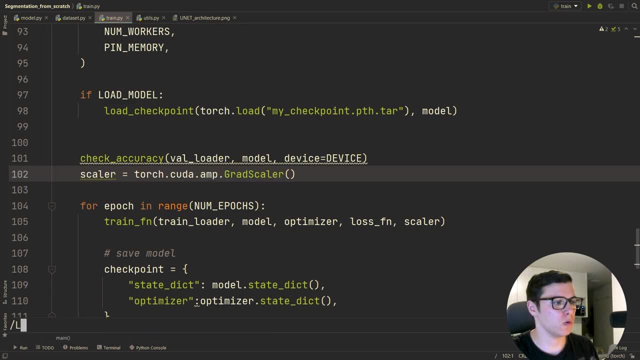 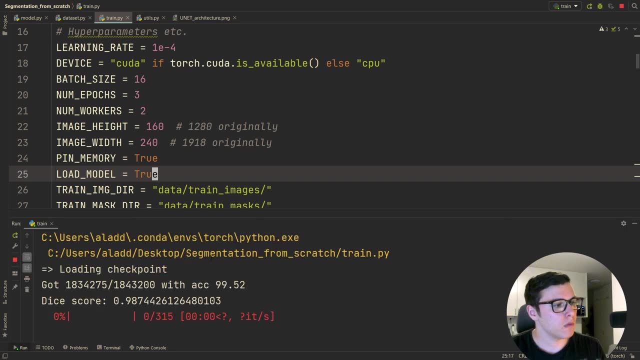 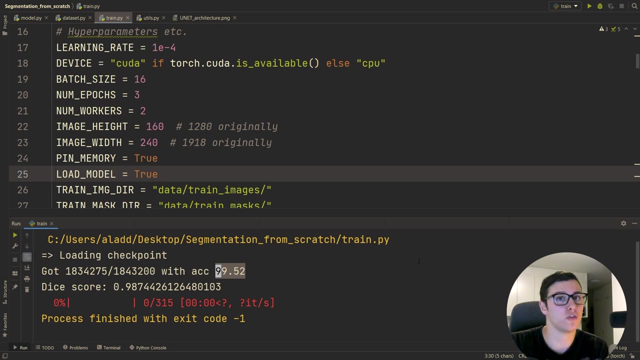 the model And then I guess we'll go to load model and we'll just change that to true and rerun it and see what we get Alright. so we see that we get an accuracy of 99.52.. And we've just trained three epochs. 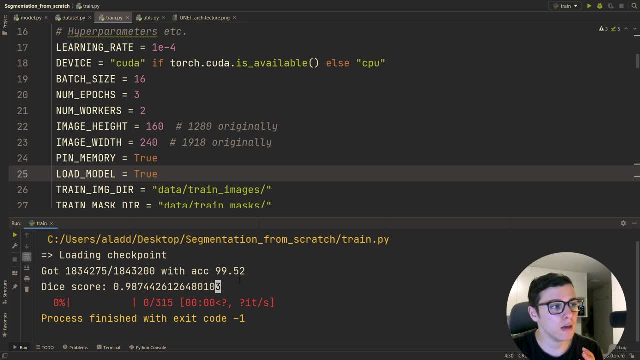 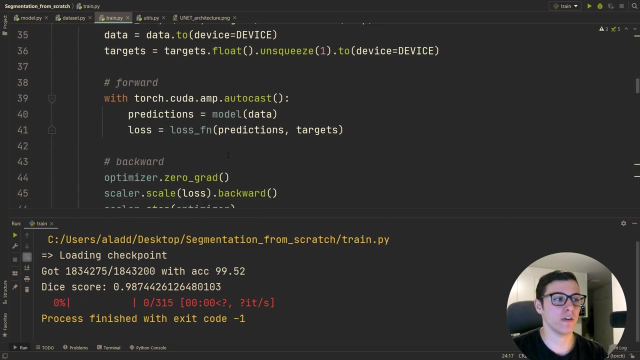 we get a die score of 98.7.. And you can just train this for longer and it would definitely improve. Then you would change the image height, image width, make it larger, And that would allow for the data augmentation of the shot images. And that's probably what I would do. And then maybe 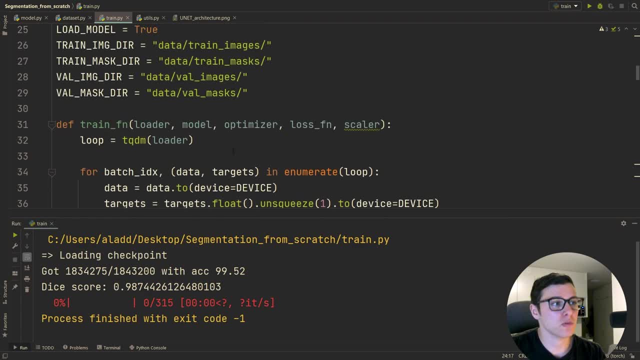 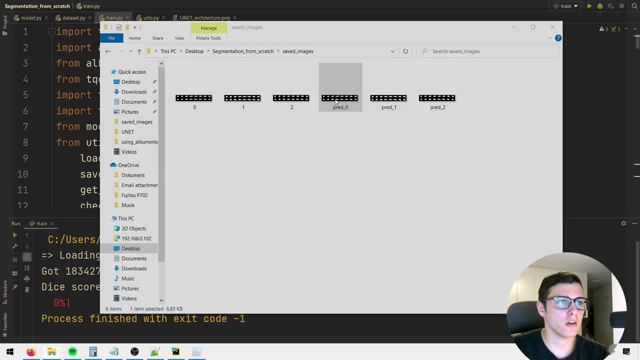 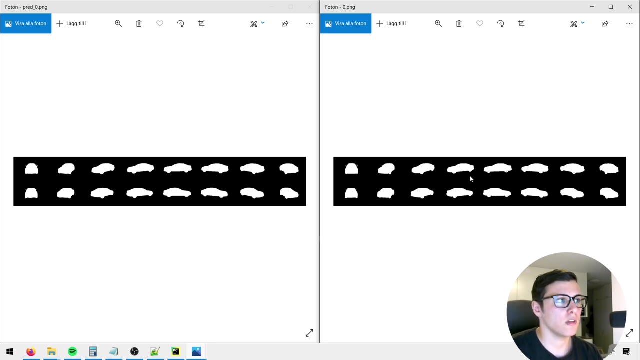 perhaps consider adding more data augmentation. But yeah, so I mean, this is for sure working. Let's see if we can look at. so save the images. So here are some predictions. Let's put them side to side, Alright. so here it is. So at the right we have. 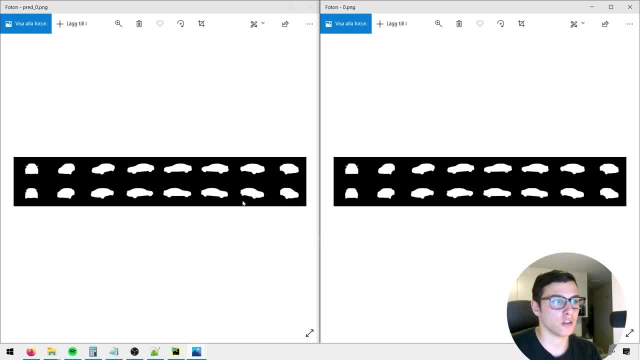 the correct target segmentations. On the left we have the predictions, four de corresponding targets. as you can see, it's obviously very close to being correct, which is why it also has that good of a score. i think that what the winners had of that kaggle competition, 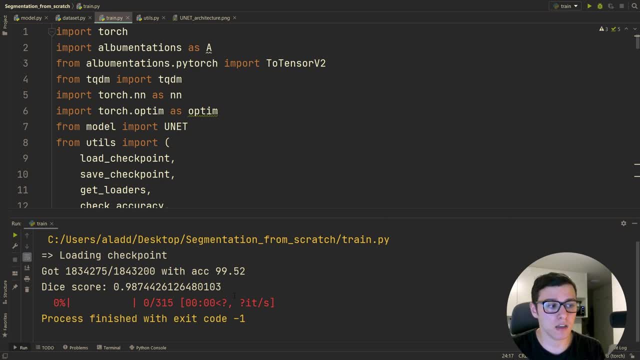 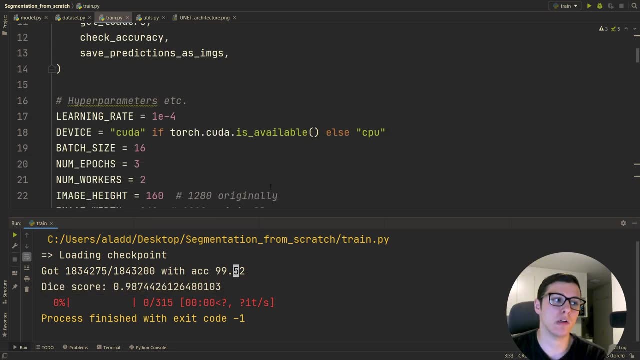 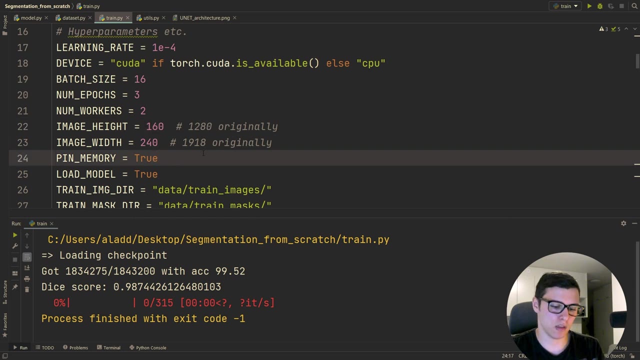 was 99.7 in dice score, so obviously we're pretty far off, but yeah, and also we're looking at smaller images. um, what you would do, what you would do, is you would want it for these original images and then you would just do a resizing, um, and yeah, so that would, and i guess the resizing has to be.